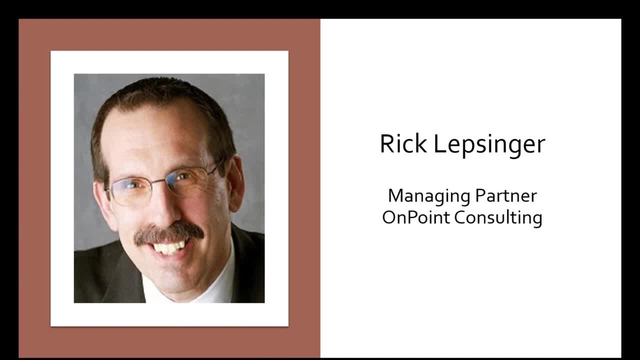 Rick has written numerous articles and is the author or co-author of several books, including his most recent Closing the Execution Gap- How Great Leaders and Their Companies Get Results. Welcome, Rick, and thank you for joining us today. Sarah, thanks very much. I'm glad to be here and everyone welcome. Thank you for joining us today. 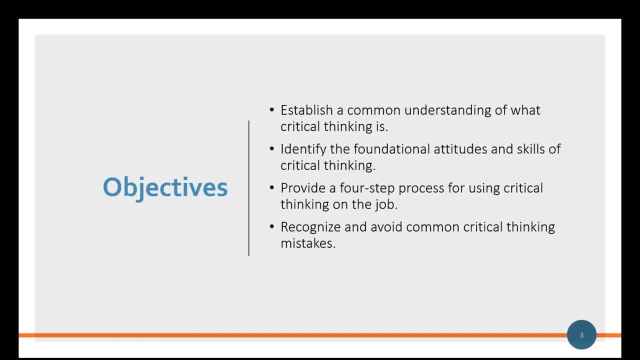 As Sarah said, today's topic is around critical thinking, which is all about enhancing judgment and the quality of your decisions overall, And we're going to take time to cover four primary objectives. We're going to talk a little bit about what we mean by critical thinking. 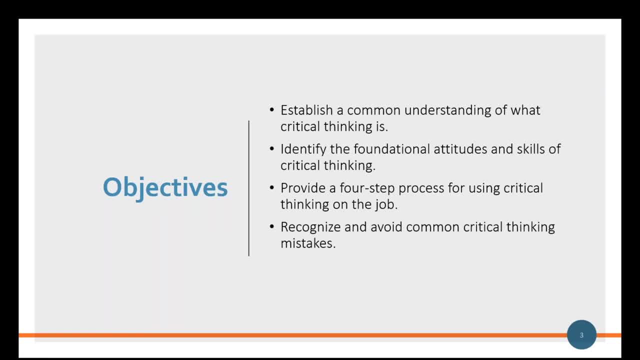 what it actually is, what it actually looks like in practice. We'll talk about some of the basic skills, the attitudes, the characteristics of effective critical thinkers. We'll walk through a four-step process for critical thinking and really the importance of that is that critical. 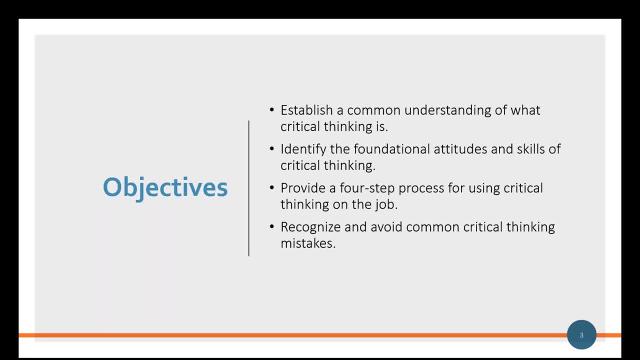 thinking is a skill you can learn. Some people may be born with a tendency to be more critical in their thinking, but all of us can learn to do this and to do this effectively, And we'll also talk a little bit about some of the common critical thinking mistakes and what you can do. 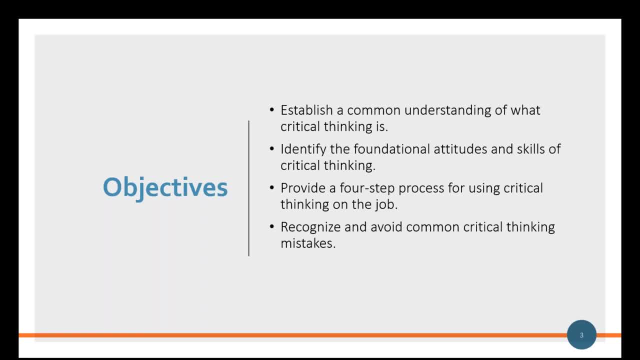 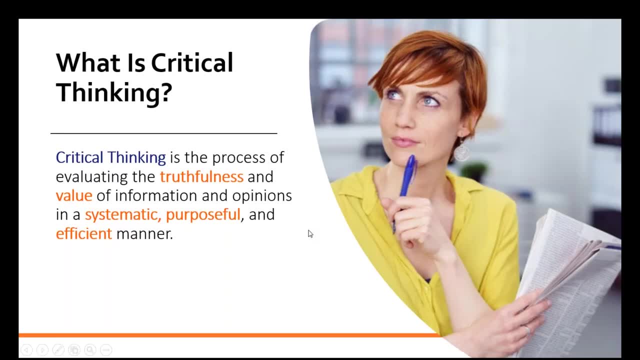 to avoid them overall. So let's start with the definition in terms of what we mean by critical thinking, And critical thinking really is, fundamentally, it's the process by which you go about evaluating the information that you're receiving, And you're evaluating it in terms of its truthfulness. 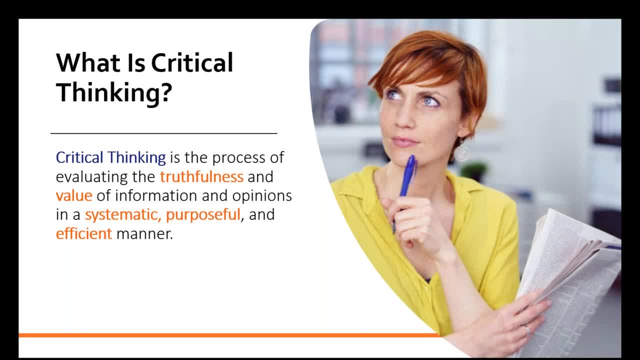 and its value overall. But you're doing this in a systematic way, in a way that is directive and that is efficient overall. And you're doing this in a systematic way, in a way that is effective overall. So it really is thinking a little bit about the information you're. 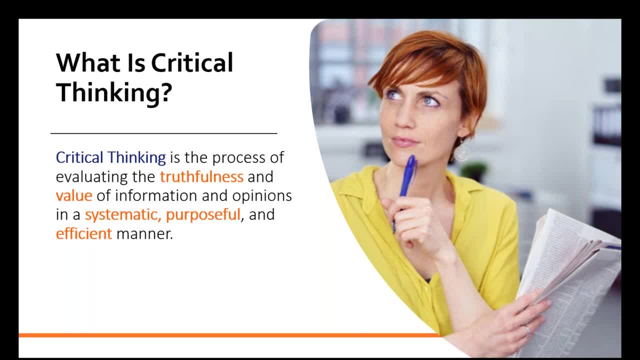 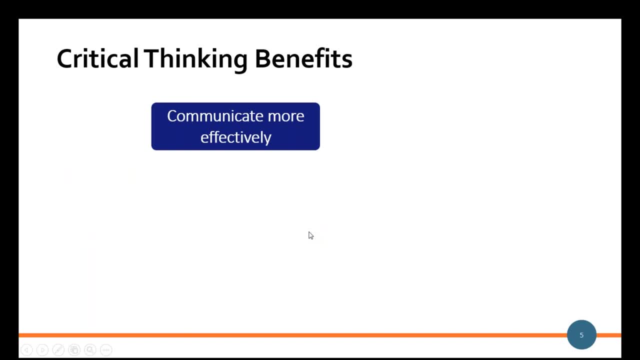 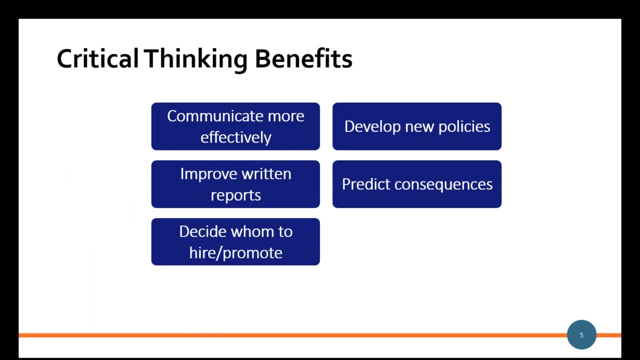 getting, in terms of how accurate is it and is it of use to me in general? So in terms of the benefits, I think we spoke a little bit before that critical thinking is kind of a baseline or fundamental skill or competence that would impact any number. 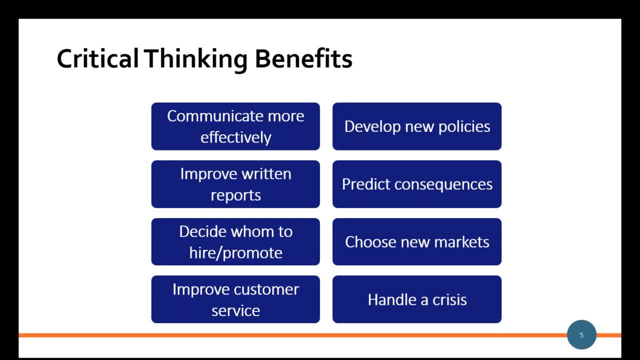 of related activities that you can see listed here. It would certainly improve communication. It can help in your written communication as well. When it comes to making decisions on the job about choosing new markets, handling a crisis, deciding who to hire, critical thinking. 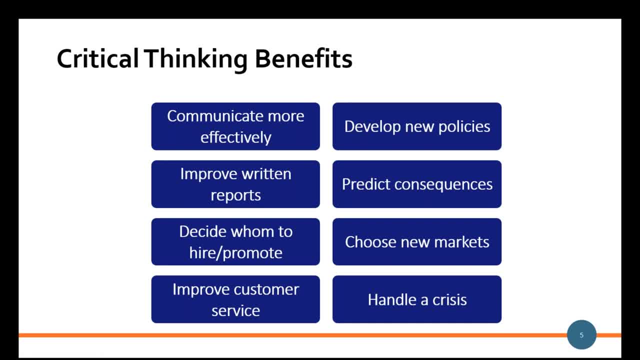 is sort of fundamental to being able to do those things well. The challenge for many of us in a very busy, stressful world is to take the time right and to avoid old habits and biases that may negatively impact our ability to really think through the situation and the information that we're getting. 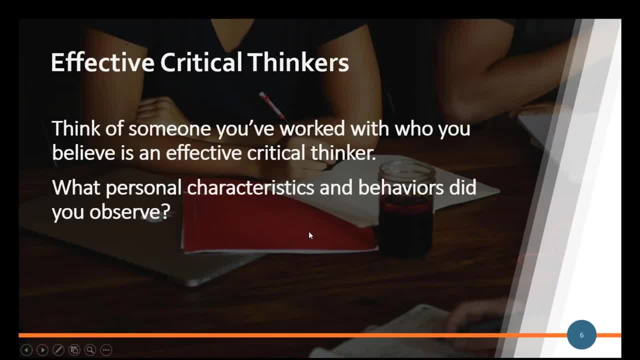 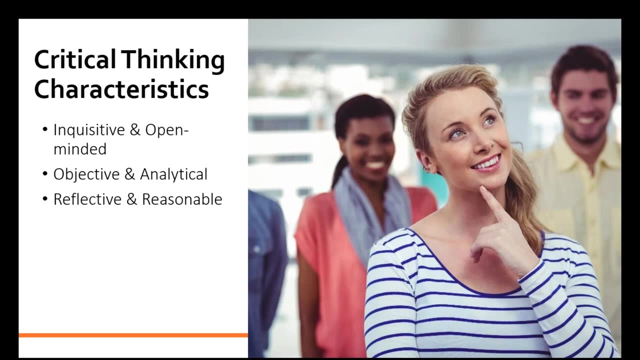 When you think about the people who are the most effective critical thinkers. there are a number of characteristics Dr Kenneth Wesson MD of them share, and it's interesting because some of these things are sort of you might think of them as almost mutually exclusive, but these are people who are inquisitive and open-minded. 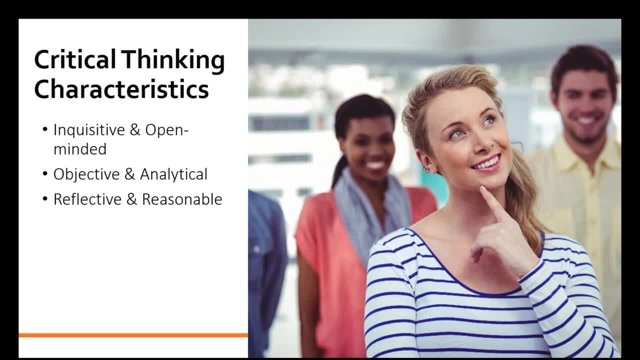 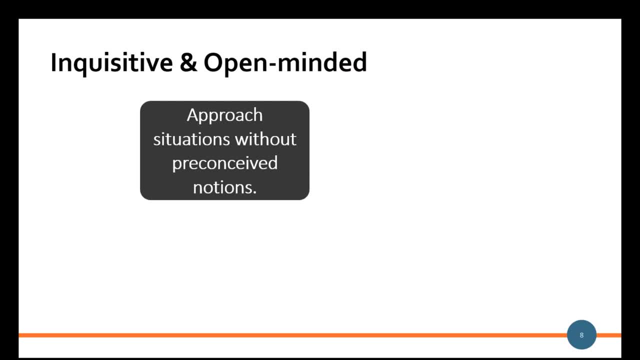 they're objective and analytical, and they're also reflective and reasonable. let's take a look at each one of those in a little bit more detail. in terms of being inquisitive and open-minded, this is really approaching a situation without any preconceived ideas, and this can be very 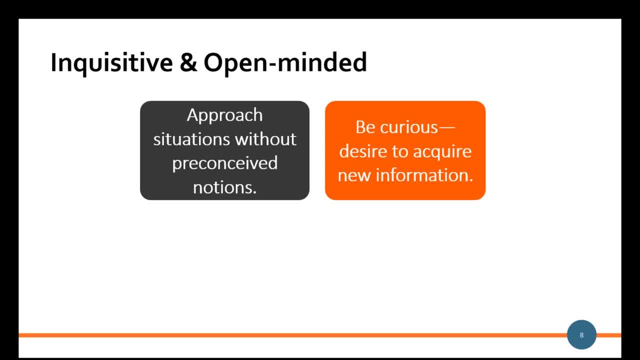 challenging, and one of the things i would suggest is that it's not that all of a sudden we become kind of neutral or all of a sudden being open-minded where we just don't have preconceived notions. the idea here is that with awareness you can check yourself. so you, we all naturally 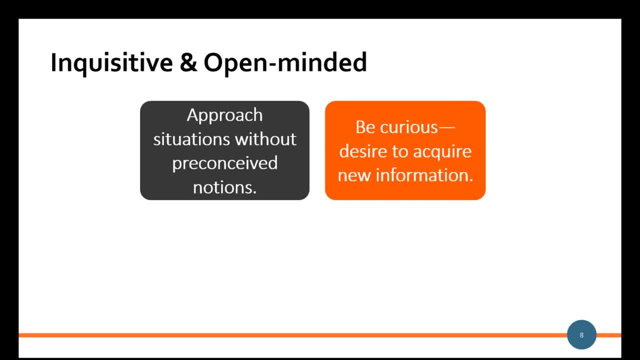 have some preconceived idea you can check yourself. so we all naturally have some preconceived idea about a situation or about a choice or an option or about an individual. The idea is to not let that preconceived idea dominate, to really be able to check yourself and say: 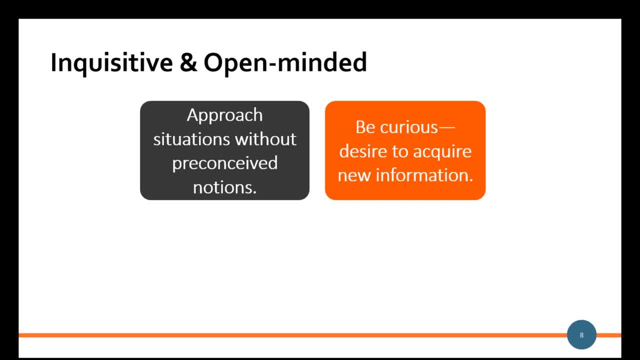 is there other information? Is there another way to look at that? And that's really what we mean by being curious. It's not that you don't have the preconceived idea, it's that you move past it. You're aware of the fact that you do and you move past it. 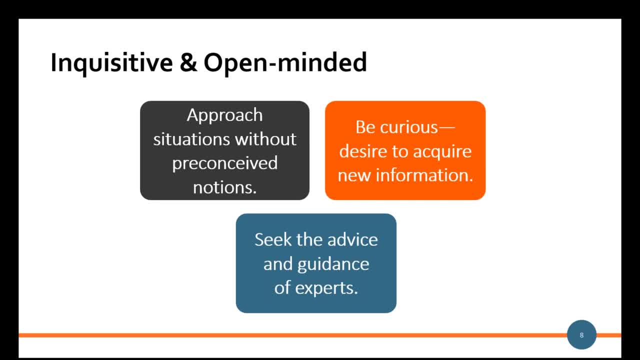 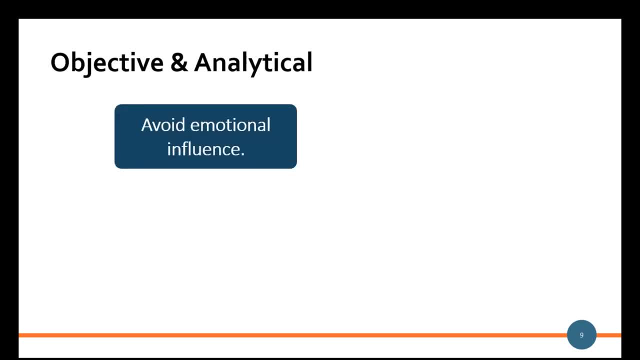 So the idea is that you- and one way to do that may be to check in with other people, trusted advisors, people who are subject matter experts- to give you another perspective on a particular situation. On the objective and analytical side, this is about minimizing the impact of emotion. 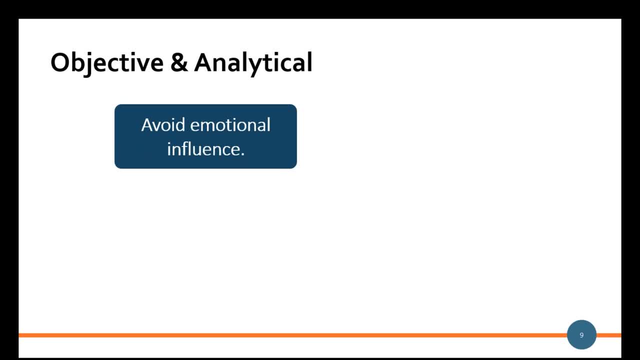 on your decision making, And we can talk about it a little bit later. but it's not that you eliminate emotion, because it's an important component of the decision making process, but you also wanna be as objective as possible And in terms of being analytic, 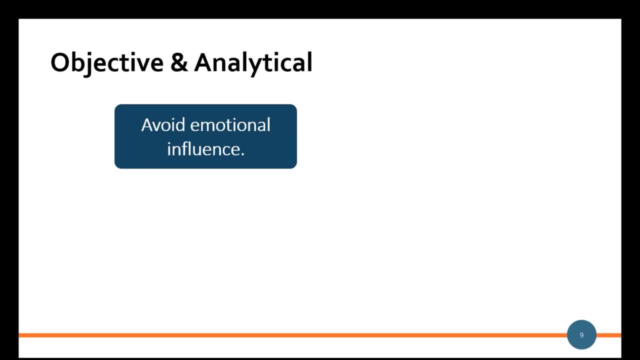 to be able to assess the data that's in front of you and to be able to determine, of all the information you're getting, which is most important and which is most useful. And the key here is being able to separate facts from opinion, And that becomes very challenging in today's world. 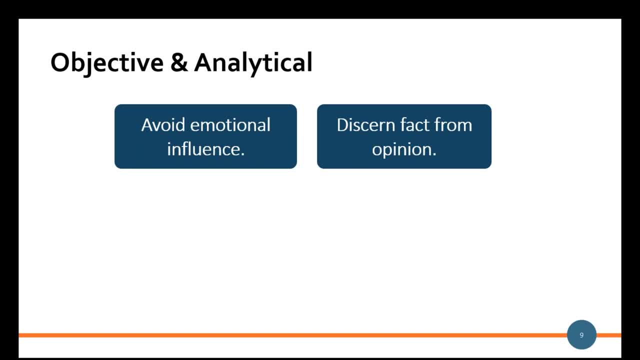 What is a fact? We used to know what that was, but for some reason it's not as clear as it used to be from someone's opinion. overall, The main difference is that facts can be proved or disproved. Facts have some kind of backup information. 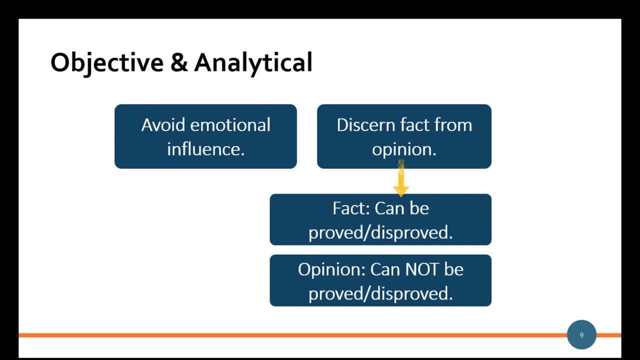 and it's objective, it's unbiased Opinion is something that it's a point of view that I have, that I may or may not be able to provide some supporting information. So the whole idea here is to avoid taking opinions and presenting them as if, in fact, they were facts. 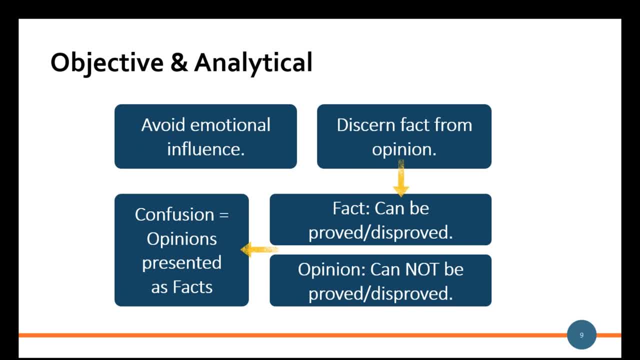 Now, the key here again is not so much what you expect other people to do, but it's really on the receiving side- is, as you're listening, as you're reading, to really say what's the basis of this, What's behind this overall. 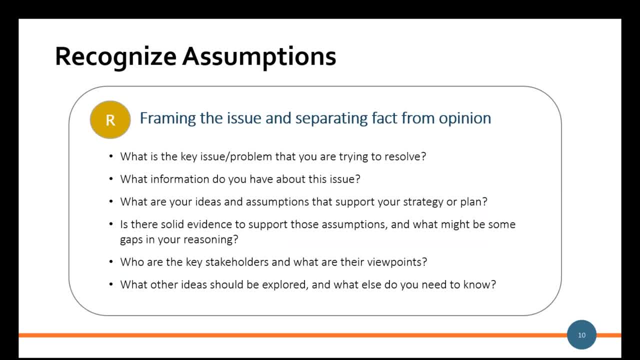 And there are a couple of key questions that you can use to help you separate facts from opinion. overall, To really think about the key issue or the problem you're trying to resolve, What information do you have about the issue Or what assumptions do you have or ideas? 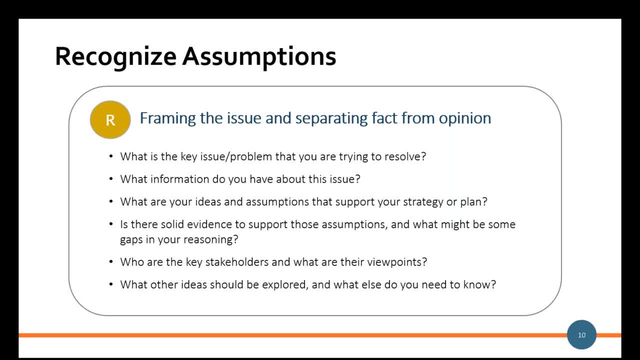 that support your strategy or plan? Is there evidence to support these assumptions? What might be gaps in reasoning? And to really pose these questions to yourself or to the team, to really help you think it through, To not necessarily just take the information as given. 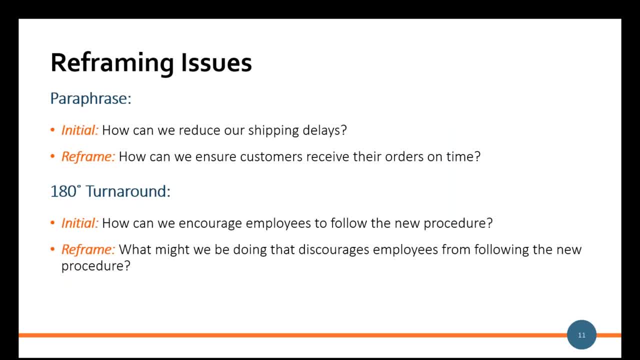 that it will be true and accurate. Another technique to help you rethink or reframe the problem, to give you a fresh point of view on it, is reframing, And there are four different ways to reframe an issue or a problem, And one is paraphrasing. 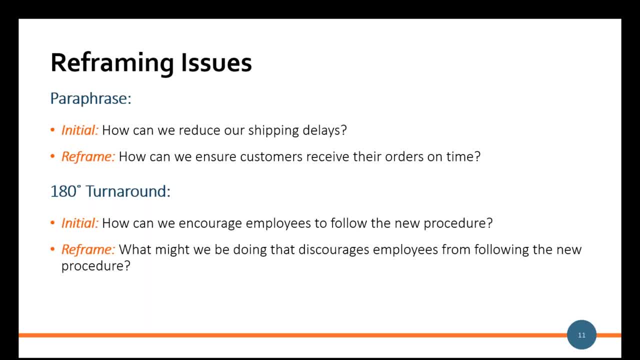 So your initial view or issue is: how can we reduce our shipping delays? If you were going to reframe it using paraphrasing, you might say: how can we ensure customers receive their orders on time? And looking at it through a different lens, 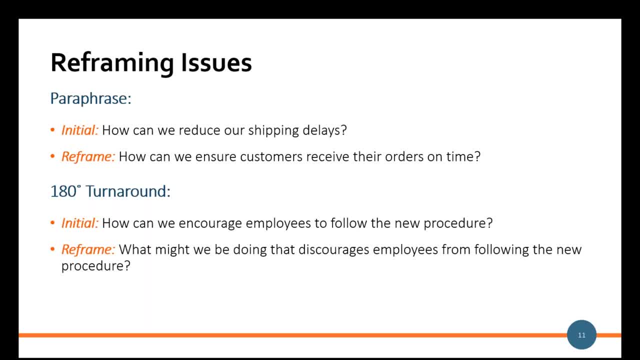 helps you start to think through and separate opinion from facts going forward. The other is a 180 turnaround. If initially you're thinking about how can we encourage employees to follow the new procedure, If you flipped it around 180 degrees you might say: 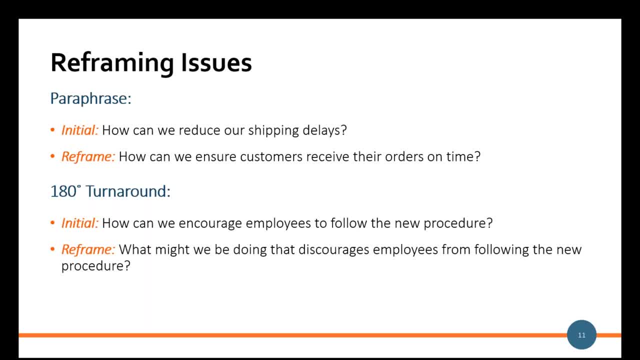 what might we be doing to discourage employees from following the new procedure? To put a different lens on it. The third is to broaden it or expand it. If initially you're thinking, should we expand our product line in China, You might reframe it by saying: 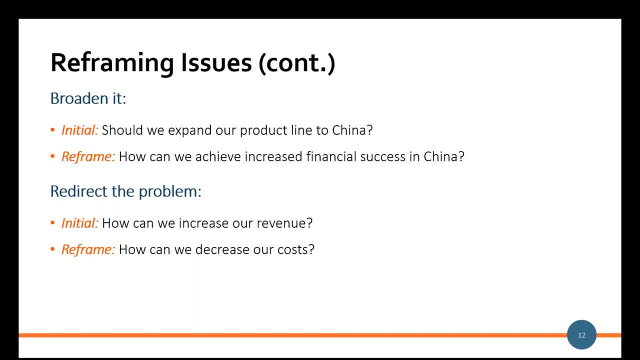 how can we achieve increased financial success in China, Or to redirect it. If initially you're posing the question how can we increase revenue, To reframe it by saying: how can we decrease our costs? Again, the idea here is to put a different lens on things. 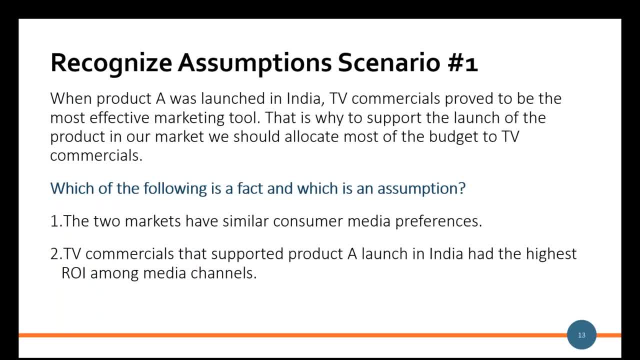 to get a different point of view. So let's see how, in terms of your ability to determine which is a fact and which is an assumption- And we'll be doing a number of these during the course of our time together to give you an opportunity. 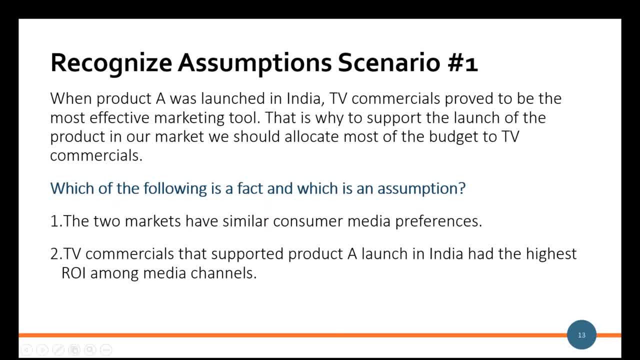 to test your critical thinking skills. So let's take a look at the first scenario around recognizing assumptions. When product A was launched in India, TV commercials proved to be the most effective marketing tool. That's why, to support the launch of the product in our market, we should allocate most of the budget. 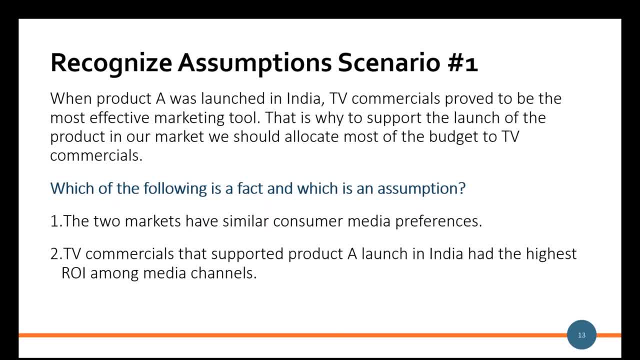 to TV commercial. So which of the following is a fact or an assumption? Number one: the two markets have similar consumer media preferences. Is that a fact or is that an assumption? And number two: TV commercials that supported product A launch in India. 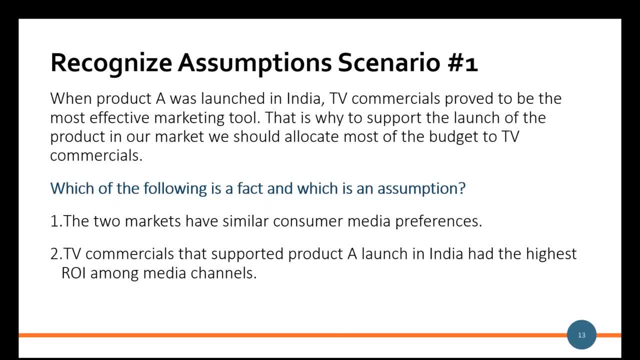 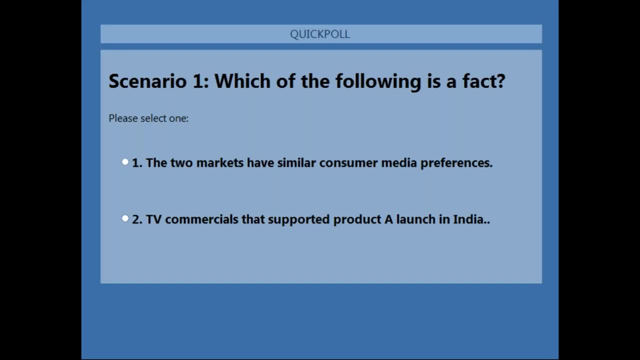 had the highest ROI among media channels, And just use the information that you've been presented in this little mini case without adding too much to it. But Sarah's putting up the polling question right now, And which one? This one is a fact. 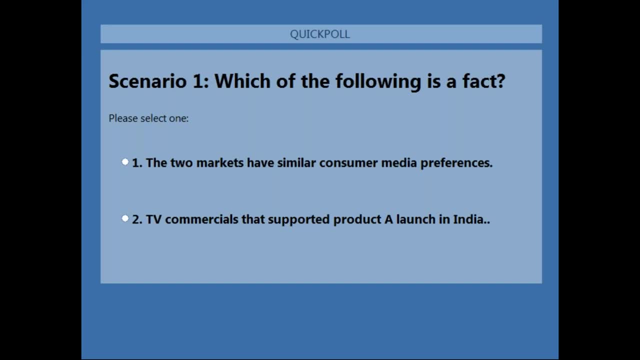 Pick the one you think is a fact And we'll keep it open for a few moments And, Sarah, you can close it when we get about half or so, depending on how fast they're coming in. OK, So most people picked the second one: TV commercials. 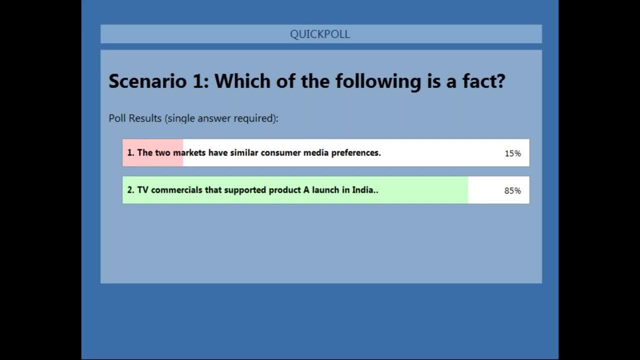 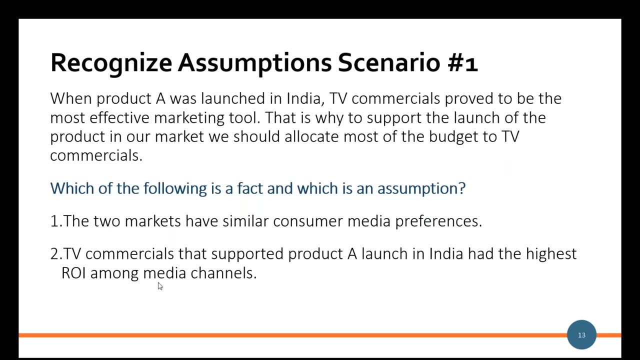 have that supported? the product launch in India tend to be the fact. So, Sarah, if you close that down, we'll take a look at the right answer. And in fact, that is the correct answer. The first one: the two markets have similar consumer media preferences- is an assumption. 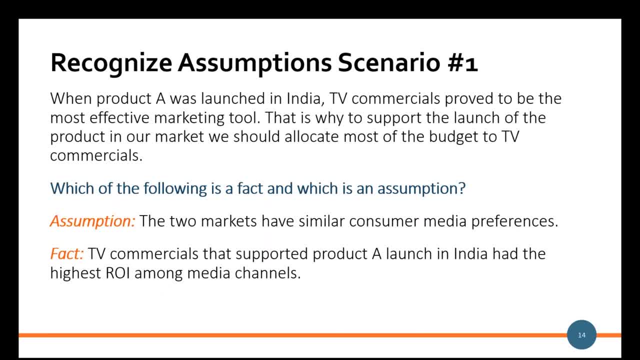 that's being made. There's no information in the little scenario that indicates that they had the same preferences, but you do have some information that can be supported that says it had the best return on investment overall. Let's take a look at a second scenario. 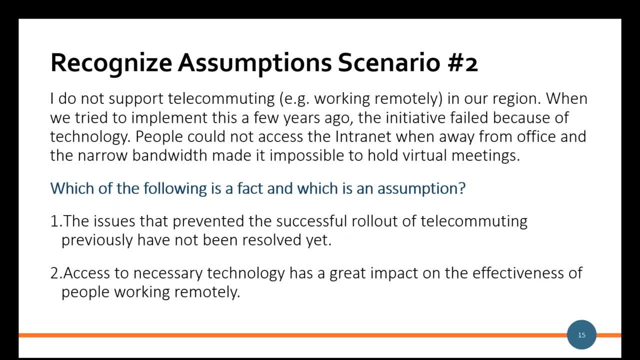 And here I do not support telecommuting in our region. When we tried to implement this a few years ago, the initiative failed because of technology. People could not access the internet, went away from the office and the narrow bandwidth made it impossible to hold virtual. 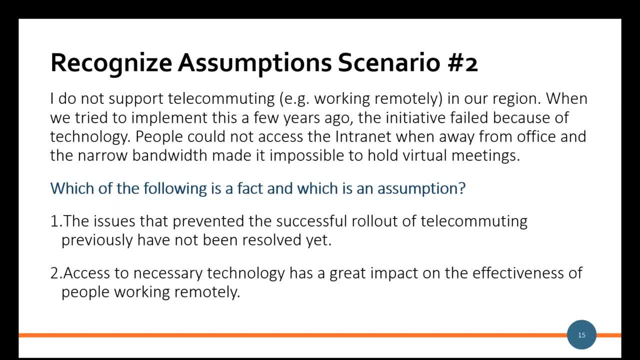 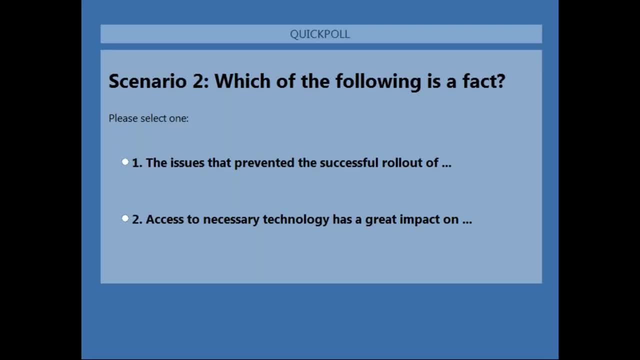 meetings. so which of the following is a fact? the issues that prevented the successful rollout of telecommuting previously have not been resolved, or access to necessary technology has a great impact on the effectiveness of people working remotely. and, sarah, if you put up the poll, and which one of these statements is the fact, 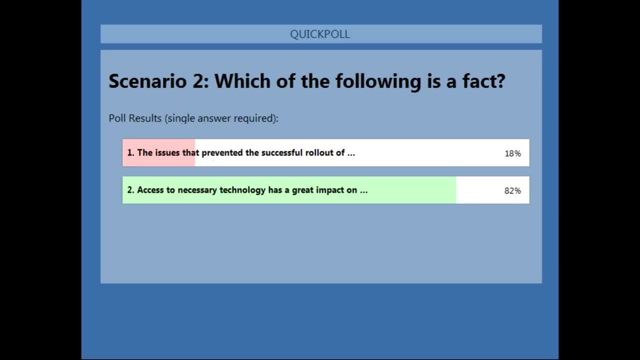 all right, sarah, you can close it whenever. oh, there we go. okay, let's take a look at the results. so again, uh, people selected number two. access to technology has a great impact, and the um. most people take that as a fact. overall, let's take a look at the. and, in fact, that is a fact. 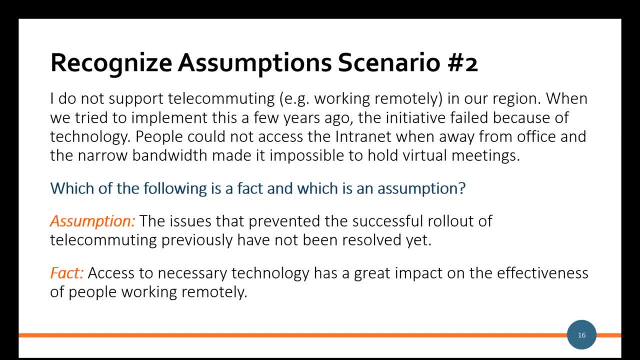 is the correct answer. We do know that, based on this scenario that access is critical- We do not have any real data that says these issues have not been resolved. This particular person who's speaking is assuming that the issues have not been resolved. 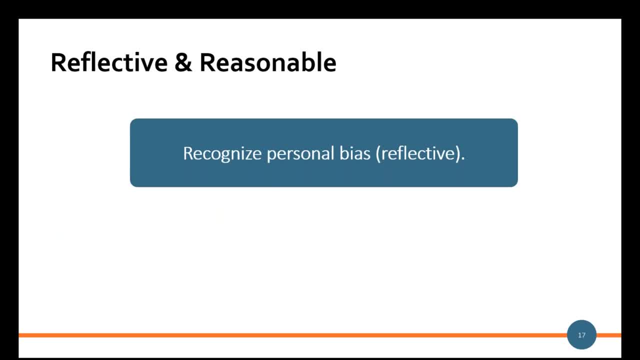 but there's no information in this particular case that would indicate that The second is around being reflective and reasonable, And here we're talking about personal bias and avoiding personal bias and applying common sense. And again, the key here on personal bias, it's not that you won't have bias and preferences. 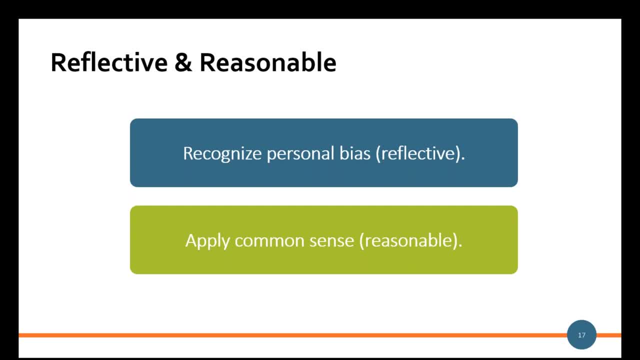 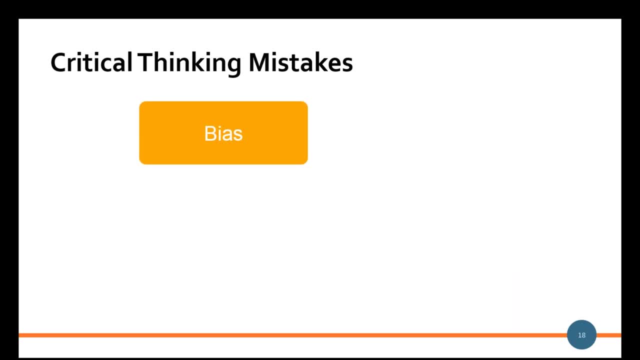 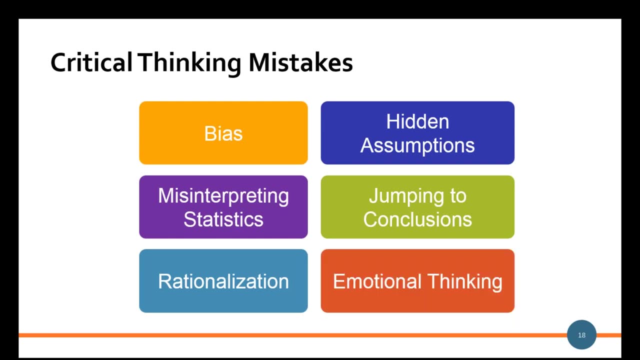 The challenge is to recognize it and recognize when it's affecting your choices and your decisions. So, when we think about some mistakes that individuals make, there's a number of them and they have to do with bias, with hidden assumptions, with misinterpreting statistics. 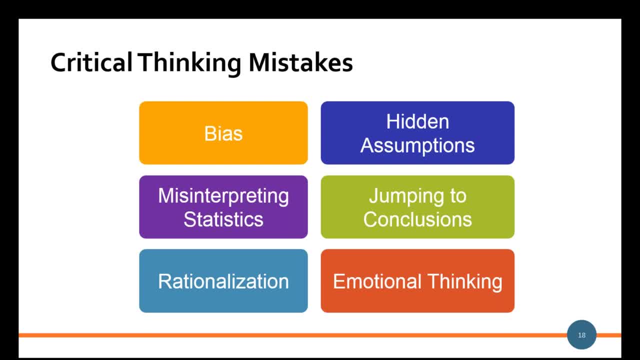 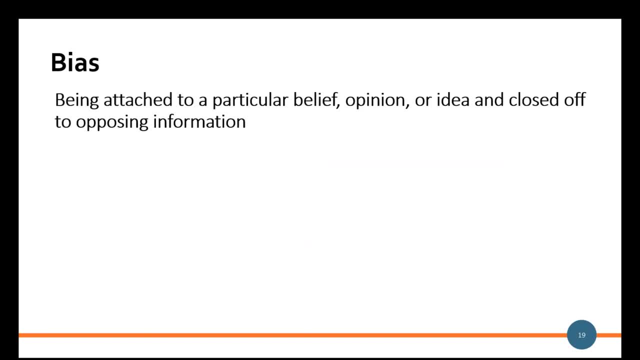 jumping to conclusions, rationalizing and emotional thinking, And let's take a look at each one of those in a little bit more detail. Biases is about being attached to a particular belief and closed off to information that runs counter to that overall. 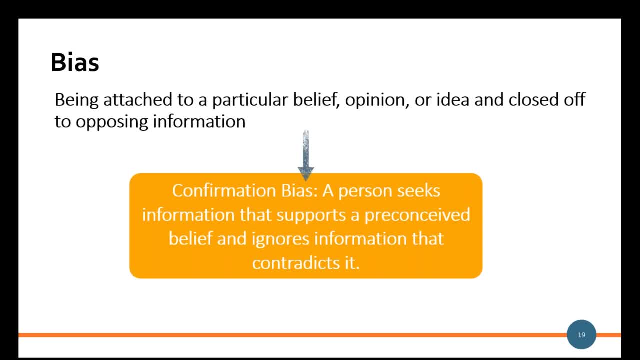 So we have the idea of a confirmation bias, where you're only looking for information that supports your conclusion. You draw the conclusion, then look for information that supports it and do not attend to other data. Again, it's not. it's almost human nature to do it. 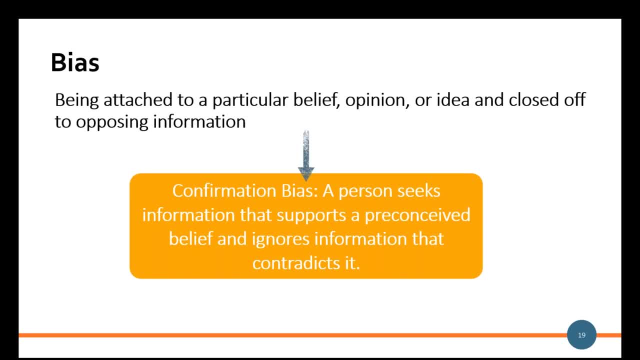 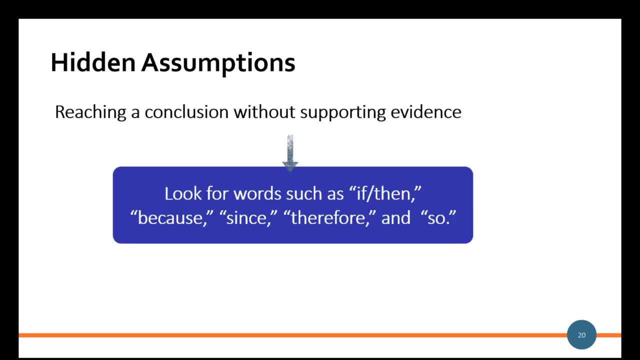 It's the awareness that it's happening, it's recognizing so you can stop it from happening. Hidden assumptions is about reaching a conclusion without supporting evidence. right, So it's just. I believe this. I don't. there may not be any data around it. 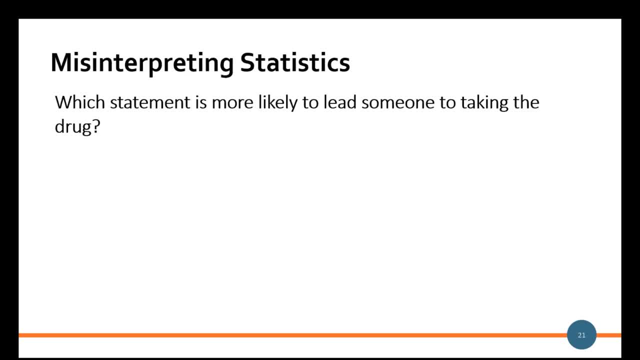 but I believe it overall. The misinterpreting statistics, and I think this is particularly interesting, especially against this notion of what's a fact. I thought it was a fact, but what is a fact? And there's this idea about misinterpreting. 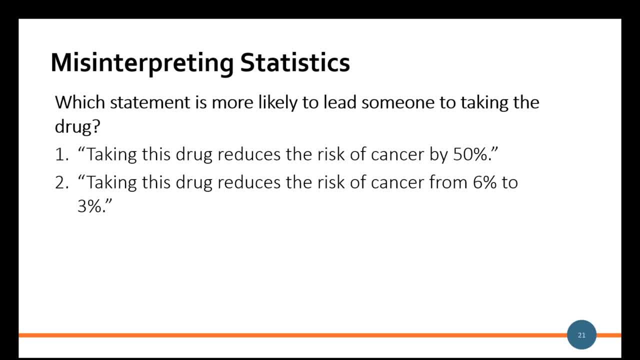 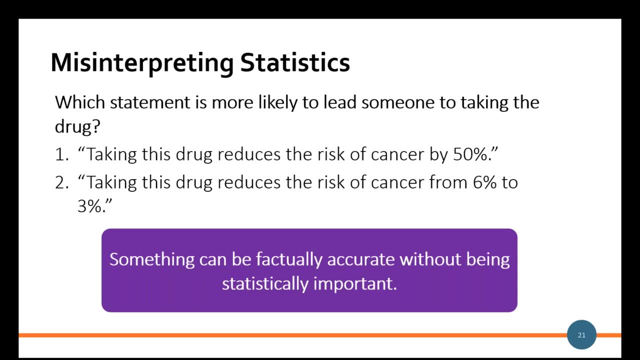 or misusing statistics overall. So, if you take a look at these two items, taking this drug reduces the risk of cancer by 50%. taking this drug reduces the risk of cancer from 6% to 3%. right, So which one would be most? 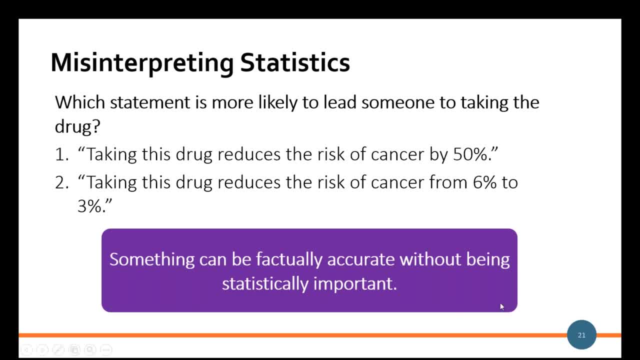 most convincing to you, right? For most people taking the drug, the drug reduces the risk of cancer by 50%. seems much better than reducing the risk of cancer from six to 3%. However, it's the same statistic. It's just being presented or said in a different way. 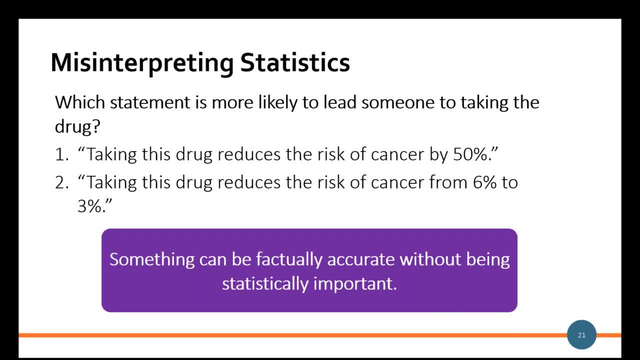 So you could in fact, take something that's truthful, that's factual, but it might not necessarily be statistically important, Okay or significant in terms of the conversation overall. And I think again, in many ways people manipulate data to put the best spin on it, And part of critical thinking is to really 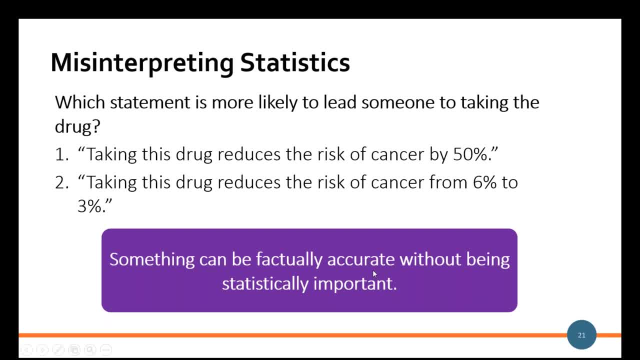 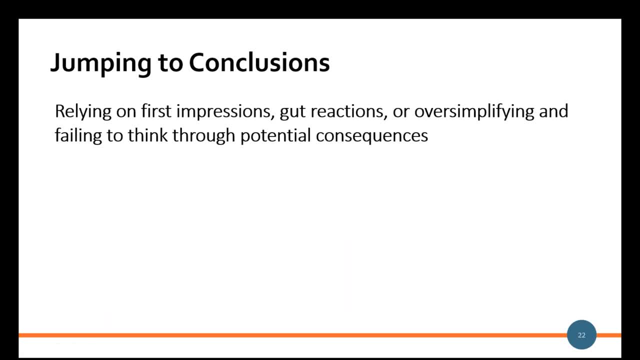 dig in to understand the implication of that data and what the meaning is overall. The other is around jumping to conclusions And this is about going with first impression, right, your gut reaction, And this is a little bit about the emotional side as well. This is: 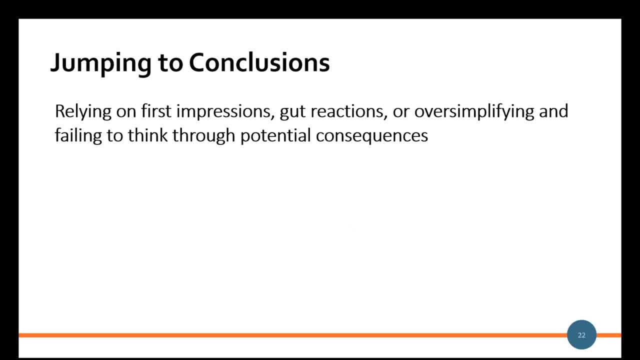 how I feel about it, This is what I believe, This is my experience, So it must be true, overall, right, And you're trying to just be aware, because this can be a result of stress, of time pressure that causes us to move to what we think is the easiest conclusion. 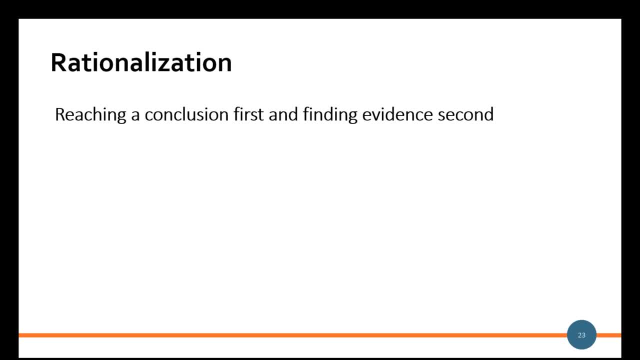 The idea of rationalization is basically reaching a conclusion and then looking for evidence. right, So we have an opinion and then we look for data that supports it overall, The emotional thinking is the idea of reacting emotionally, And it could be because of the 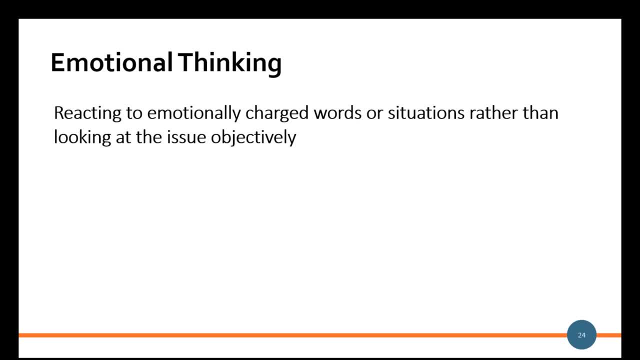 language. the other person is using the situation, the stakes that are high, rather than being more objective. And I would say to you: in these situations, it's not so much to eliminate feeling, to eliminate your gut reaction, But what you want to do is make. 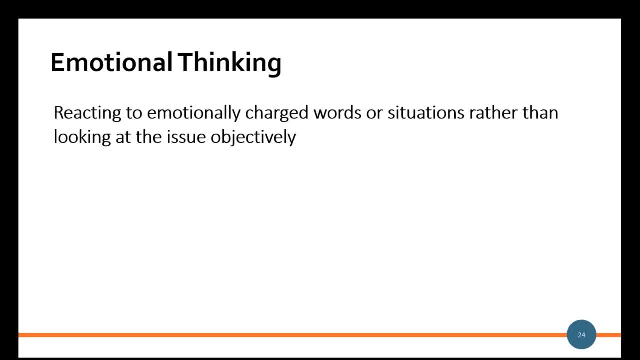 sure that you're not just thinking about the situation but you're also thinking about the balance. You want both your right brain and your left brain to sort of be operating together so that you have kind of the best of both worlds. You have the subjective, the objective, analytic. 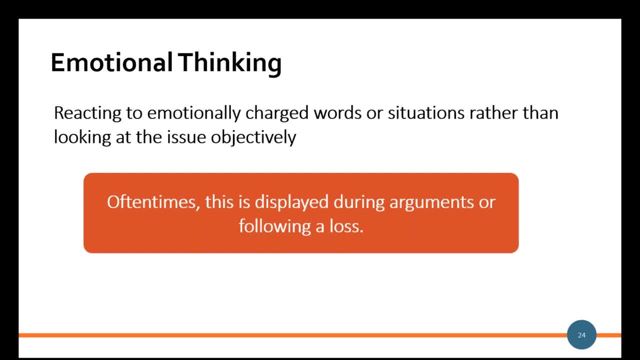 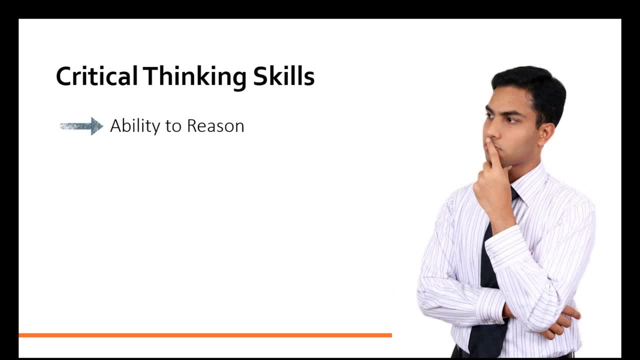 side and you have the subjective sort of gut feeling And then you can sort of put those two things together. So, moving to critical thinking skills overall, and there are three of them: the ability to reason, the ability, the ability to predict and the ability to evaluate. Once again, these are all learned. 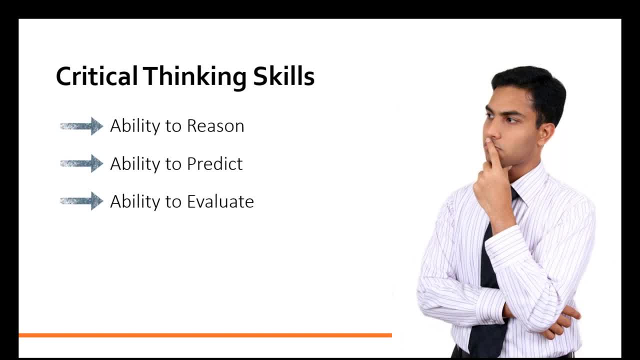 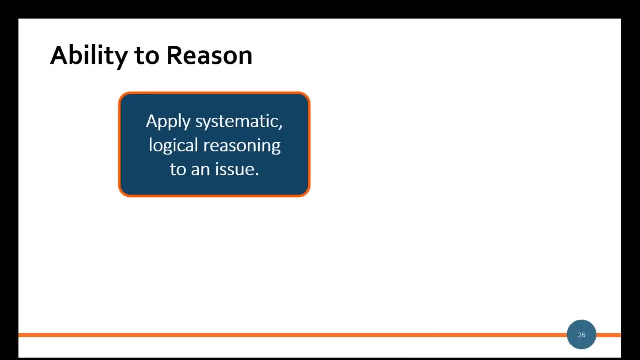 skills. Some of us have more of a tendency to them, but these are all things we can all learn and enhance our ability. So the whole idea of the ability, the reason it's about applying systematic, logical reasoning to an issue. overall, The key here is being able to. 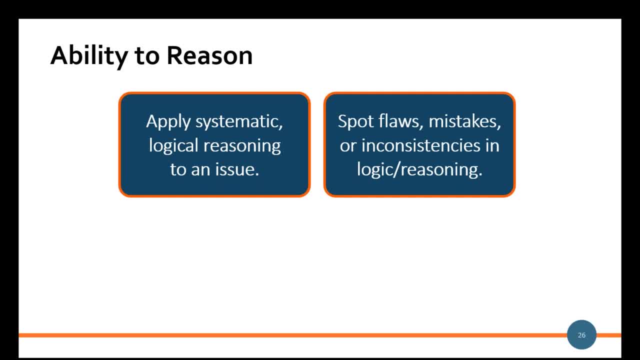 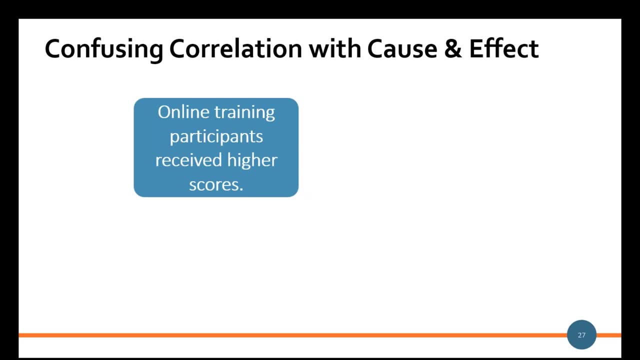 find mistakes, inconsistencies in logic and reasoning and to take the time to actually look for them. overall, right, You want to find and surface hidden assumptions. overall, The idea of thinking about cause and effect and to avoid confusing. that is part of that analytic thinking. So, for example, 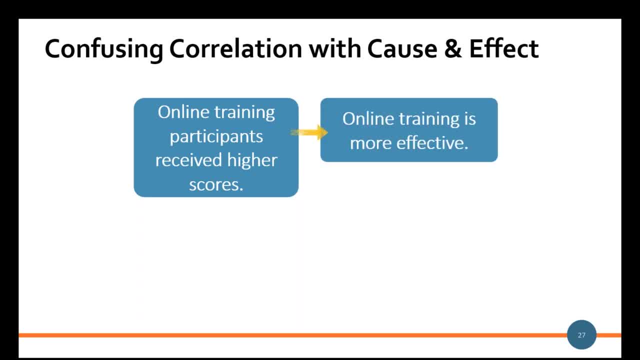 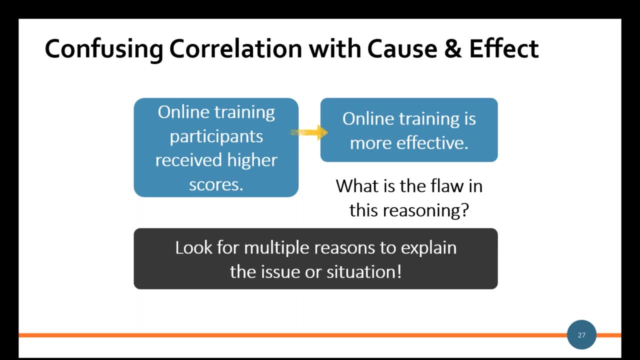 you have online training, participants receive higher scores. So the you know. the conclusion would be: online training is more effective. However, the problem with that reasoning is that there are probably multiple reasons that might contribute to that outcome. So, even though there might be a relationship between those two, 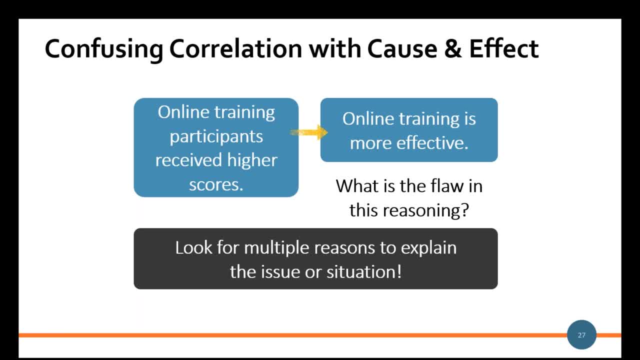 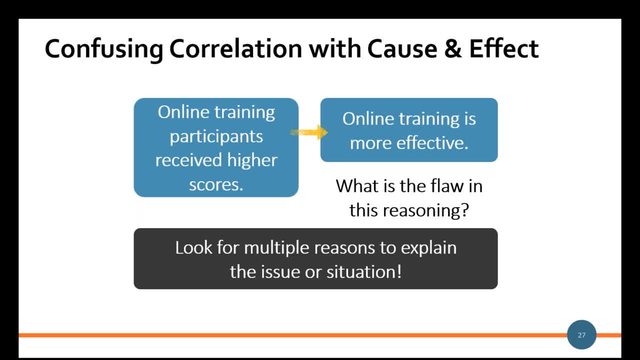 people who don't smoke or smoke. you know people who don't smoke or smoke. you know people who don't smoke or smoke, or people who you know eat kumquats or live longer. Well, there may be a relationship between those two factors. 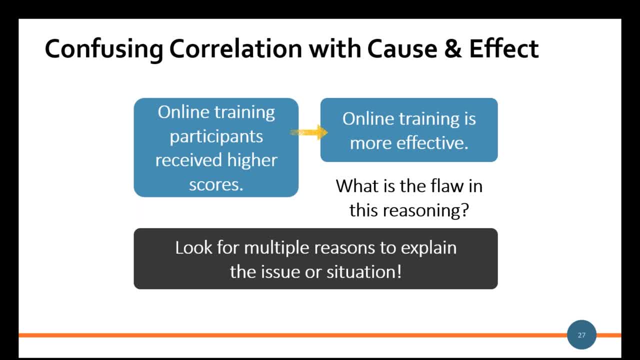 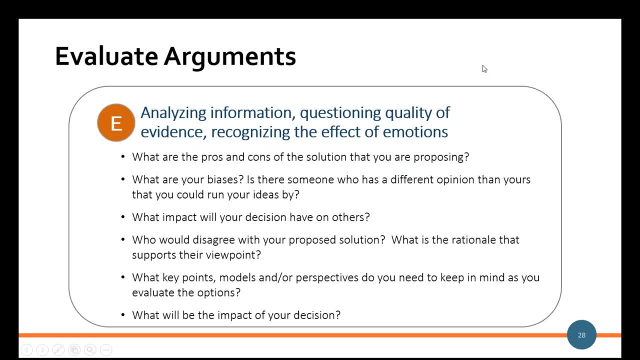 but it doesn't necessarily mean that one causes the other, And that's where we need to be more discerning, more critical, more focused in terms of our thinking. A couple of questions you can use to help you recognize the quality of the information and the evidence that you have. 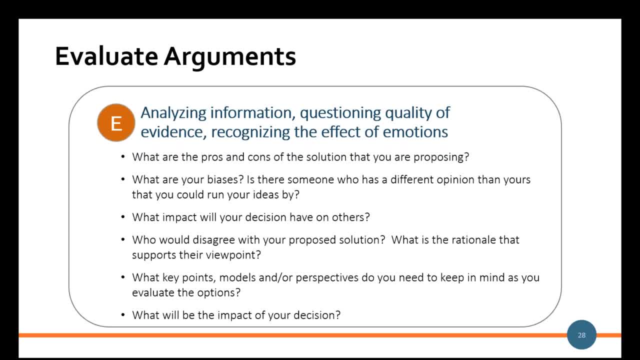 And to be able to recognize the effect of your emotions on when you're evaluating arguments is to think about the pros and cons, to really step back and say what are my biases And to be explicit about exploring that. to think about the impact of the decision on other people, think about who. 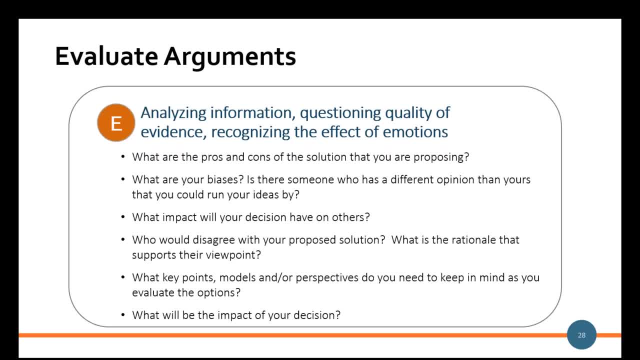 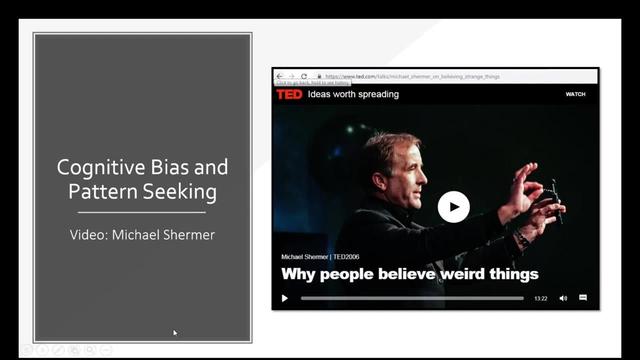 would agree or disagree with the proposed solution and think about key points, perspectives that you need to keep in mind as you're evaluating. So part of this is not so much to let critical thinking just happen. It really is the application of some key questions overall. The other idea- sorry, let me just go back- is to use this idea. 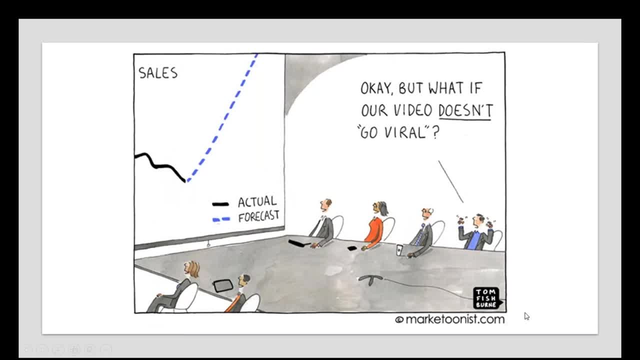 of the devil's advocate, You really do want to have what-if questions. We frequently try to suppress people who are asking what-if questions. We try to suppress people who are asking what-if questions And we try to suppress people who are asking what-if questions And we try to suppress 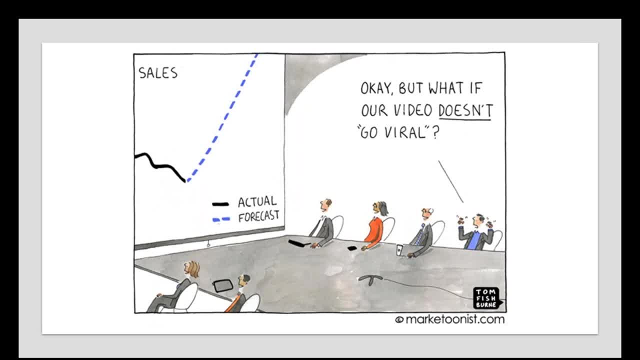 people who are asking what-if questions, And we try to suppress people who are asking what-if questions Because they tend to slow things down. We see it as not being a team player And we really want to get on to the next task overall. So when people raise the, well, what if it doesn't? or what if it? 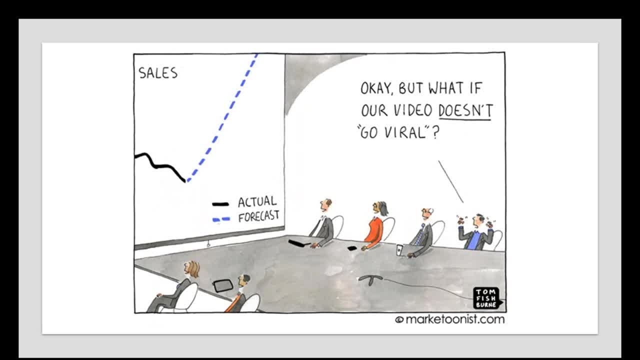 does, or what if it could. we really aren't open to that, But in point of fact, we should be doing the opposite. We should be encouraging this kind of questioning, this kind of raising these kinds of issues to get us to look at the other side of things. 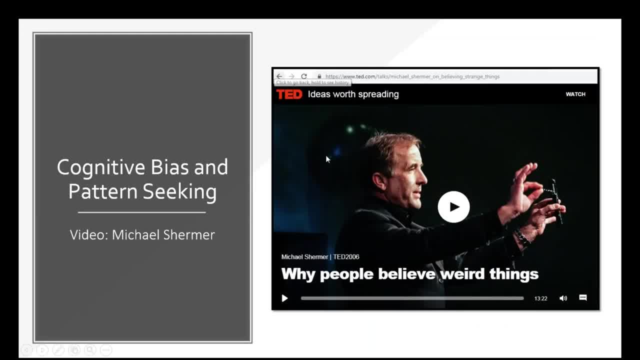 This idea of evaluating information overall, I think is in terms of related to our cognitive biases and how we go about assessing the quality and value of information. I have a video that I'd like to share with you. It's a TED talk. I think you'll find it very, very interesting. It's really. 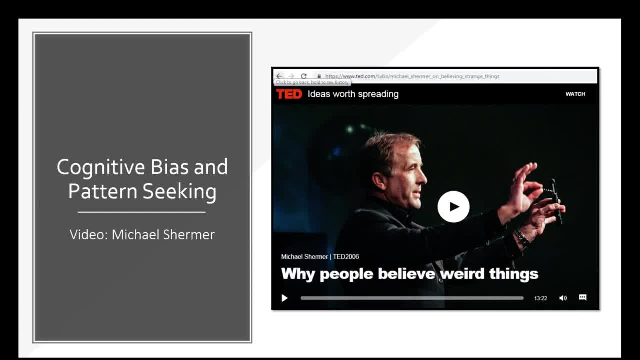 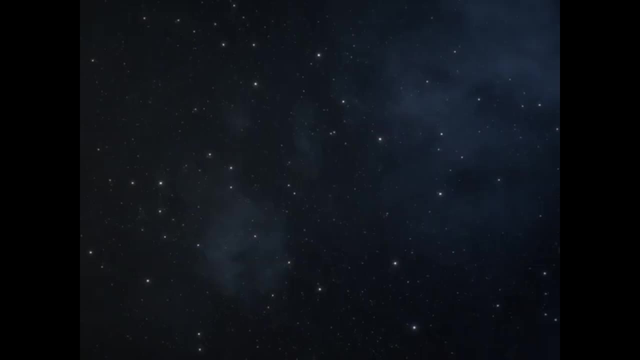 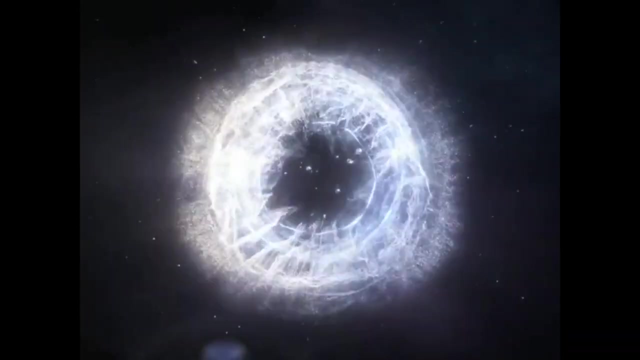 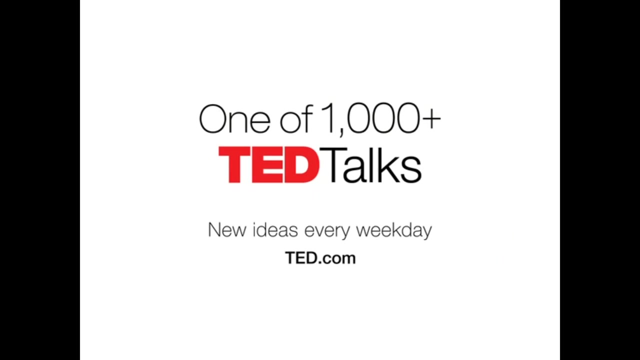 about our tendency to be more biased, to look for patterns, to make assumptions and not to really be particularly critical about the information we're looking at. So, Sarah, if you could start that video for us please? I am Michael Shermer, the director of the Skeptic Society, the publisher of Skeptic Magazine. 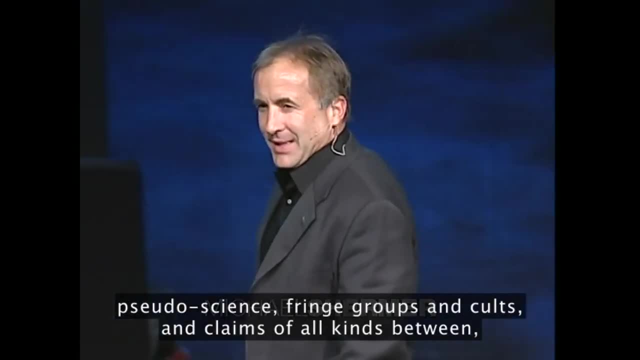 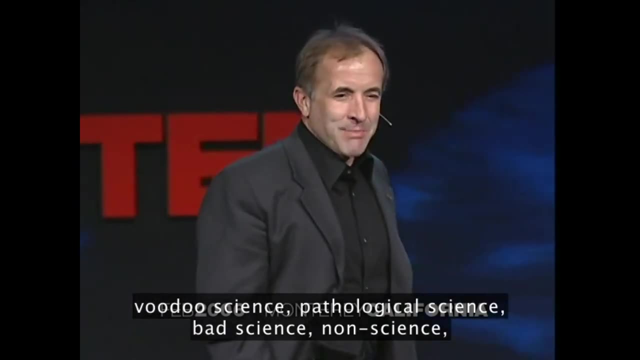 where we investigate the claims of the paranormal, pseudoscience and fringe groups and cults and claims of all kinds between science and pseudoscience and nonscience, junk science, voodoo science, pathological science, bad science, non-science and plain old nonsense. And unless you've been on Mars, 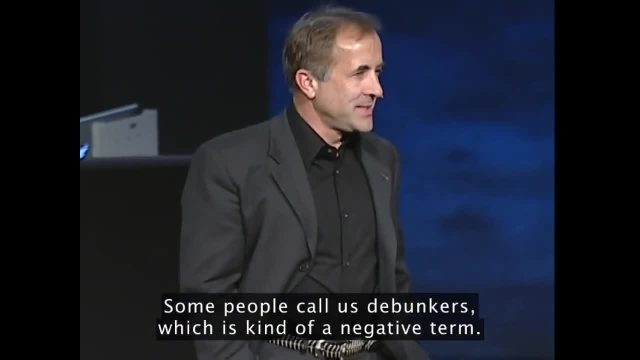 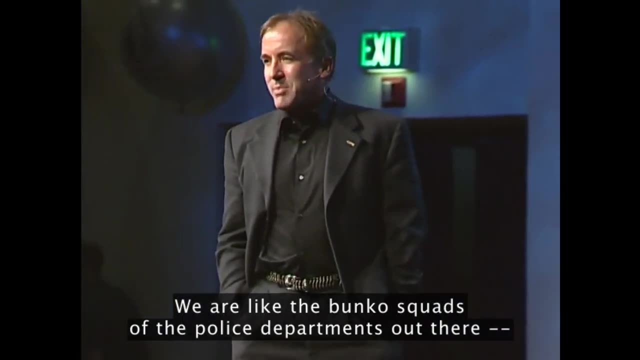 recently. you know there's a lot of that out there. Some people call us debunkers, which is kind of a negative term, but let's face it. there's a lot of bunk And we are like the bunkers, The Bronco squads of the police departments out there flushing out. 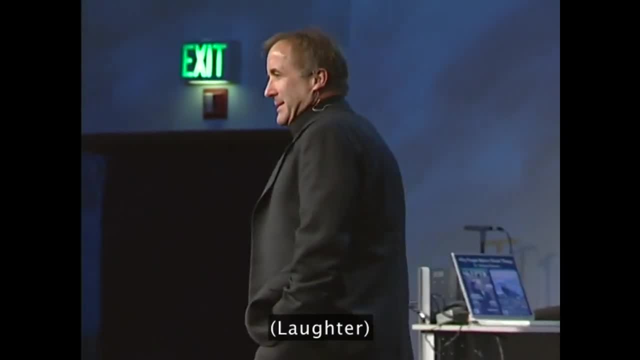 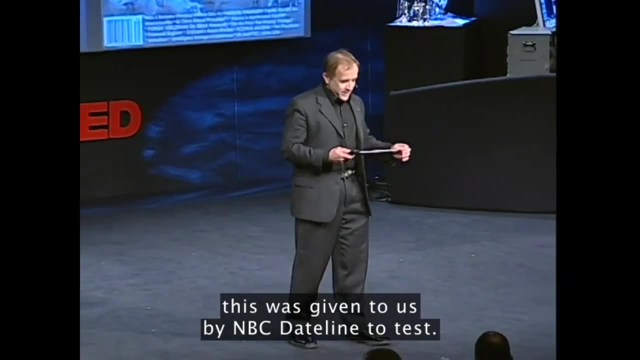 well, we're sort of like the Ralph Nader's of bad ideas, Trying to replace bad ideas with good ideas. I'll show you an example of a bad idea. I brought this with me. This was given to us by NBC Dateline to test. 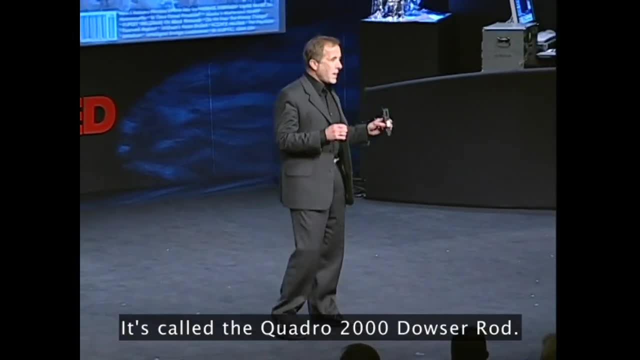 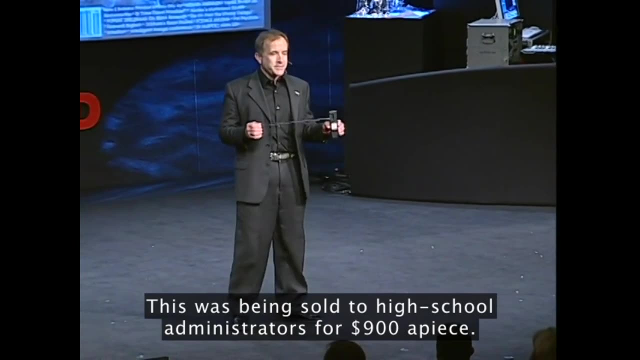 It's produced by the Quadro Corporation of West Virginia. It's called the Quadro 2000 Dowser Rod. This was being sold to high school administrators for $900 a piece. It's a piece of plastic with a Radio Shack antenna attached to it. 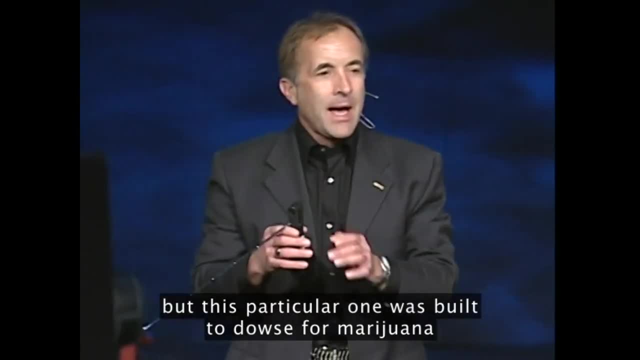 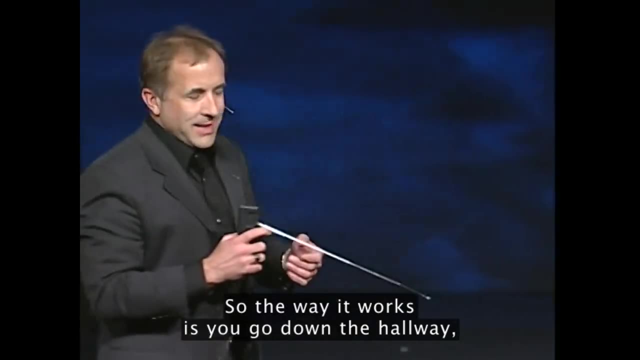 You can douse for all sorts of things, but this particular one was built to douse for marijuana in students' lockers. So the way it works is you go down the hallway and you see if it tilts toward a particular locker, and then you open the locker. 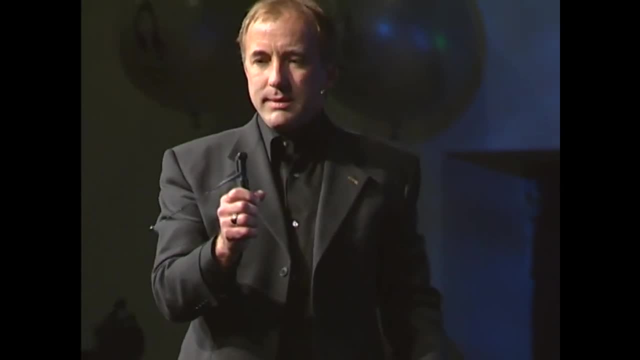 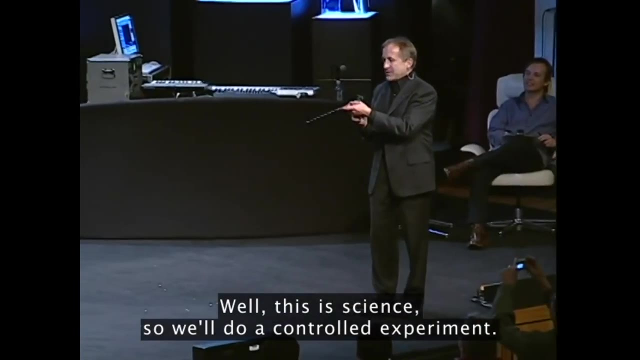 So it looks something like this. I'll show you in a minute. Well, it has kind of a right-leaning bias, so I'll show you. This is science, so we'll do a controlled experiment. It'll go this way, for sure. 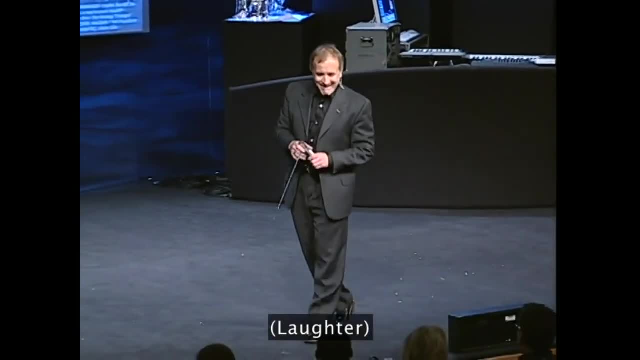 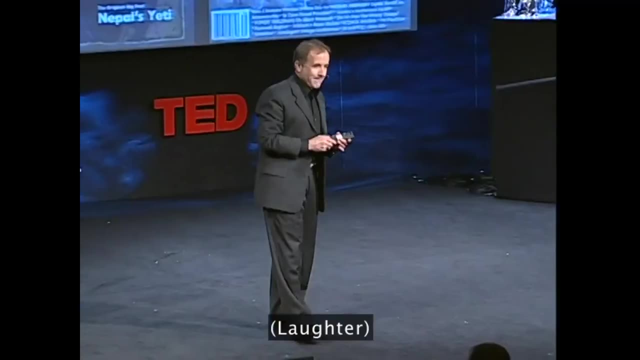 Sir, you want to empty your pockets please, sir. So the question was: can it actually find marijuana in students' lockers? And the answer is: if you open enough of them, yes, But in science we have to keep track of the misses, not just the hits. 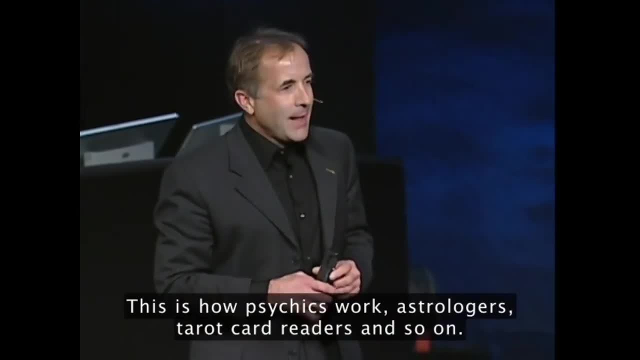 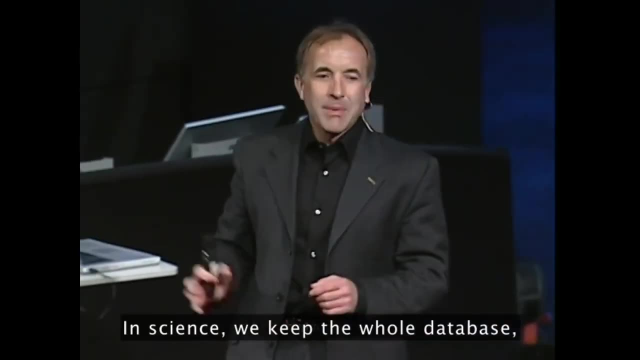 And that's probably the key lesson to my short talk here- is that this is how psychics work, astrologers and tarot card readers and so on. People remember the hits. they forget the misses. In science, we have to keep the whole database and look to see if the number of hits 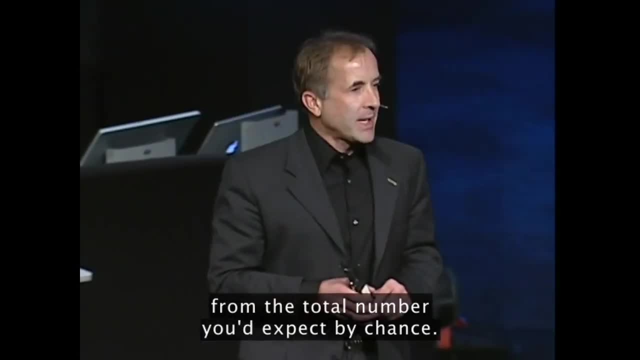 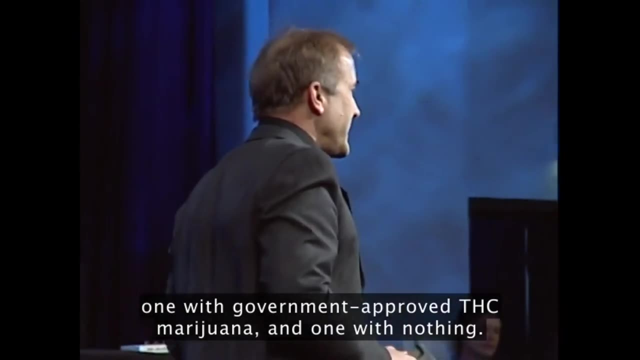 somehow stands out from the total number that you would expect by chance. In this case, we tested it. We had two opaque boxes, one with government-approved THC marijuana and one with nothing, and it got it 50% of the time, which is exactly what you'd expect with a coin flip model. 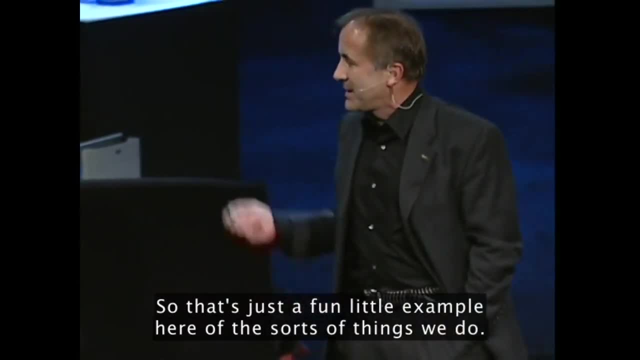 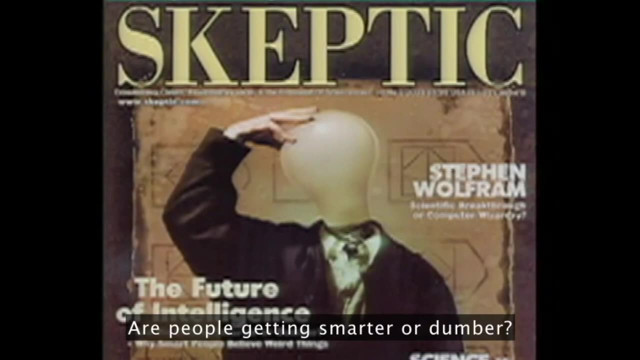 So that's just kind of a fun little example here of the sorts of things we do. Skeptic is the quarterly publication. Each one has a particular theme Like. this one is on the future of intelligence. Are people getting smarter or dumber? 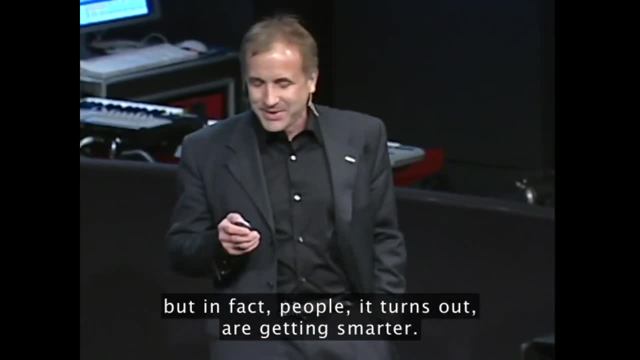 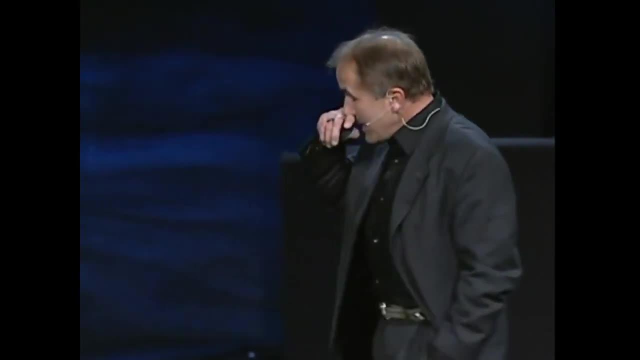 I have an opinion of this myself because of the business I'm in. But in fact people, it turns out, are getting smarter. Three IQ points per 10 years going up. Sort of an interesting thing With science. don't think of skepticism as a thing or even science as a thing. 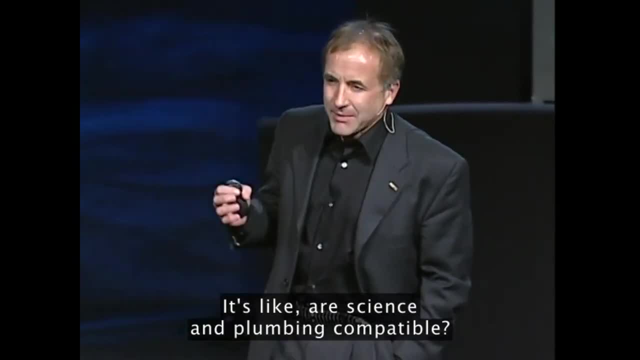 Are science and religion compatible? It's like: is science and plumbing compatible? They're just two different things. Science is not a thing, It's a verb. It's a way of thinking about things. It's a way of looking for natural things. 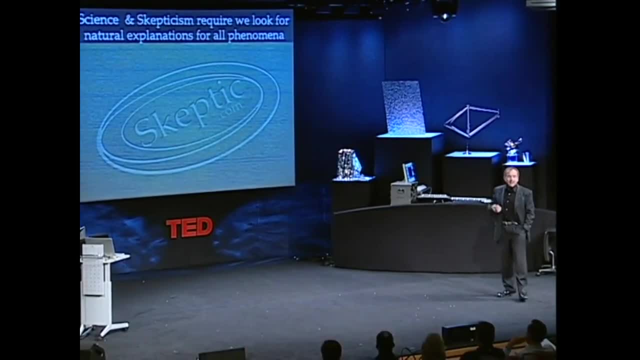 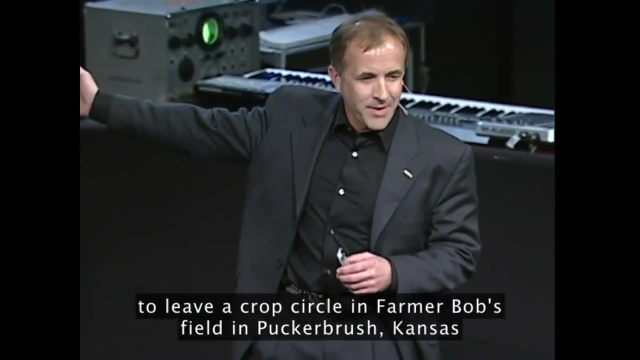 It's natural explanations for all phenomena. I mean, what's more likely that extraterrestrial intelligences or multidimensional beings travel across the vast distances of interstellar space to leave a crop circle in Farmer Bob's Field in Pucker Brush, Kansas? 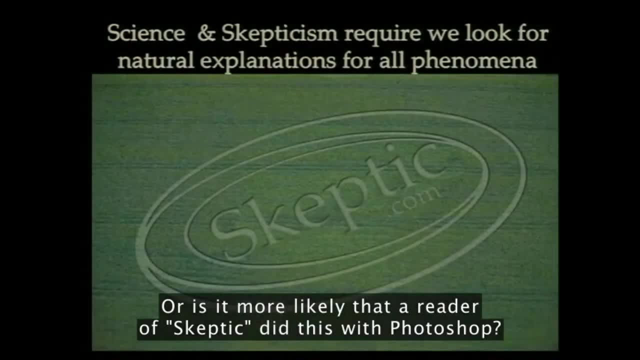 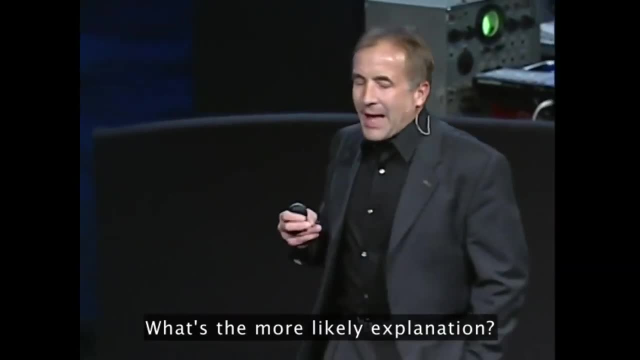 to promote skepticcom, our web page, or is it more likely that a reader of Skeptic did this with Photoshop? And in all cases, we have to ask what's the more likely explanation And before we say, something is out of this world. 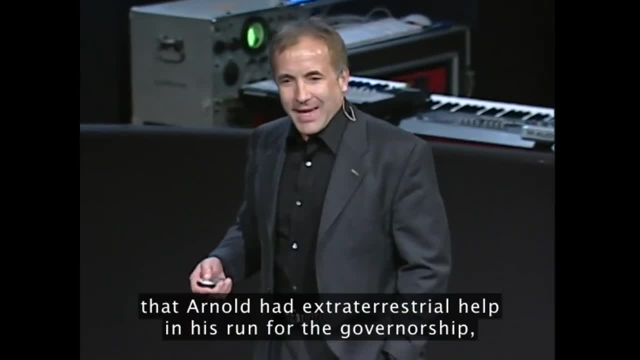 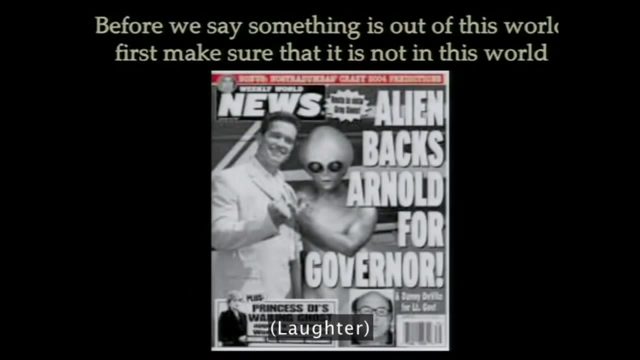 we should first make sure that it's not in this world. It's more likely that Arnold had a little extraterrestrial help in his run for the governorship or that the World Weekly News makes stuff up And part of that. the same theme is expressed nicely here in the Sydney Harris cartoon. 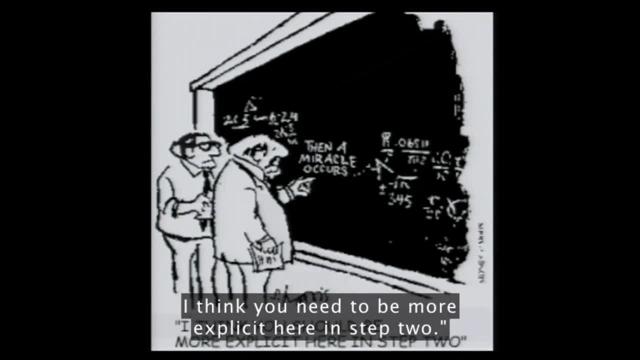 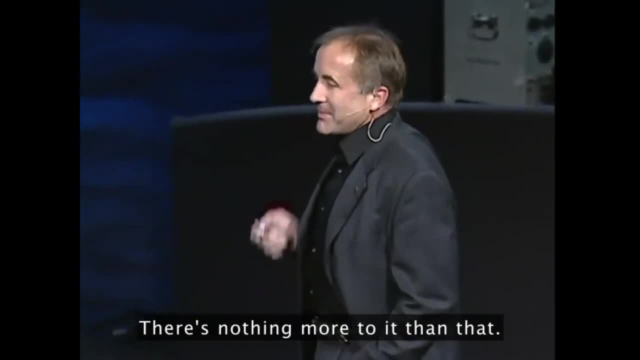 For those of you in the back. it says here: then a miracle occurs. I think you need to be more explicit here. in step two. This single slide completely dismantles the intelligent design arguments. There's nothing more to it than that You can say a miracle occurs. 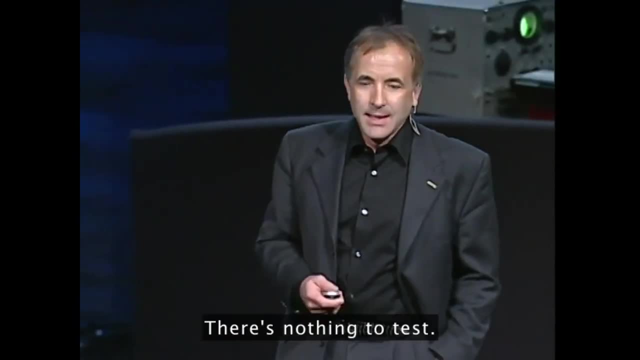 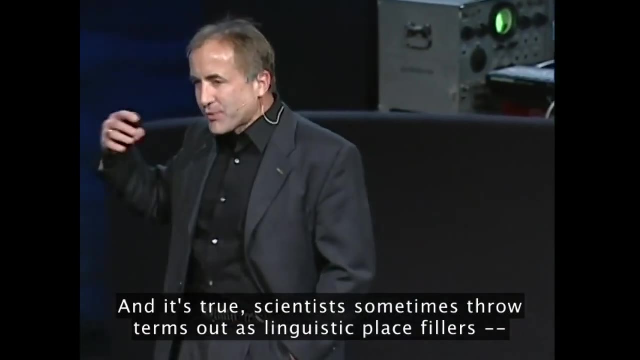 It's just that it doesn't explain anything, It doesn't offer anything, It doesn't test. It's the end of the conversation for intelligent design creationists- And it's true, Scientists sometimes throw terms out as linguistic place fillers, dark energy or dark matter or something like that. 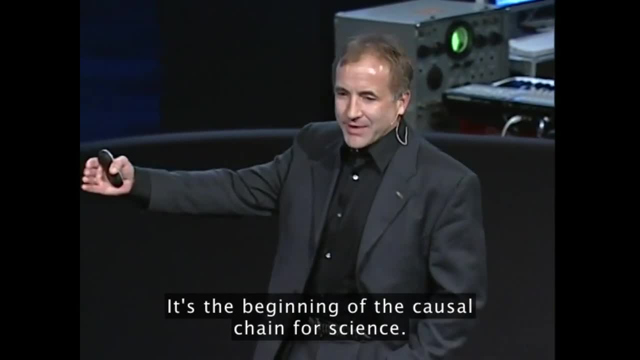 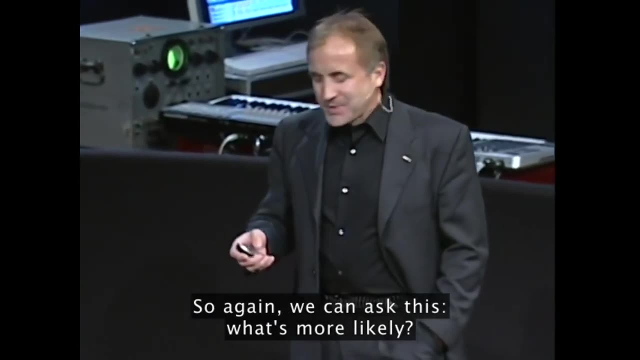 until we figure out what it is, We'll just call it this: It's the beginning of the causal chain. for science, For intelligent design, creationists, it's the end of the chain. So again we can ask this: what's more likely? 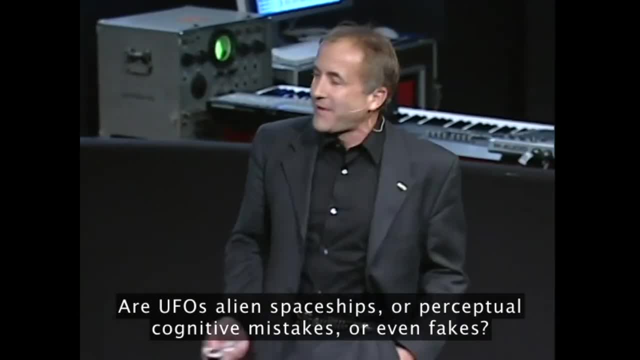 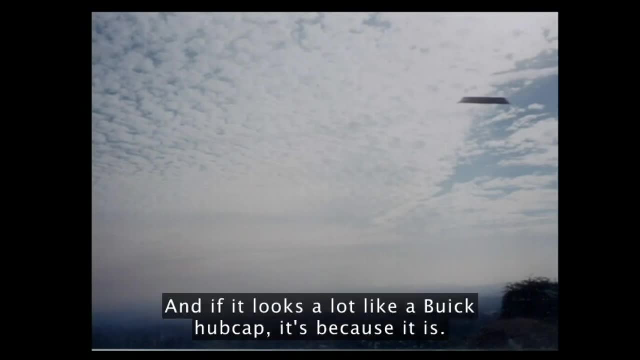 Are UFOs, alien spaceships or perceptual cognitive mistakes or even fakes? This is a UFO. This is from my house in Altadena, California, looking down over Pasadena, And if it looks a lot like a Buick hubcap, it's because it is. 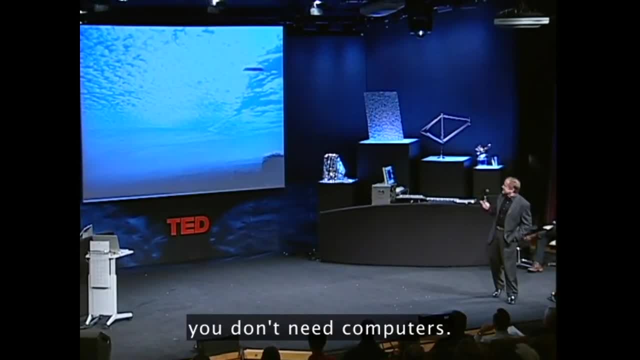 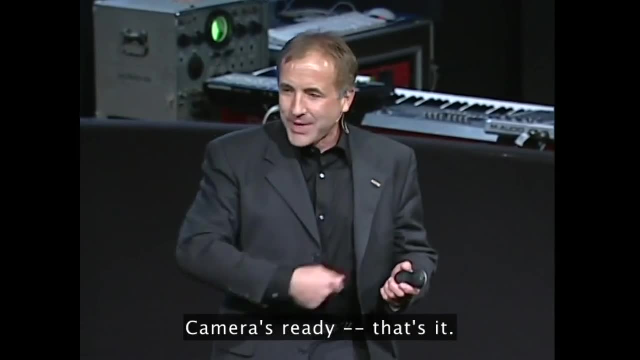 You don't even need Photoshop, You don't need high-tech equipment, You don't need computers. This was shot with a throwaway Kodak Instamatic camera. You just have somebody off on the side with a hubcap ready to go. camera's ready. 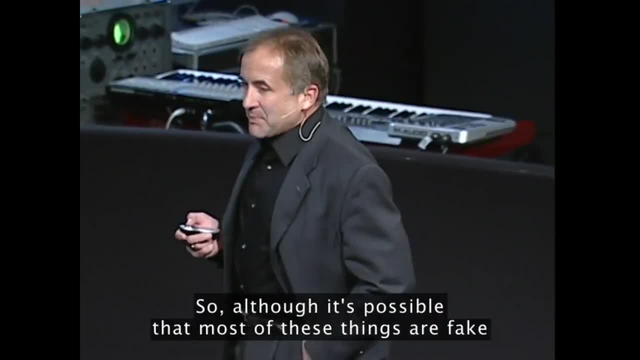 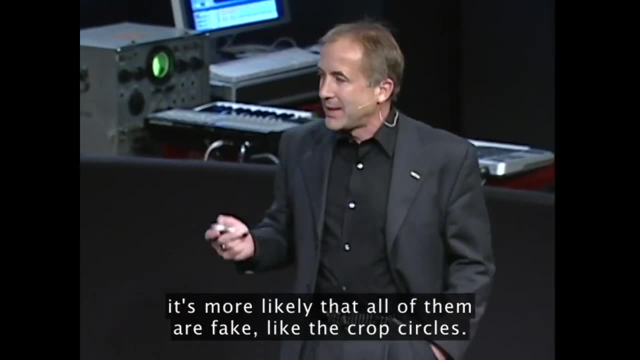 That's it. So, although it's possible that most of these things are fake or illusions or so on, and that some of them are real, it's more likely that all of them are fake, like the crop circles. On a more serious note, in all of science, 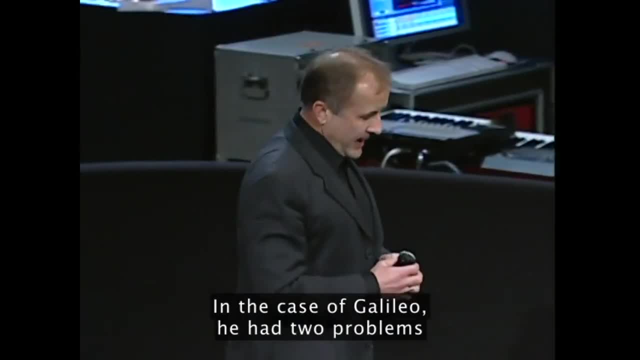 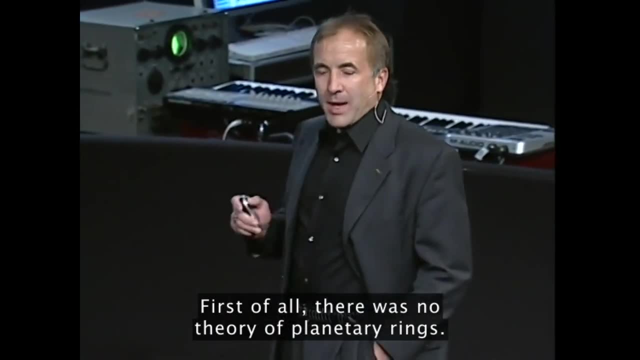 we're looking for a balance between data and theory. In the case of Galileo, he had two problems when he turned his telescope to Saturn. First of all, there was no theory of planetary rings And, second of all, his data was grainy and fuzzy. 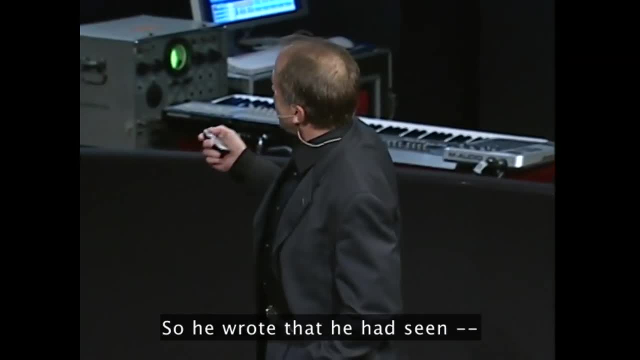 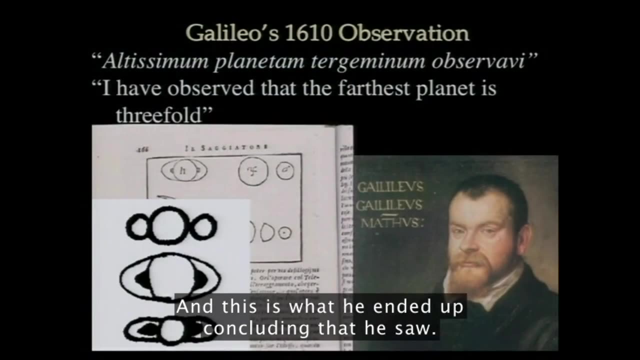 and he couldn't quite make out what it was he was looking at. So he wrote that he has seen, I have observed that the furthest planet has three bodies, And this is what he ended up, concluding that he saw. So, without a theory of planetary rings and with only grainy data, 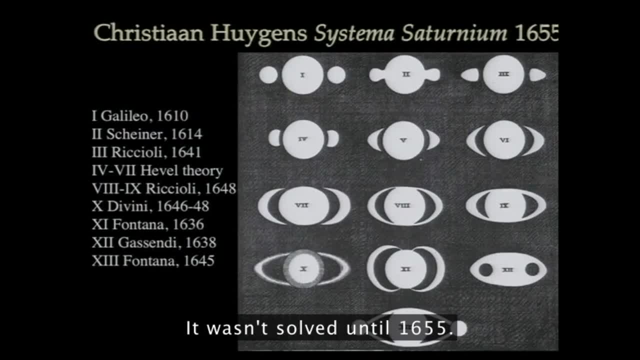 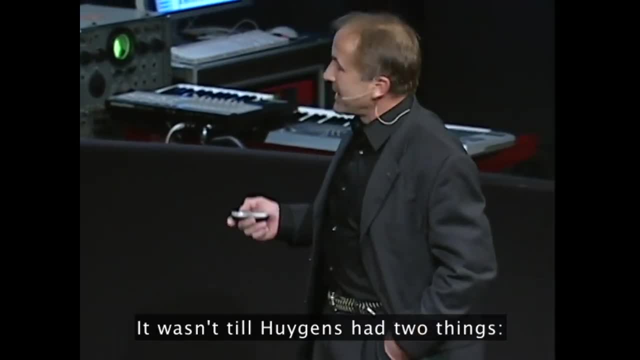 you can't have a good theory, And it wasn't solved until 1655.. This is Christian Huygens' book, in which he catalogued all the mistakes that people made in trying to figure out what was going on with Saturn. It wasn't until Huygens had two things. 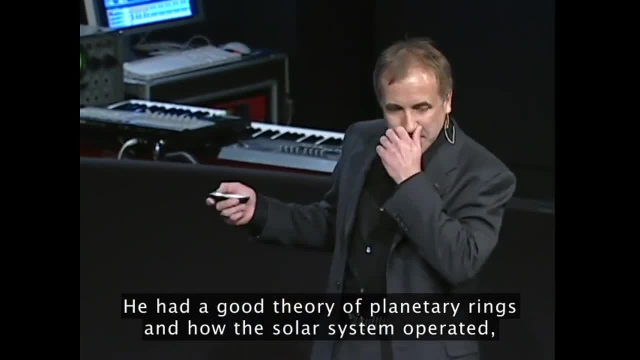 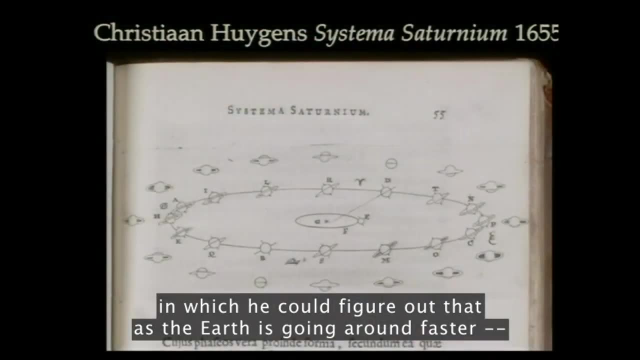 He had a good theory of planetary rings and how the solar system operated, and then he had better telescopic, more fine-grained data in which he could figure out that, as the Earth is going around faster, according to Kepler's laws, than Saturn, 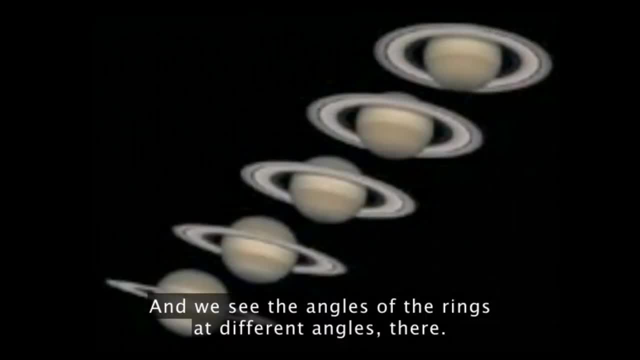 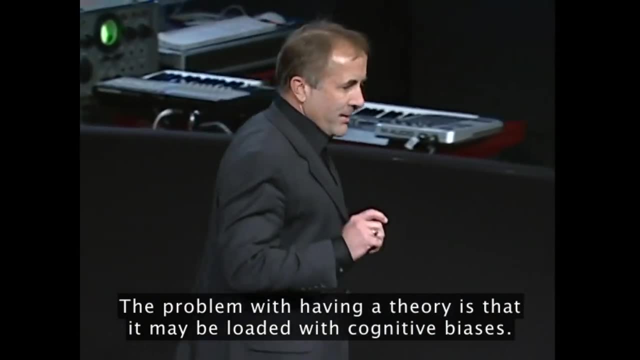 we catch up with it and we see the angles of the rings at different angles there, And that in fact turns out to be true. The problems with having a theory is that your theory may be loaded with cognitive biases. So one of the problems of explaining why people believe weird things. 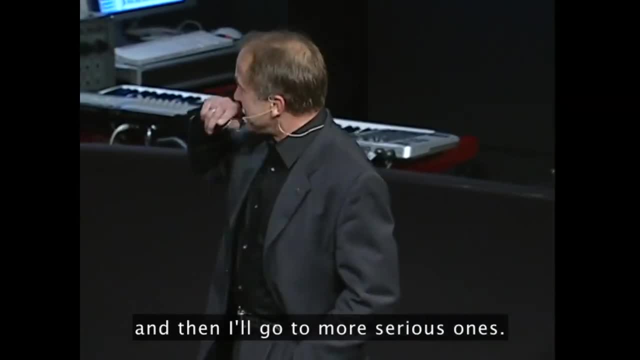 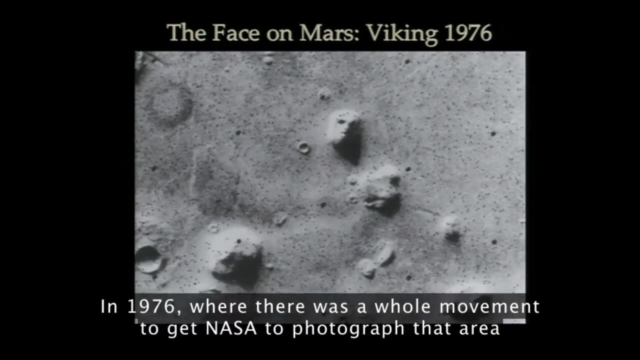 is that we have things on a simple level and then I'll go to more serious ones. like we have a tendency to see faces, This is the face on Mars which was in 1976. So there was a whole movement to get NASA to photograph that area. 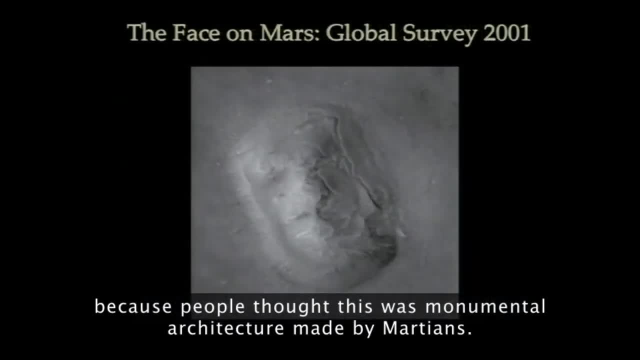 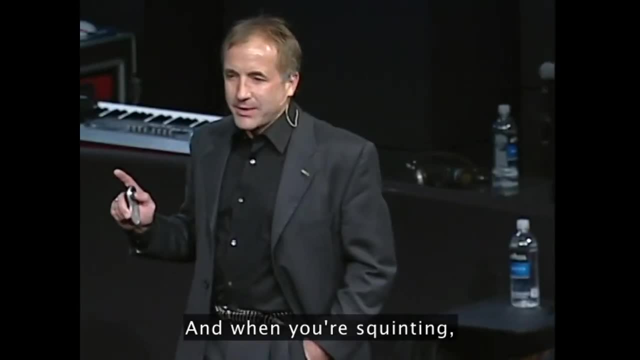 because people thought this was monumental architecture Made by Martians. Well, it turns out. here's the close-up of it from 2001.. If you squint, you can still see the face, And when you're squinting, what you're doing is you're turning that. 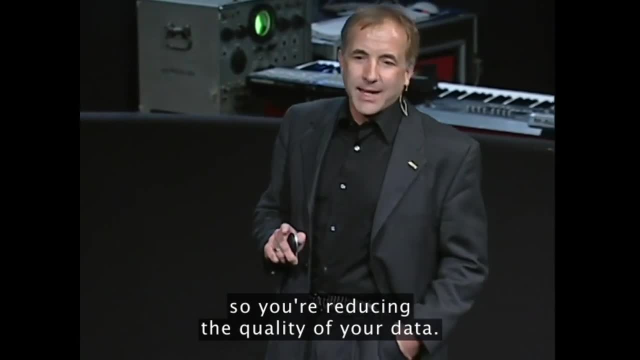 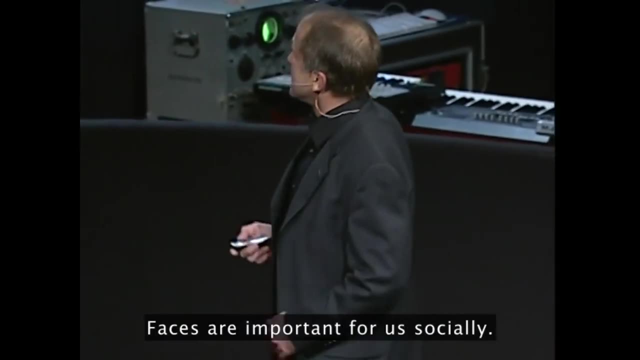 from fine grain to coarse grain, And so you're reducing the quality of your data. And if I didn't tell you what to look for, you'd still see the face, because we're programmed by evolution to see faces. Faces are important for us socially. 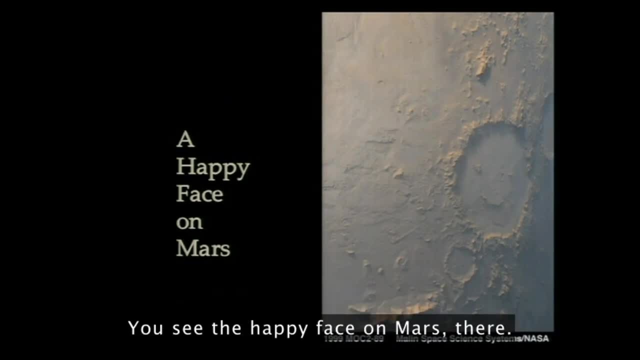 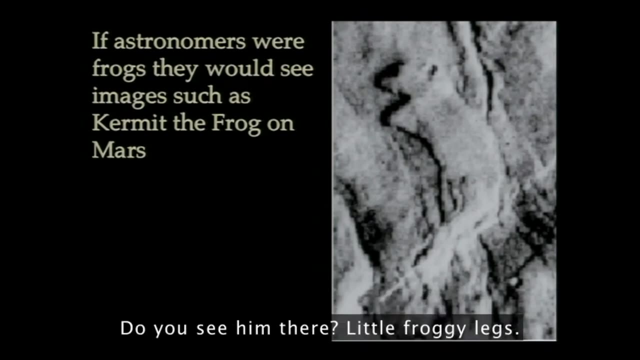 And, of course, happy faces. Faces of all kinds are easy to see. You can see the happy face on Mars there. If astronomers were frogs, perhaps they'd see Kermit the Frog. Do you see him there, Little froggy legs? 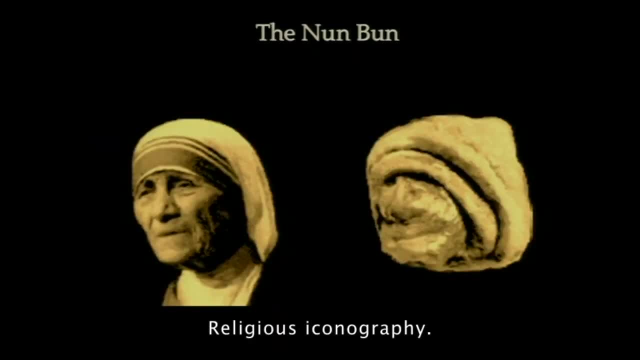 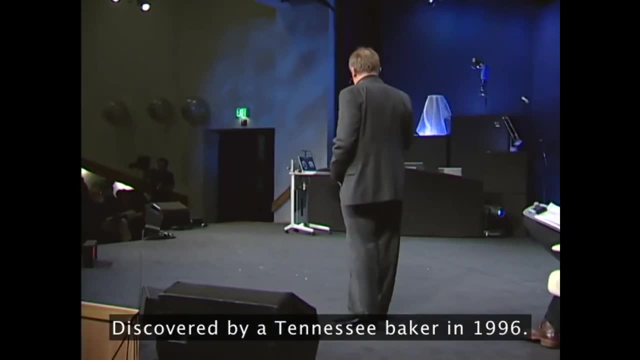 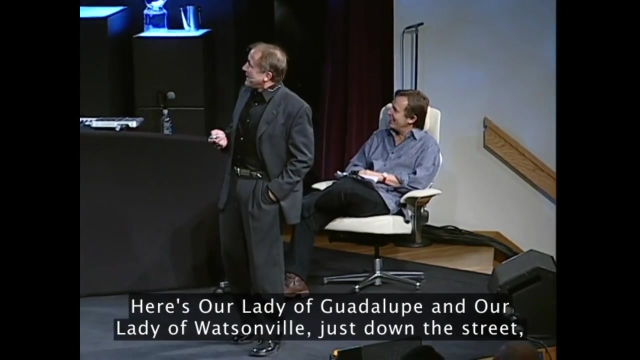 Or if geologists were elephants: Religious iconography discovered by a Tennessee baker in 1996.. He charged five bucks a head to come see the nun bun until he got a cease and desist from Mother Teresa's lawyer. Here's Our Lady of Guadalupe and Our Lady of Watsonville. 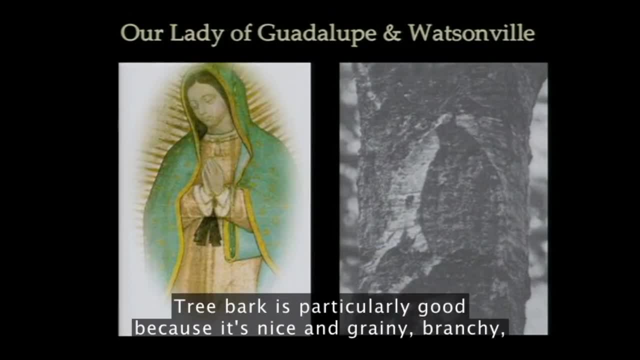 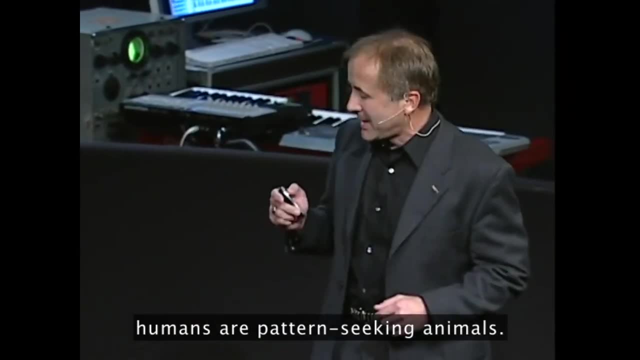 just down the street or is it up the street from here? Tree bark is particularly good because it's nice and grainy, branchy, black and white, It's splotchy and you can get the pattern-seeking humans are pattern-seeking animals. 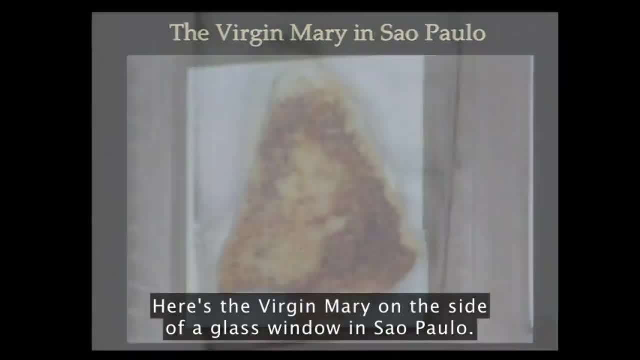 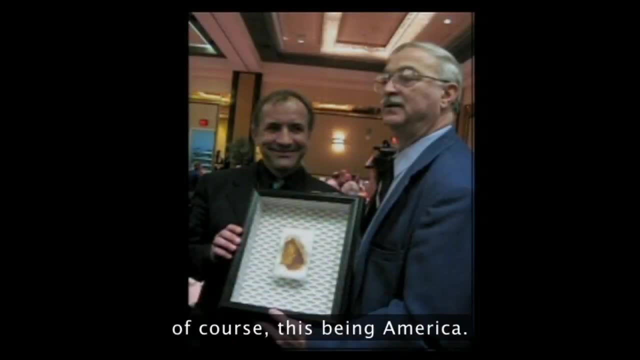 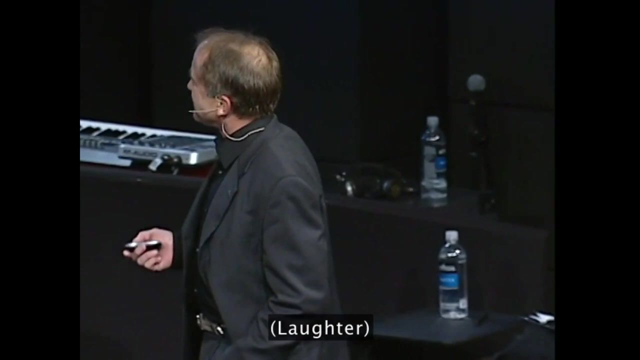 Here's the Virgin Mary on the side of a glass window in Sao Paulo. Here's the Virgin Mary made her appearance on a cheese sandwich which I got to actually hold in a Las Vegas casino. Of course this would be in America. This casino paid $28,500 on eBay for the cheese sandwich. 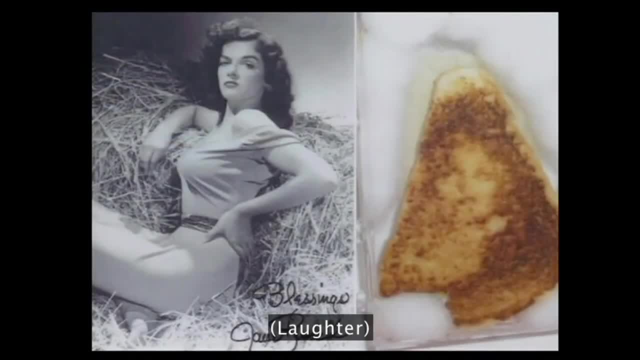 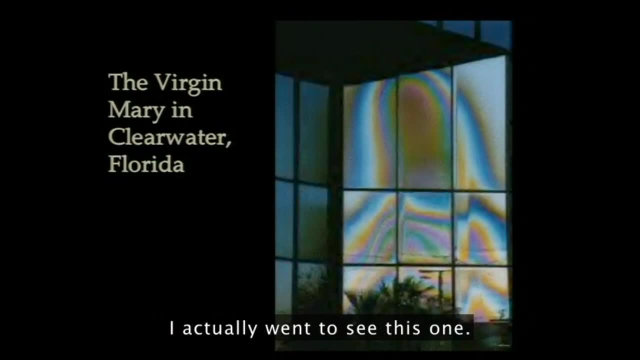 But who does it really look like? The Virgin Mary Has that sort of puckered lips, 1940s-era look. Virgin Mary in Clearwater, Florida, I actually went to see this one. There was a lot of people there, of the faithful come to be in their wheelchairs. 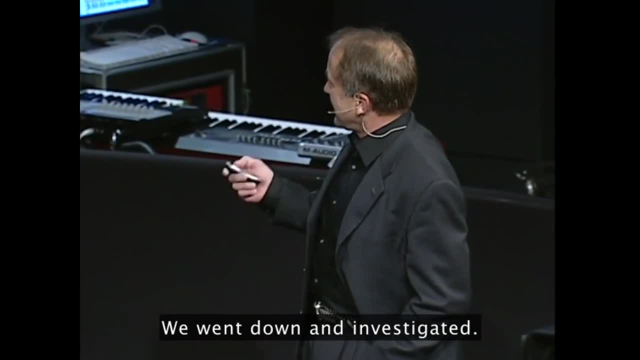 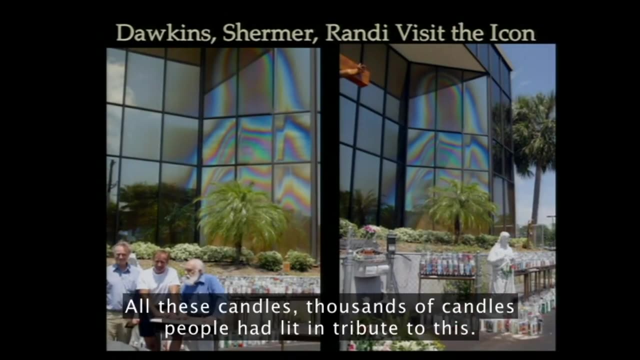 and crutches and so on, and we went down and investigated. Just to give you a size, that's Dawkins, me and the amazing Randy next to this, two two-and-a-half-story size image. All these candles, so many thousands of candles people had lit in tribute to this. 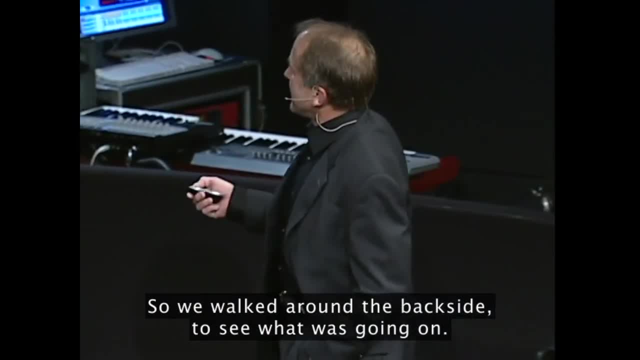 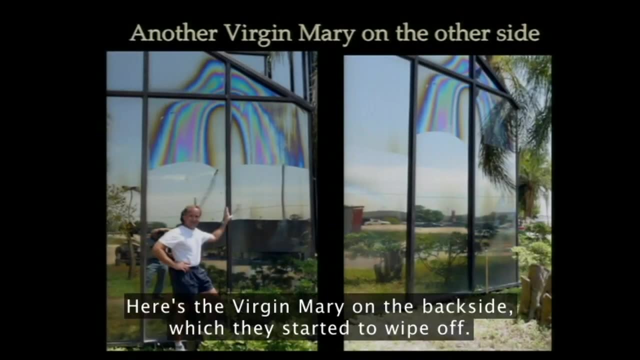 So we walked around the backside just to see what was going on. here, It turns out, wherever there's a sprinkler head and a palm tree, you get the effect. Here's the Virgin Mary on the backside, which they started to wipe off. 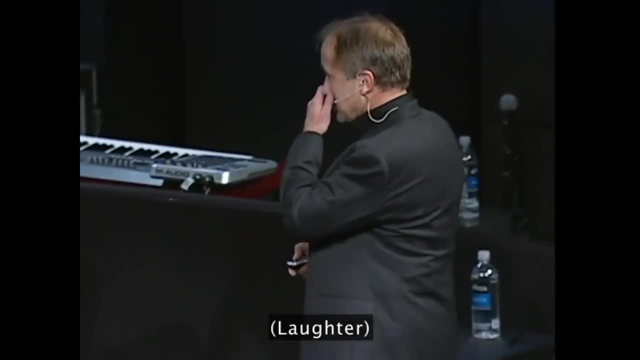 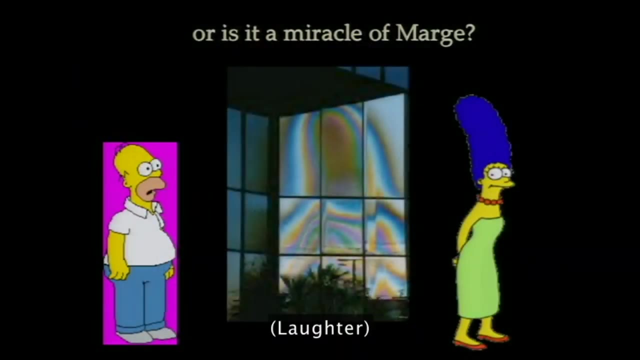 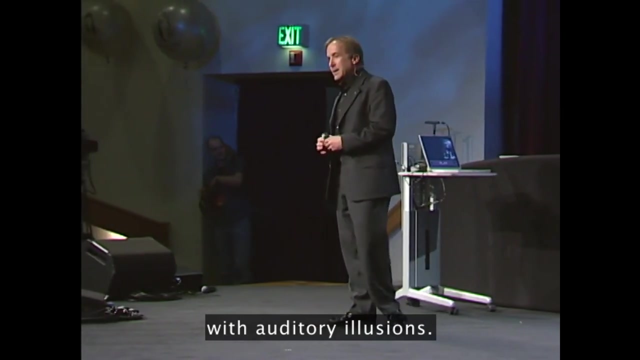 I guess you can only have one miracle per building. So is it really a miracle of Mary or is it a miracle of Marge? And then I'm going to finish up with another example of this with auditory illusions. There's this film, White Noise, with Michael Keaton, about the dead talking back to us. 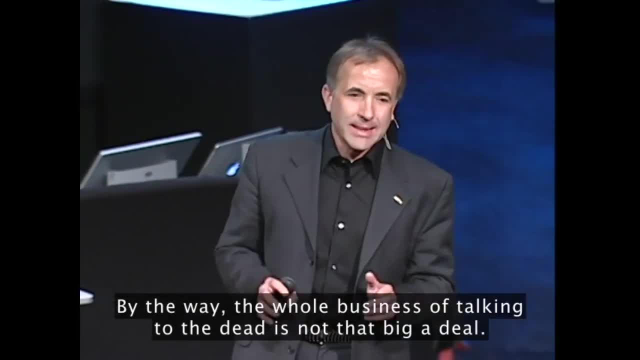 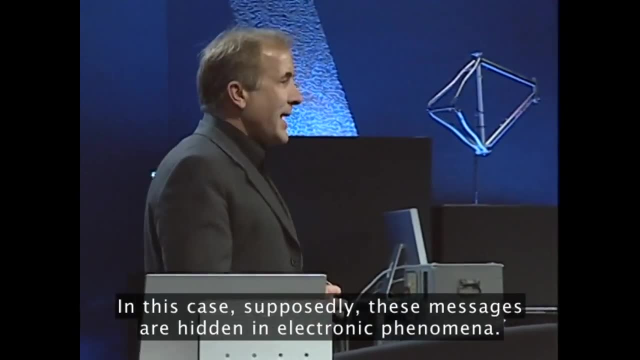 By the way, this whole business of talking to the dead, it's not that big a deal anymore. Nobody can do it. It turns out it's getting the dead to talk back. That's the really hard part In this case. supposedly, these messages are hidden in electronic phenomena. 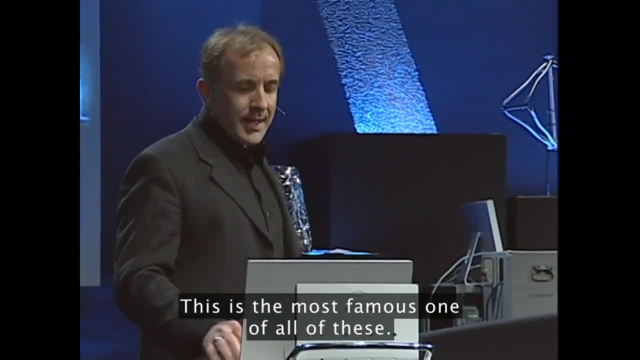 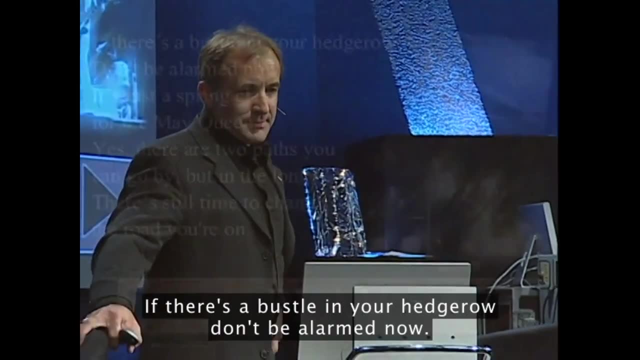 There's a reversespeechcom web page in which I downloaded this stuff. Here is the forward. This is the most famous one of all of these. Here's the forward version of the very famous song. If there's a bustle in your hedgehog, don't be alarmed. 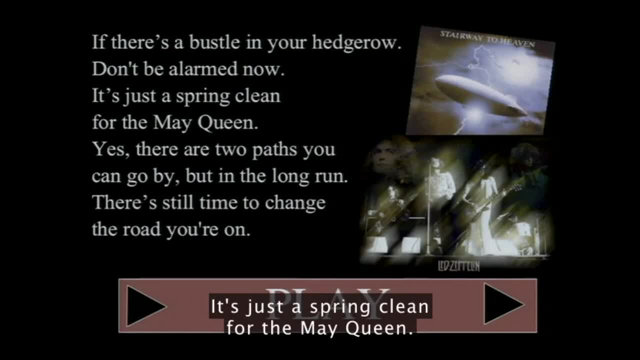 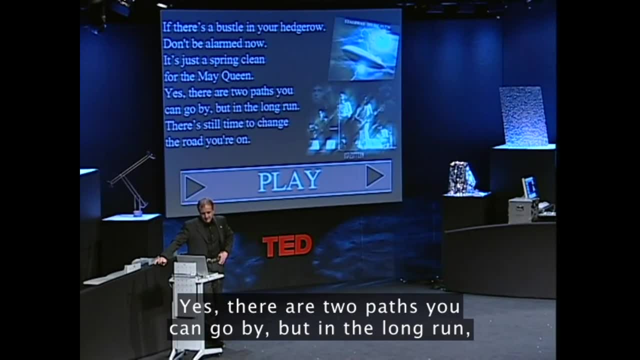 It's just a sprinkler for the making queen. Yes, there are two paths you can go by, But in the long run there's still time to change the road you're on. Boy, can you just listen to that all day? 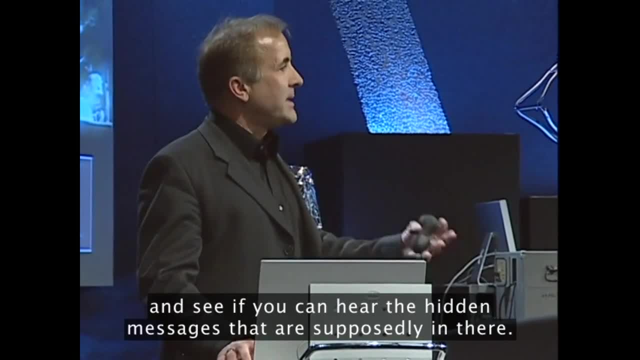 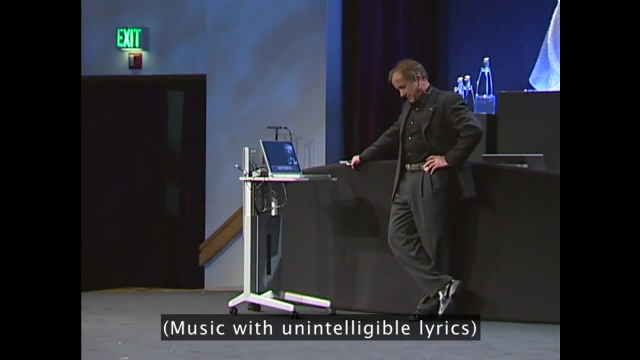 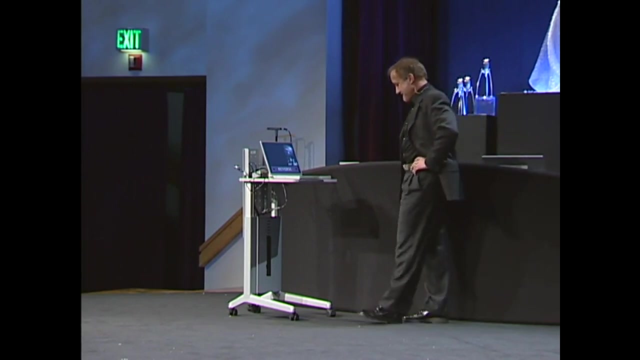 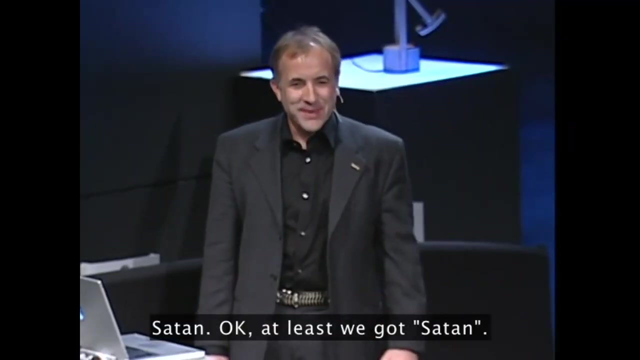 All right, here it is backwards and see if you can hear the hidden messages that are supposedly in there. What did you get? Satan. Okay, at least we got Satan. Now I will prime your auditory part of your brain to tell you what you're supposed to hear. 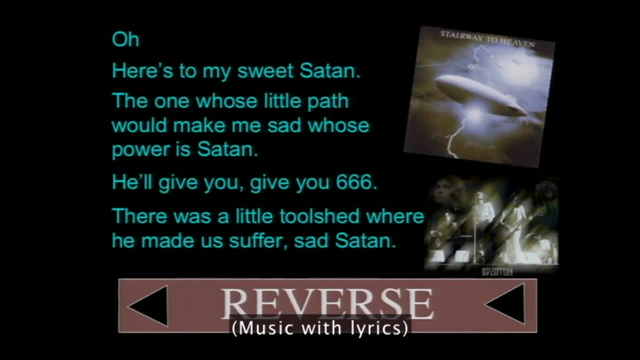 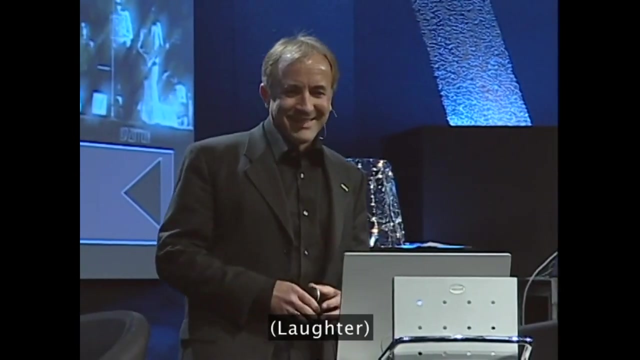 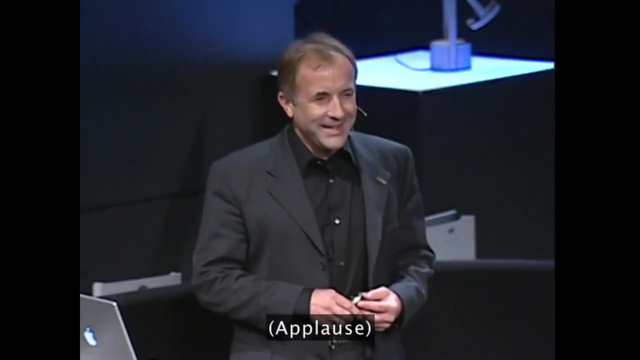 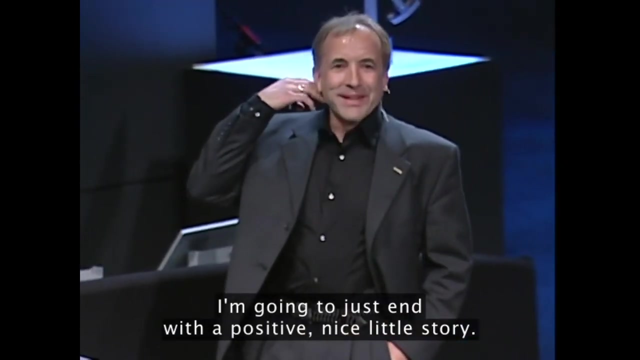 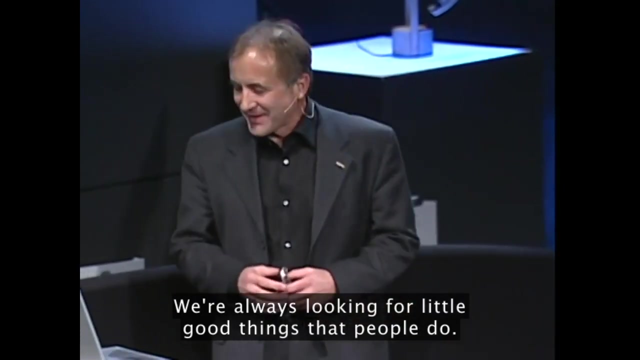 And then hear it again. You can't miss it when I tell you what's there. All right, I'm going to just end with a positive. a nice little story about the Skeptics is a nonprofit educational organization. We're always looking for little good things that people do. 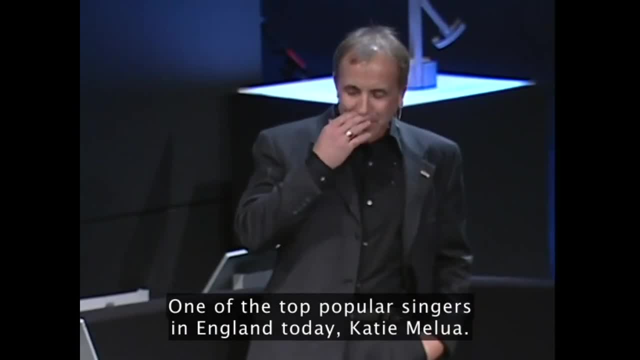 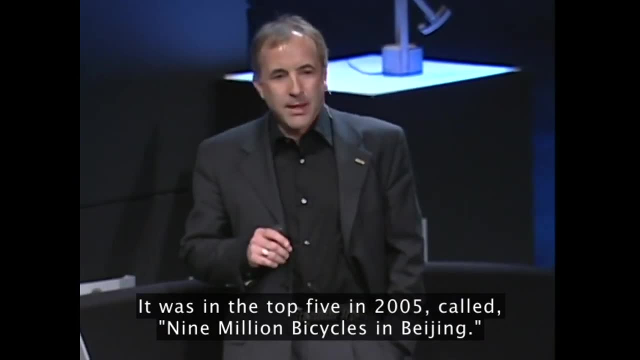 In England. there's a pop singer, one of the top popular singers in England today, Katie Malua, And she wrote a beautiful song. It was in top five in 2005, called 9 Million Bicycles in Beijing. It's a love story. 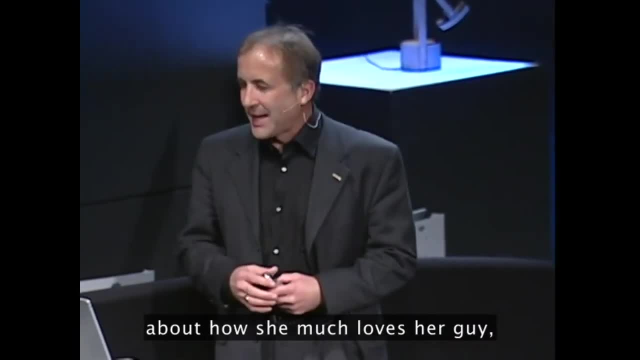 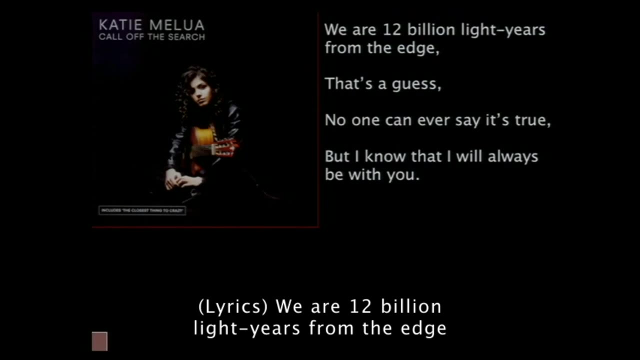 She's sort of the Nora Jones of the UK about how much she loves her guy and compared to 9 million bicycles and so forth, And she has this one passage here. We are 12 billion light years from the edge. That's a guess. 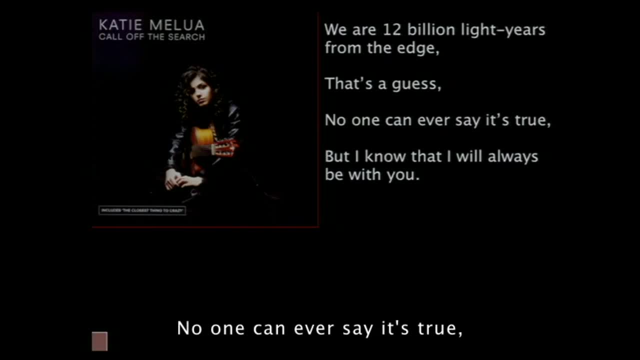 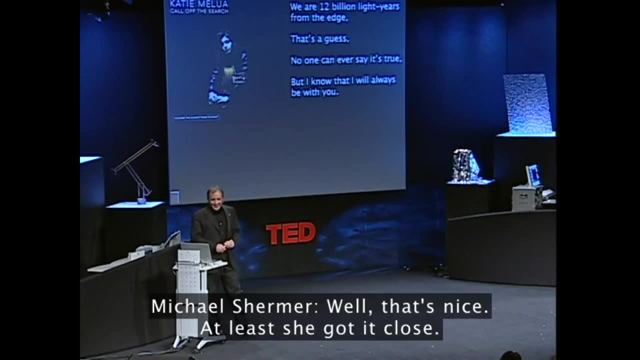 No one can ever say it's true, But I know that I will always be with you. Well, that's nice. At least she got it close. In America it would be. we're 6,000 light years from the edge. 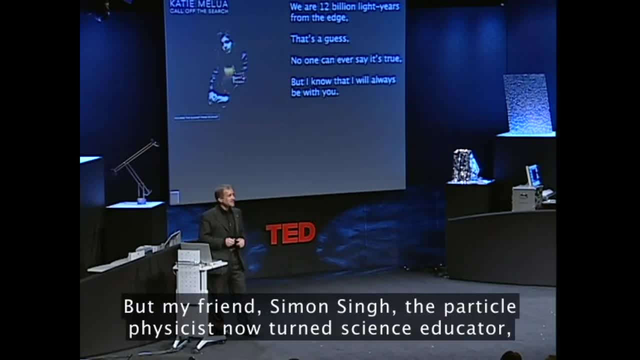 But my friend Simon Singh, the particle physicist now turned science educator, and he wrote the book The Big Bang and so on- uses every chance he gets to promote good science, And so he wrote an op-ed piece in The Guardian about Katie's song in which he said: well, we know exactly how far from the edge. 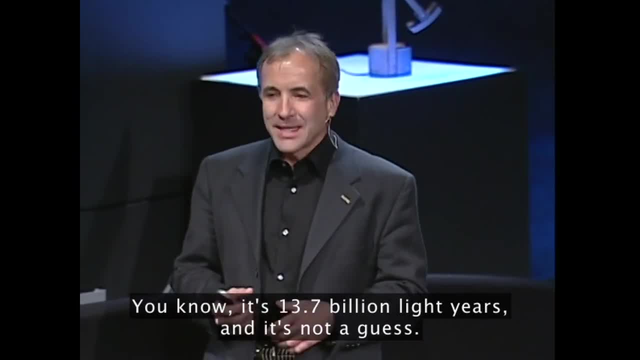 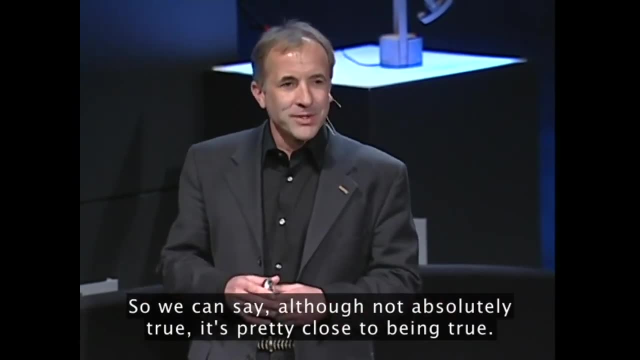 You know it's 13.7 billion light years, And it's not a guess. We know within a precise error bars there how close it is, And so we can say, although not absolutely true, that it's pretty close to being true. 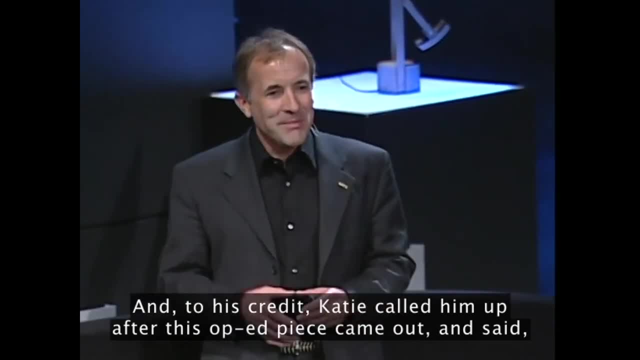 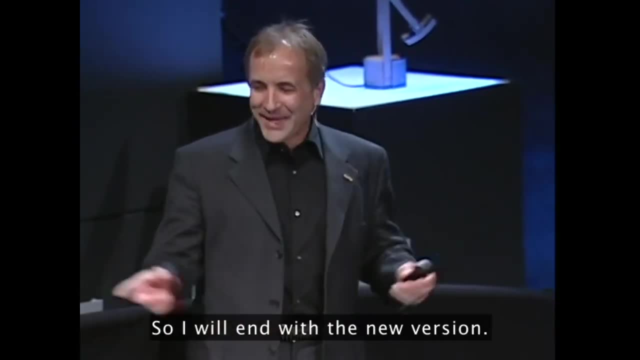 And, to his credit, Katie called him up after this op-ed piece came out and said: I'm so embarrassed, I was a member of the astronomy club and I should have known better. And she recut the song. So I will end with the new version. 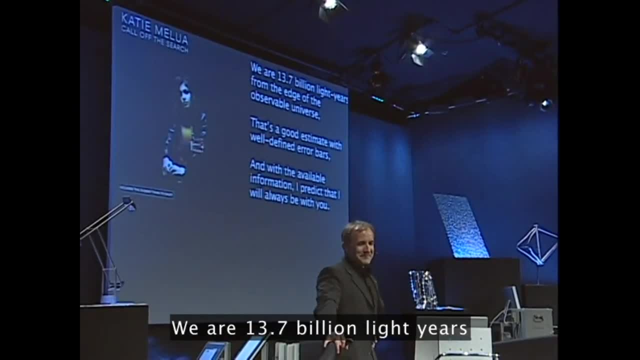 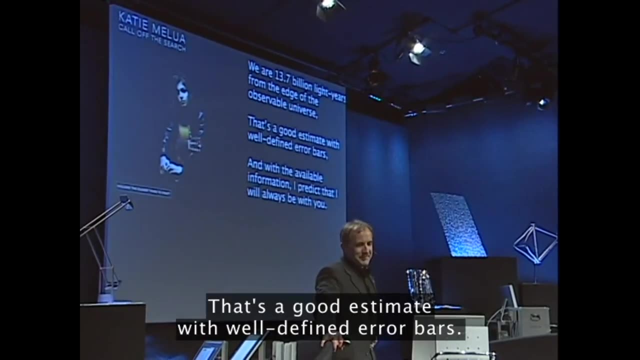 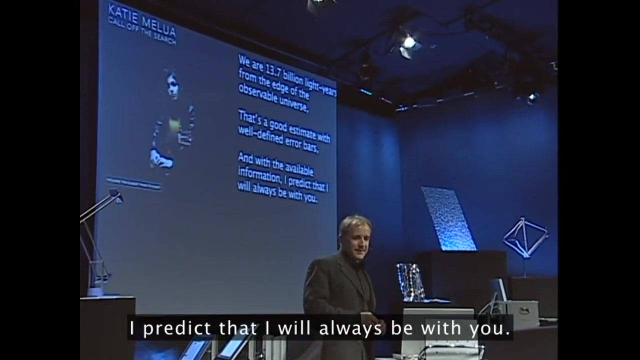 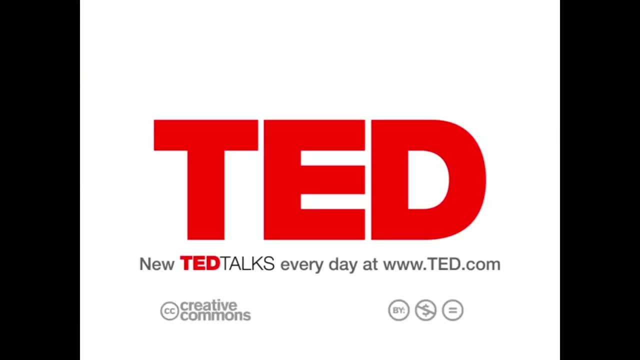 We are 13.7 billion light years from the edge of the observable universe. That's a good estimate, with well-defined error bars And with the available information, I predict that I will always be with you. How cool is that? 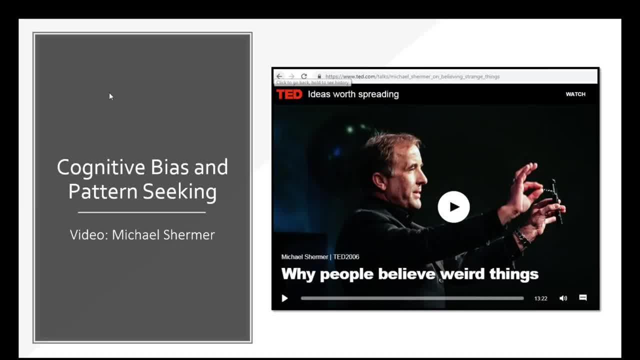 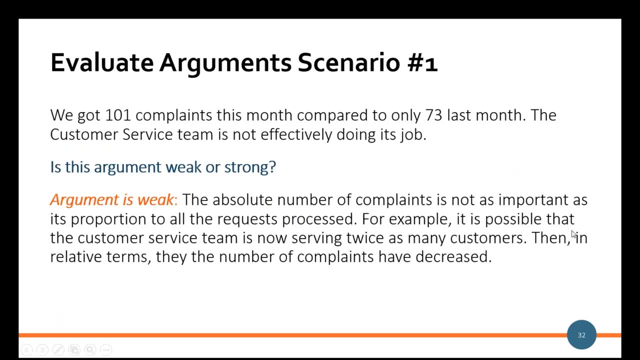 One way to talk a little bit about the role of cognitive biases, how they impact our judgment, the way in which we look at information and the importance of critical thinking, the importance of being skeptical and really looking at information overall. I'm going to skip these next couple of slides. 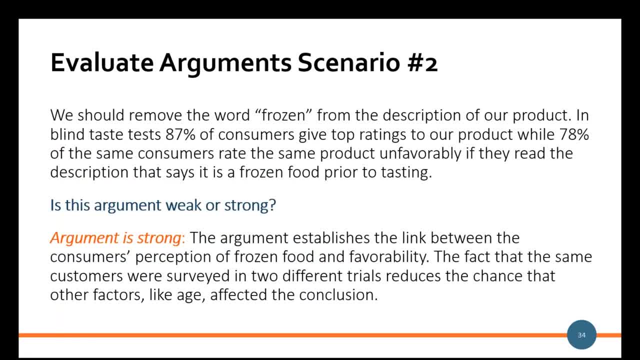 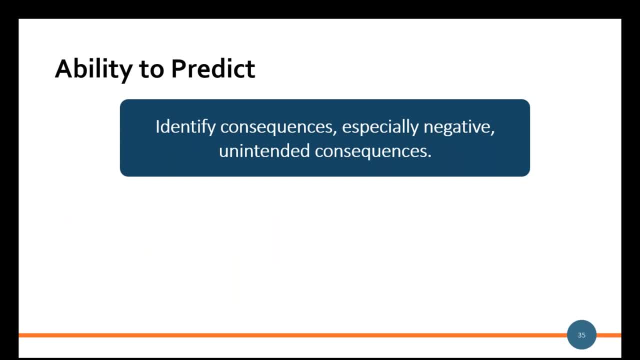 I'm going to try to okay, All right. So the third area is around the ability to predict, And this is about identifying consequences, especially looking at the unintended consequences or the potentially negative consequences of your action overall. Sorry, there's a little delay in the 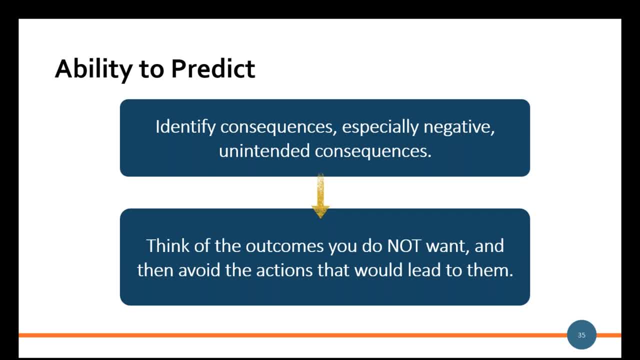 So the third area is to think about the outcome, but not the ones you want, Rather to think a little bit about the possible potential problems that might be out there overall, And that is really the focus. We tend to focus on what we want rather than what might be or what could happen. 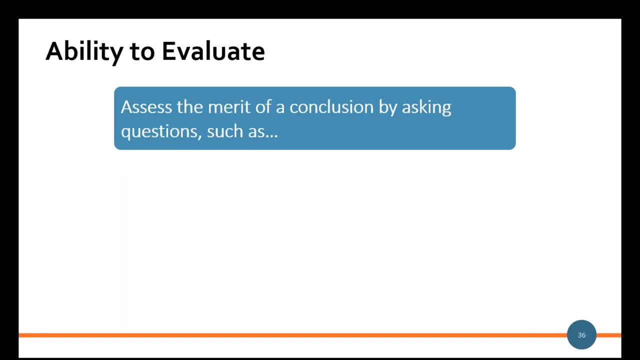 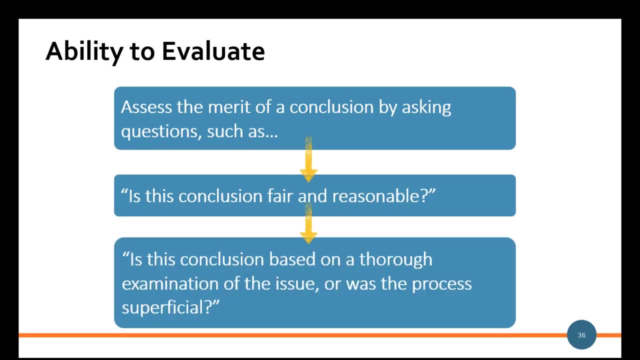 And the last is the ability to evaluate overall. This is around assessing the merit of a conclusion that you're making overall And what you're trying to do is think about. does it follow from the data I have? Is the conclusion fair and reasonable? 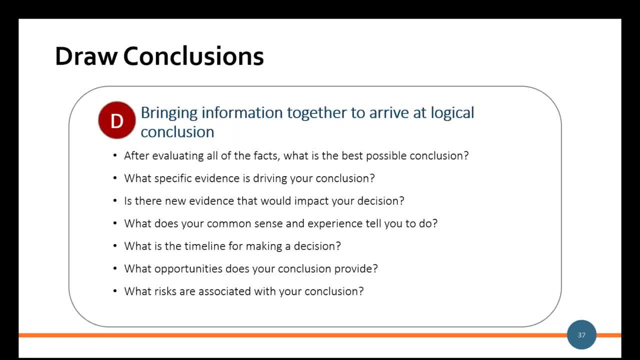 And, based on the information I have, does it make sense overall- And here are a couple of questions that you can ask yourself to basically help you determine if your conclusions are following the information that you have- overall, After evaluating the facts, what's the best possible outcome? 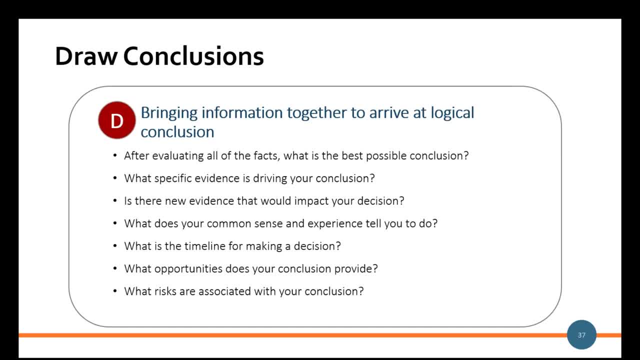 What specific evidence do I have that's driving my conclusion? Is there new evidence that I should be thinking about? What does your common sense say overall? What's the timeline? What opportunities does your conclusion provide? And by being specific and asking yourself these questions, you can make it part of your thought process overall. 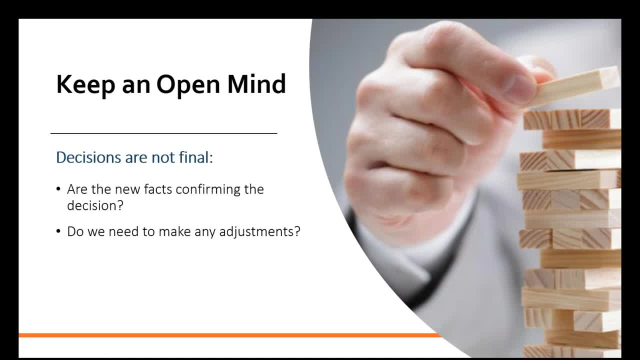 The important thing to remember, I think, around critical thinking, is that decisions should not be fixed, Decisions should not be seen as final. You really need to be open to new facts, new information that may give you a different point of view on things and may cause you to make a few adjustments overall. 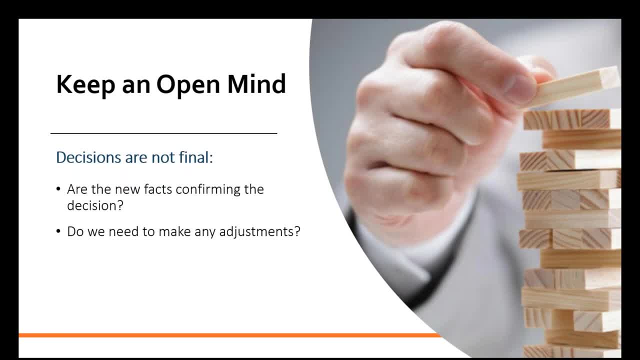 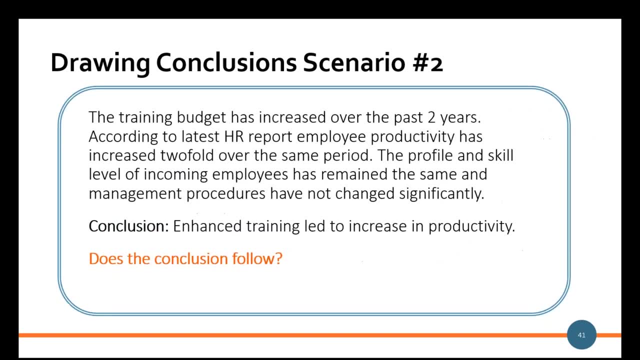 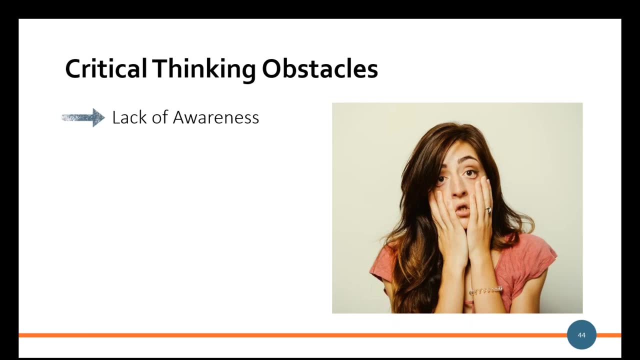 What you're trying to do is not avoid or ignore new information just because you've made a commitment to a particular point of view. All right, Let's just move ahead a little bit on this. So, in terms of some of the obstacles around critical thinking, one of them is a general lack of awareness. 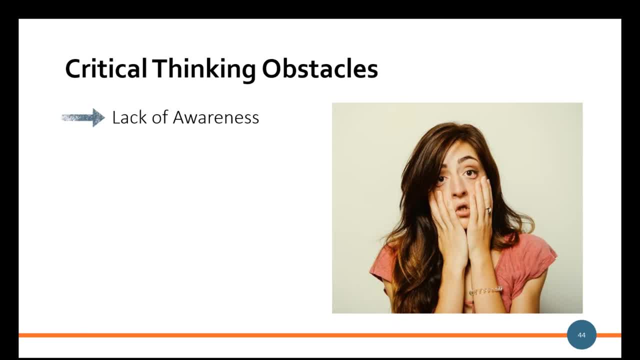 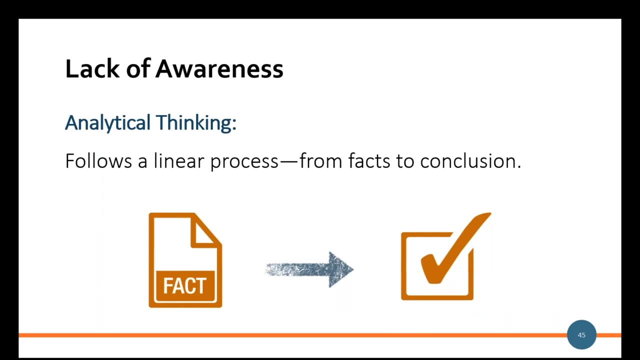 And, in general, that's what we've been talking about: being introspective, understanding your own biases, understanding what some of the key questions are. Being a little bit skeptical is a key component of being a critical thinker and a key obstacle. So let's take a look at each one of those. 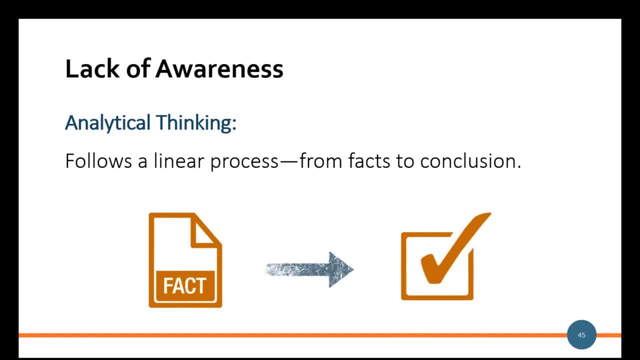 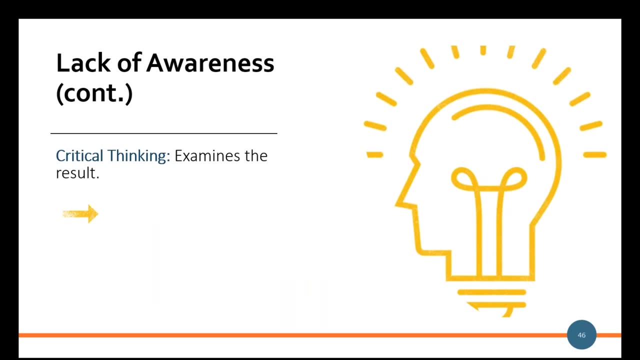 In terms of the lack of awareness, one solution is to follow a linear process, to use a structured process around collecting information, assessing the information and drawing a conclusion which will help in terms of addressing that awareness piece. So you want to, overall, be in a critical thinking. 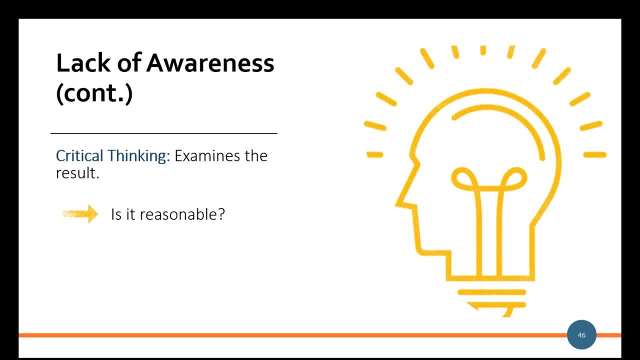 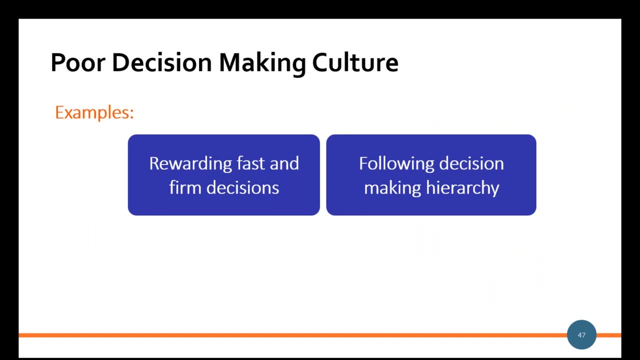 Take a look at the results and basically ask: is it reasonable, What are the overall implications And what decisions and actions will you take now going forward? right, A poor decision-making culture here is around, a culture that rewards speed and fast decisions. 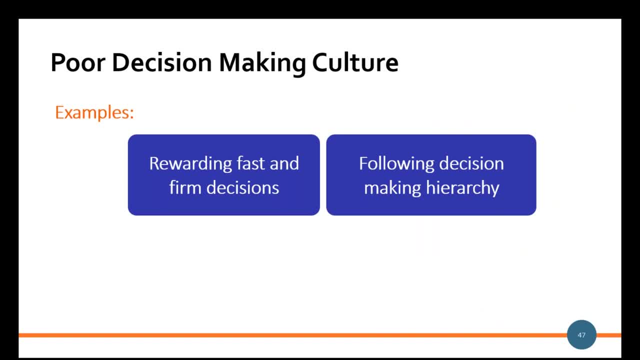 And when people do critical thinking, self-assessment, one of the things that causes problems is not that they're not good critical thinkers. Many people are excellent critical thinkers. But when you rush the test or when you get interrupted during the test, it tends to have a negative impact on your scores, on the outcome. 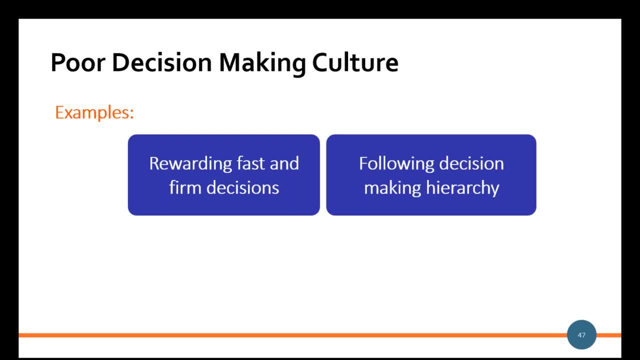 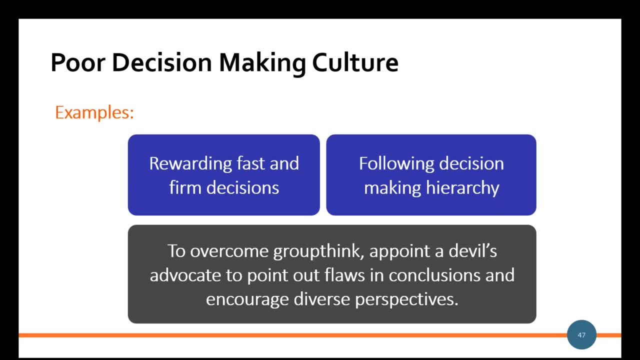 So this idea of speed does not always work in your favor overall, right? What you're trying to do also- and this goes back to that devil's advocate, that what-if question- avoiding group think, where the culture of group think is the most important thing. 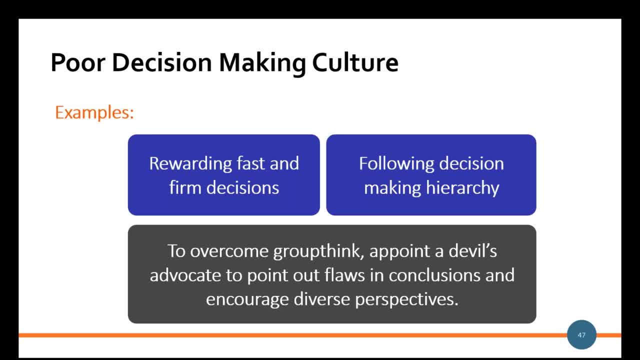 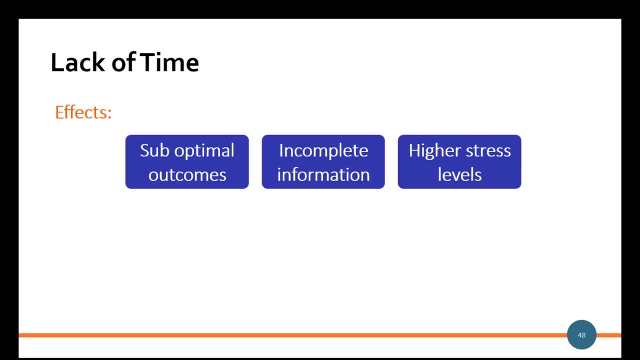 Where the culture of the organization is to go along with the group. That can be the death of critical thinking. where people don't express an alternate point of view, don't share additional information, don't ask difficult questions. overall, The lack of time, I think, is also interesting. 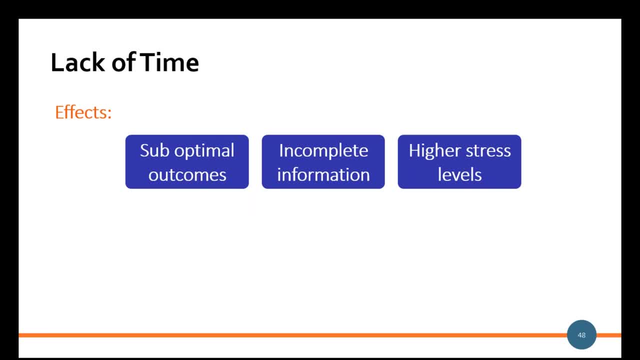 And again it goes back to the speed thing. It causes suboptimal decisions to be made Because you're not taking time to explore the relevant questions. You're not taking time to explore the relevant information. You're also working with incomplete information and higher stress levels. 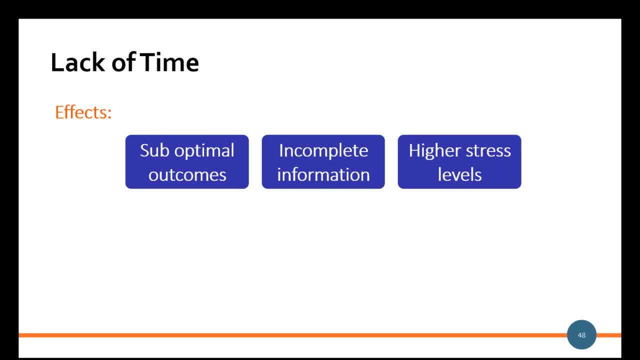 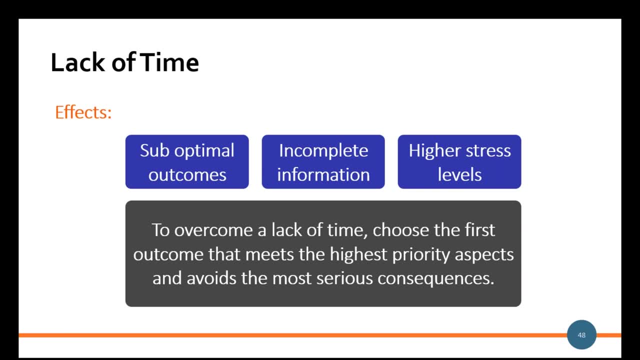 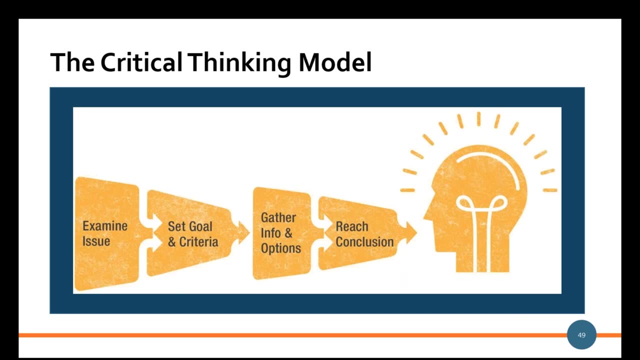 The key question here is what information is most relevant and how do you know that you have the right information. So a structured process can help with that overall and a critical thinking model. So the idea here is to start by examining the issue, Set out your decision criteria. 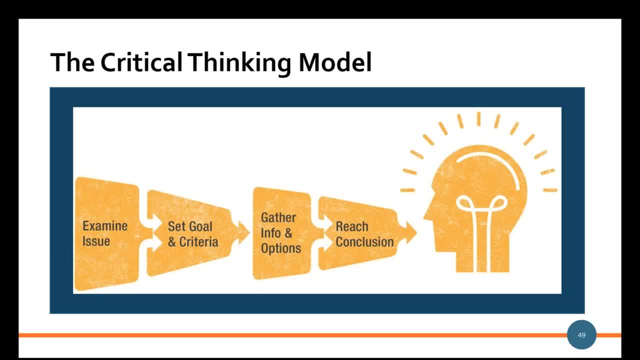 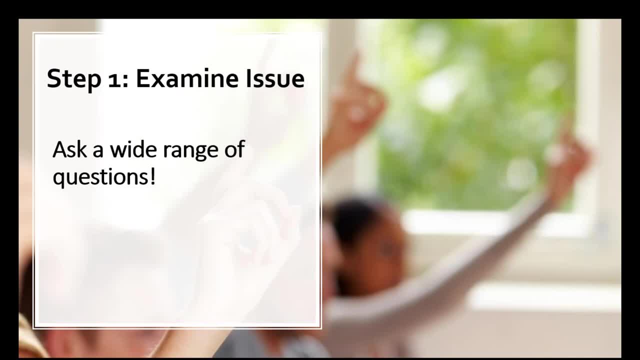 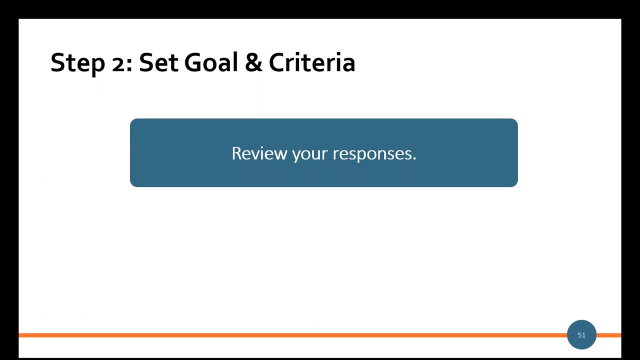 Your goal, Then gather that information related to your criteria and use that to reach a conclusion overall. Right, So you want to ask a wide range of questions when you're examining the issue overall, But the key is to set your goal or criteria, to be clear about what it is you'll use to make that decision overall. 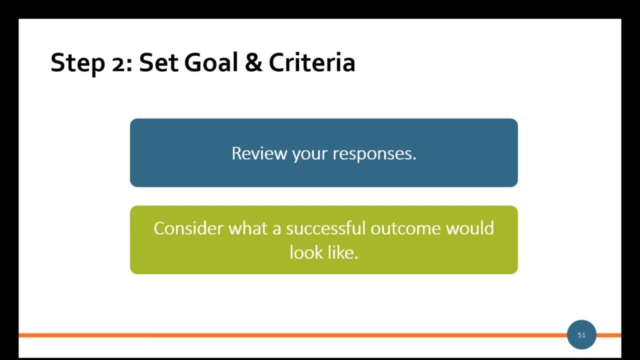 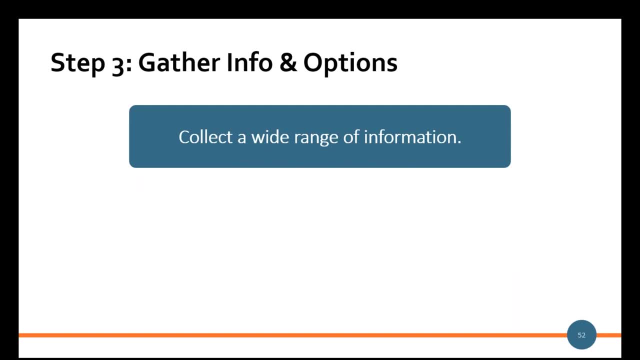 Right, Right. So you want to define what a successful outcome would look like before you start to look at information, And now you're at the data gathering stage And you want to collect a wide range of data, But you also can't go on an unlimited search for information as well. 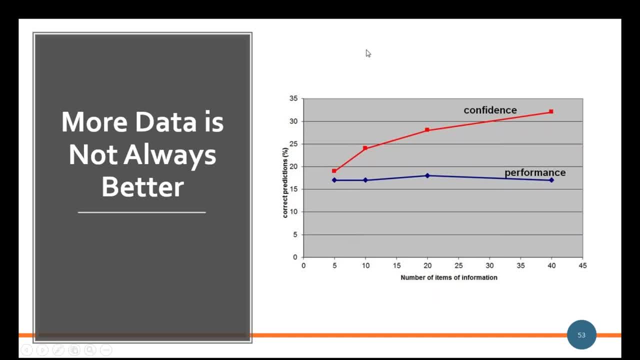 Right. So the key here is to be able to determine when enough data will help you make the best decision Right, And how do you have enough information? This chart shows the results of a study that was done, where they took a look at horse handicappers, race handicappers, people who bet on horses. 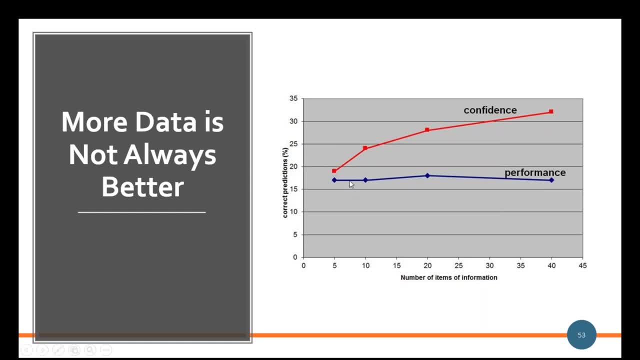 And you can see that the red line is the degree of confidence they had And the blue line is their performance. And you can see that as they were given more information, their confidence increased from there, But their performance did not improve at all. 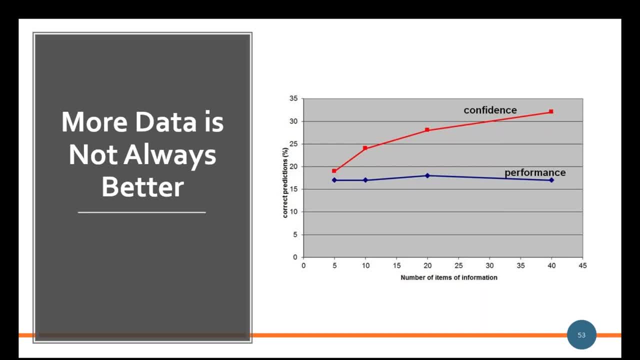 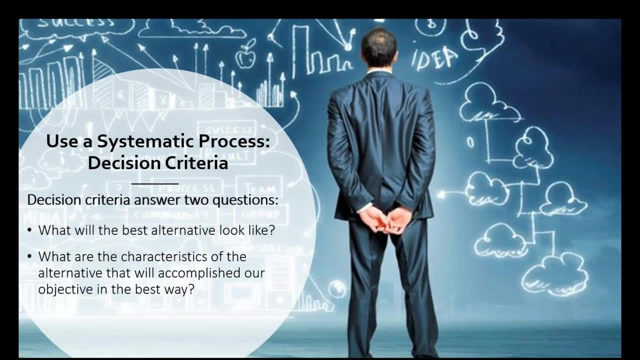 As a matter of fact, there's sort of an inflection point where you can see that their performance actually started to decrease as the information increased. So more information is not necessarily better. What you're looking for is the right information, Right? So how do you know when you have the right information? 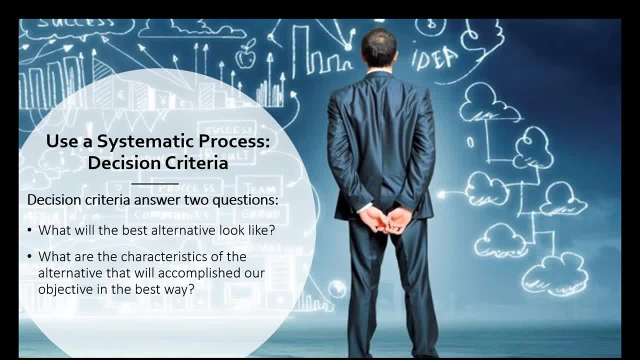 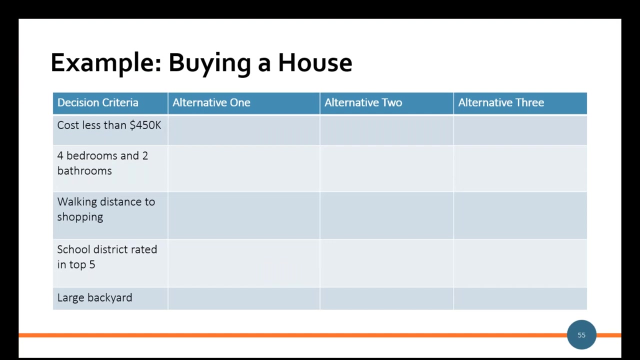 And the answer to that question is the systematic process and a decision criteria. A decision criteria answers two key questions: What will the best alternative look like And what are the characteristics of that alternative that will accomplish our objective in the best way? And here's an example of what a decision criteria might look like. 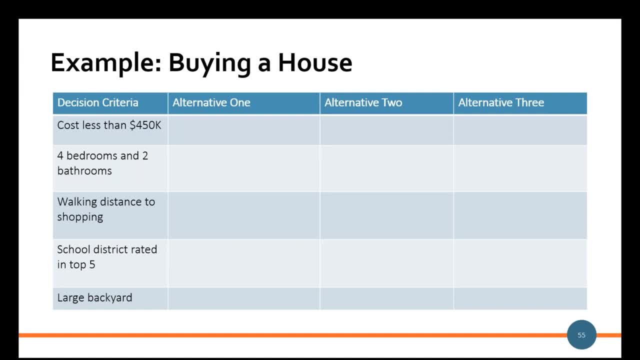 This example is around buying a house, which I think is something many of you know. I think it's something many of you have done, And here on the left is what you're laying out is the criteria that basically defines the best house for you. 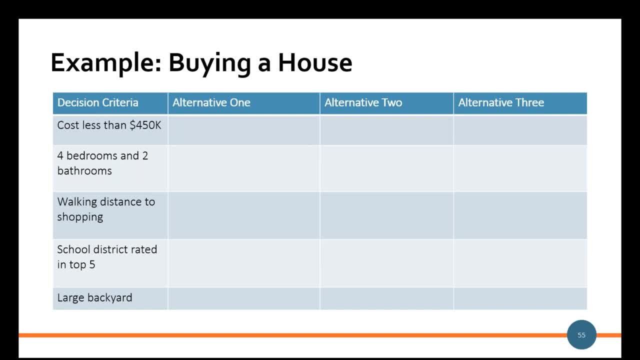 Right, And in theory, this is what you would give to the realtor And you'd say to them: only show me houses that meet this criteria. And then you take a look at two or three or more alternatives And now you're able to compare each alternative to that criteria. 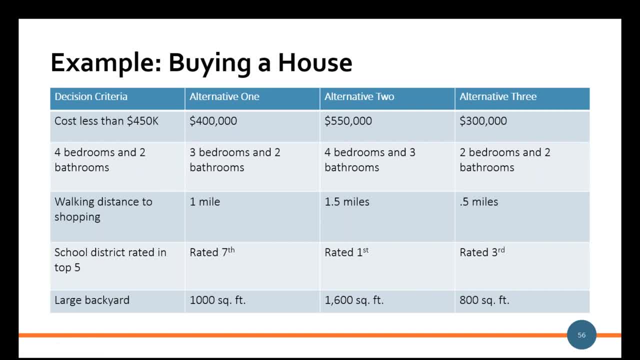 Right To see which alternative meets the criteria the best. The importance of this, or the usefulness of this, is you're defining what information is most relevant, what information is most useful, And now your search for information is in a more targeted kind of net. 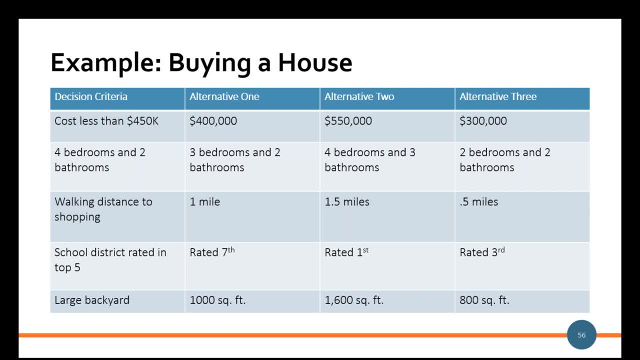 Rather than just looking at everything out there. that's possible. you're defining what's relevant and important If you can't fill in one of these little matrix squares. your search for information is also more targeted in general, because you're focused on a particular criteria. 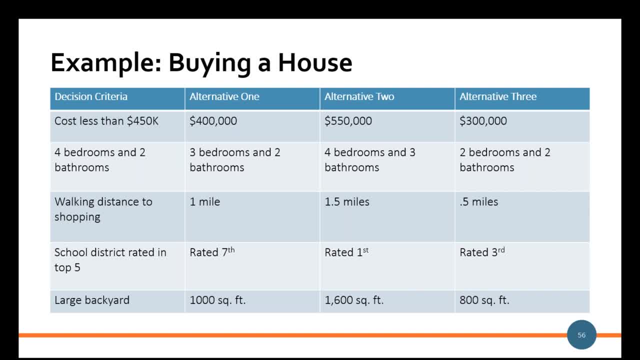 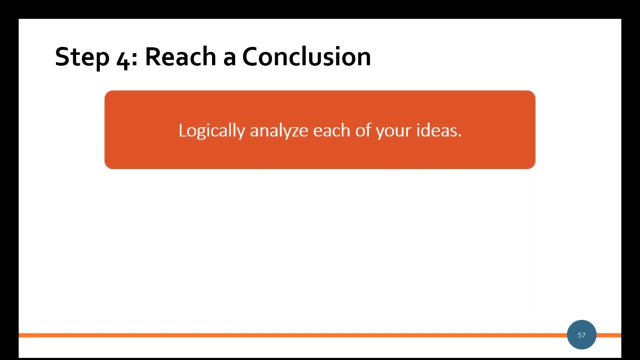 In addition, your assessment of the alternatives is more objective because you're not comparing alternatives to each other. You're comparing alternatives to the decision criteria and which one meets that criteria the best. So it takes the personal preference out of the equation And it takes personality out of the equation and allows you to be much more objective. 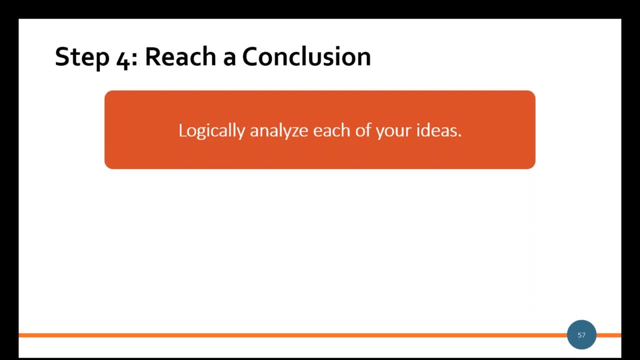 When it comes time to reaching a conclusion, you want to make sure that there's a logical flow between the information you have and the conclusion that you are drawing overall, And you're also kind of discarding those that don't meet your criteria Or may have adverse consequences, because your decision criteria gets at the positive side. 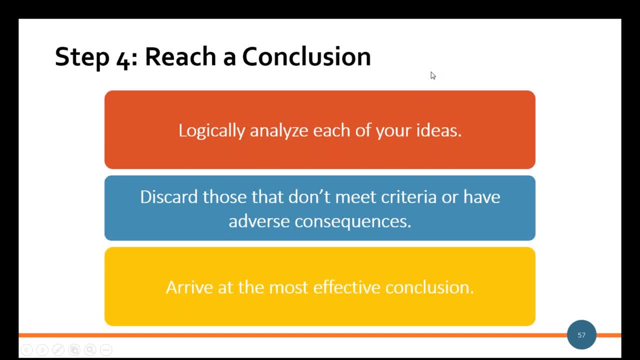 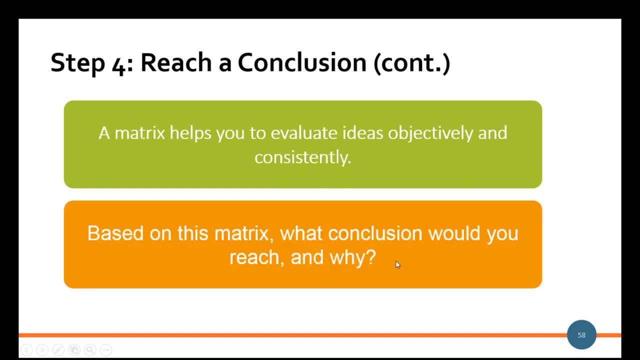 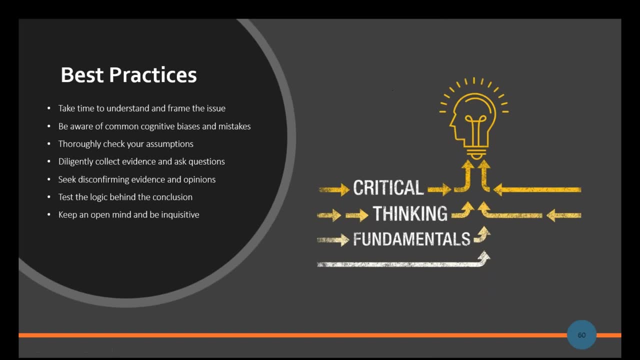 But you also want to do potential problem analysis to look at the potential downside. All right, So let's take a look at kind of some general best practices And then we can open it up for a few questions if you would like. The key here is: take time to understand and frame the issue. 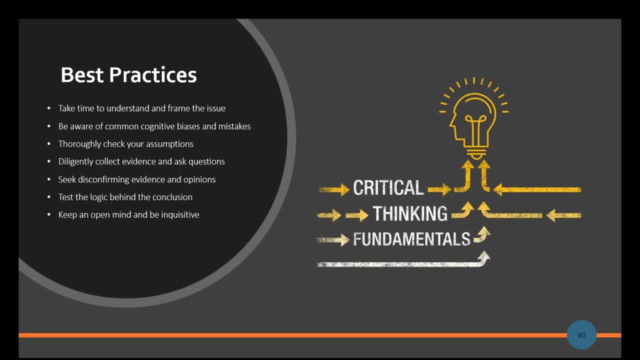 Seed here is not necessarily your friend, Even when you think you know what the situation is or you've seen it before. that, in fact, could be one of the biases. I've seen this before. I know exactly what it is. I'll do what I did before. 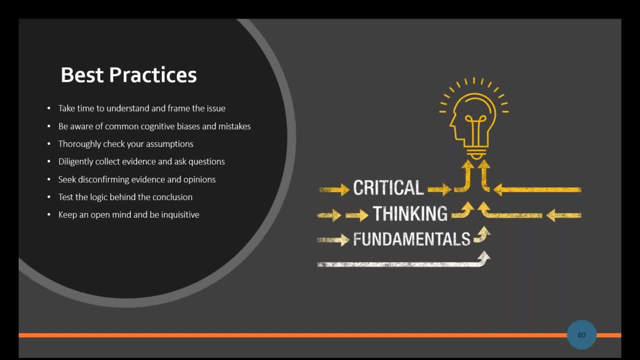 Take time to really understand, Frame the issue, to understand the problem, And then the key here is to be aware Awareness of your biases makes a big difference. It's not that you can eliminate your bias, It's not that you can all of a sudden not have them. 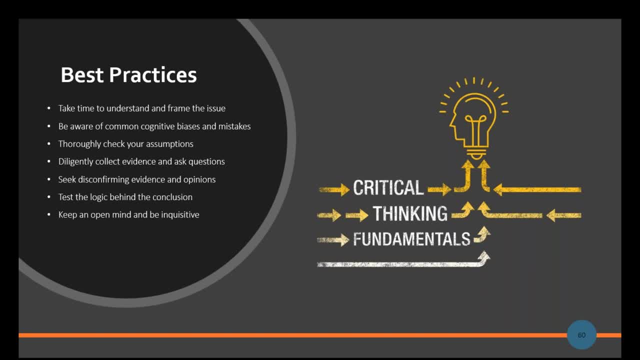 The key is to be aware, Because those biases actually help you sort through the enormous amount of information that you get every day. The idea here is to be aware of the bias and not let it have a negative impact on the way you're looking at the information and the way you're drawing conclusions. 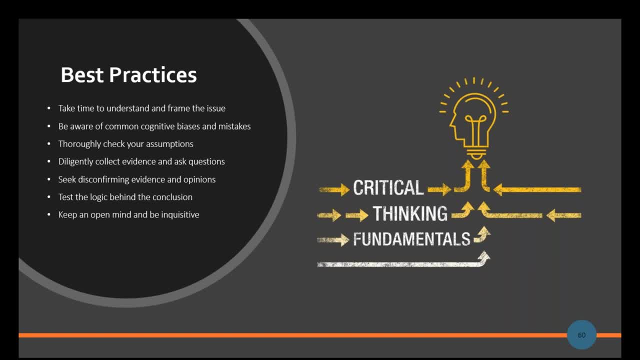 Right Along with that is to check assumptions. Make sure that opinions are backed up with data, Make sure that the facts you're looking at are presented in the most useful and relevant manner, That the information is not being manipulated or that people are selectively disclosing information. 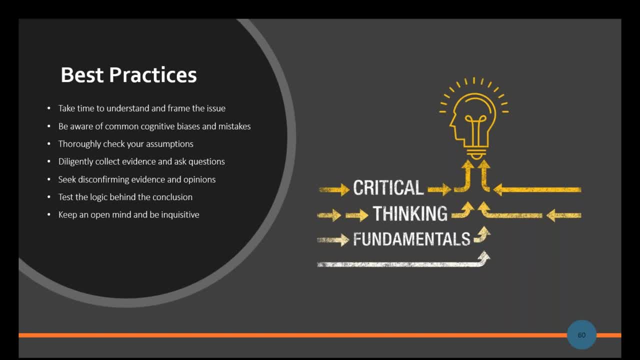 Right, You want to be diligent about collecting data and asking questions. A big part of critical thinking is asking questions overall. Now again, timeframes cause us to not do that, because it extends the decision-making process, But in fact, it's really just investing time on the front end to make a better quality decision, so you spend less time on the back end trying to fix it overall. 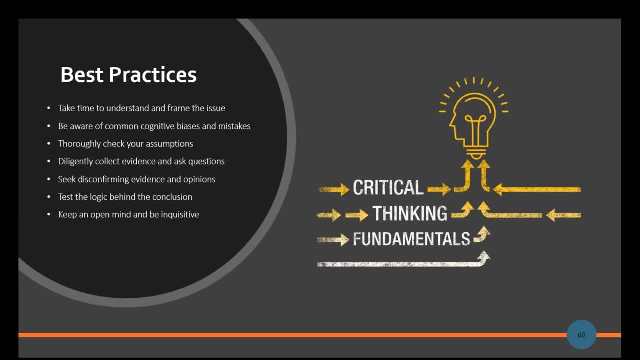 The other thing is that you should work hard to find evidence that refutes your conclusions, Find information that's disconfirming. Many of us work hard to find information that supports our point of view, And I would suggest that that's self-defeating. 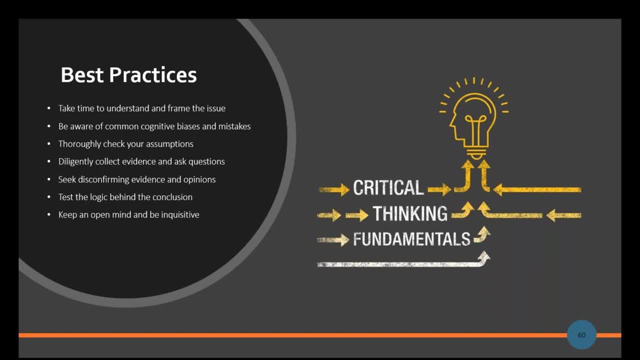 Look for information that is actually the opposite of what you would like to do, that refutes it. If, in fact, you try to knock down your idea and it still holds up, you have much more confidence that it's the right way to go. 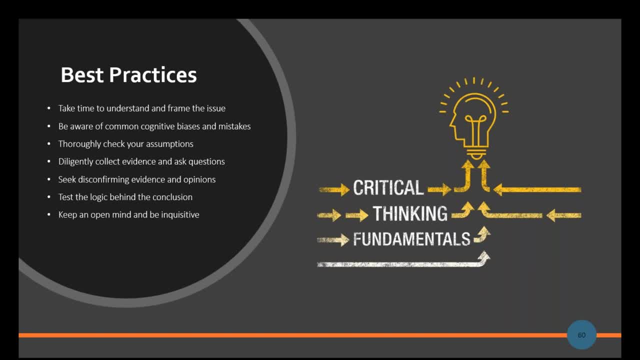 Right. So optimize that. Embrace contradictory information to really make sure your idea holds up overall. Focus on objectively testing the logic of your conclusion. Does it follow from the data that you have? overall, And try to remain open-minded, not too attached to your particular preference or opinion or conclusion. 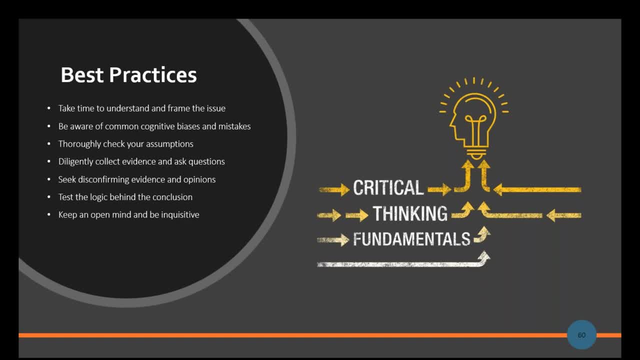 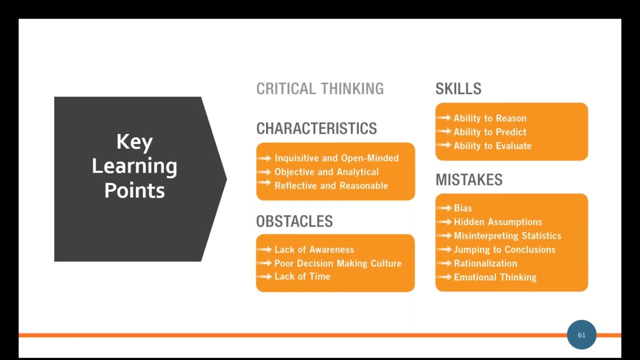 And be open to other points of view, Right. So just in general characteristics of critical thinkers. it's about being inquisitive, being objective, being reflective. These are things, if you're aware, you can in fact make happen overall. 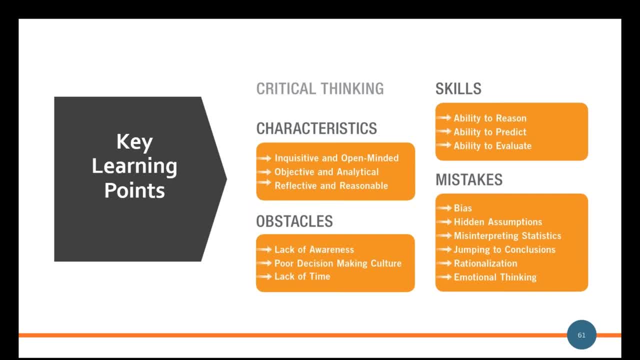 Some of those things, those characteristics, are not always skill-driven. On the skill side, though, it's really about reasoning, being able to anticipate or look forward at potential outcomes, Think forward at potential problems or consequences, and then being able to evaluate information in an objective manner. 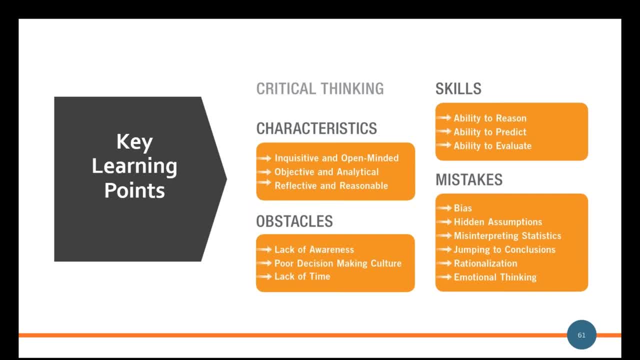 The obstacles we talked about: the lack of awareness, a culture that doesn't support critical thinking, and the lack of time And those things we actually can control to some degree And to avoid some of those mistakes: Right, The cognitive biases, rationalizations. 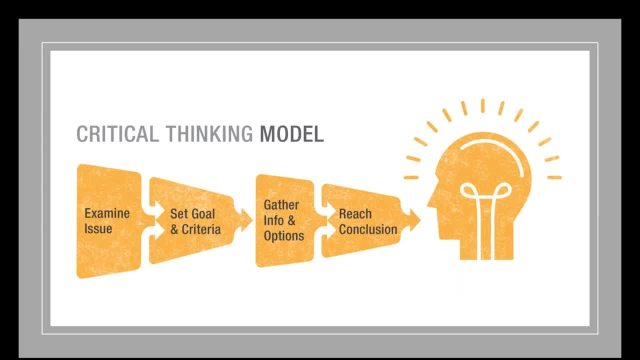 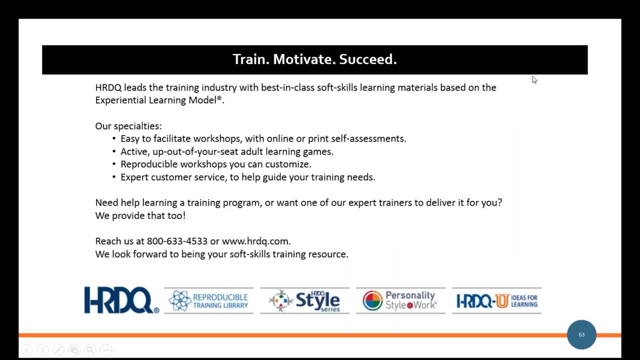 And to let emotional thinking come first. thinking dominate your uh approach. all right, so we have some time for a couple of questions, but i'll turn it over to sarah uh at this point. wonderful, thank you so much, chris. uh, rick, we do have, um, we do have some time for questions, so go ahead and type those up, send those in. 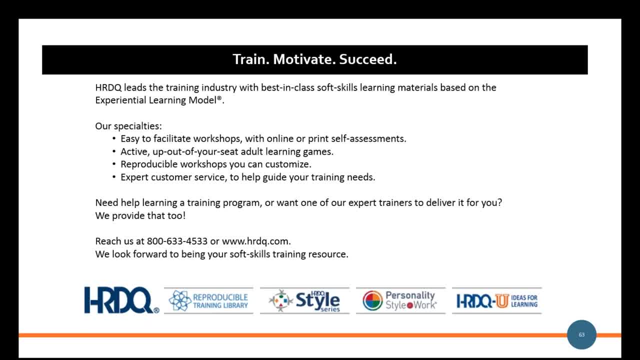 um, while we're waiting for those, i just want to introduce everyone to hrdq. we publish research based experiential learning products that you can deliver in your organization. today's session was based on our critical thinking fundamentals, and that is a piece that you can deliver yourself. 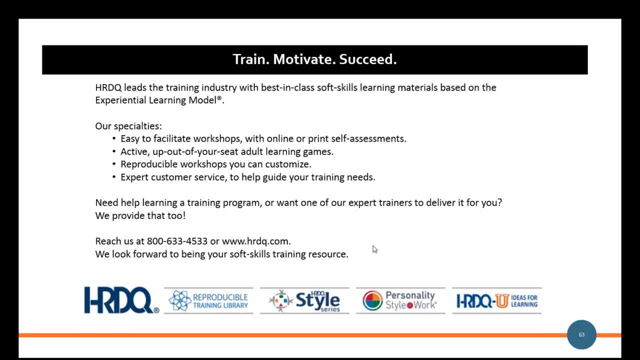 or if you want one of our expert trainers, like rick, to deliver it for for you, we also provide those services. so good, i can see some questions are coming in in, um, so let's go ahead and we're going to get started there. um. so our first question is about: 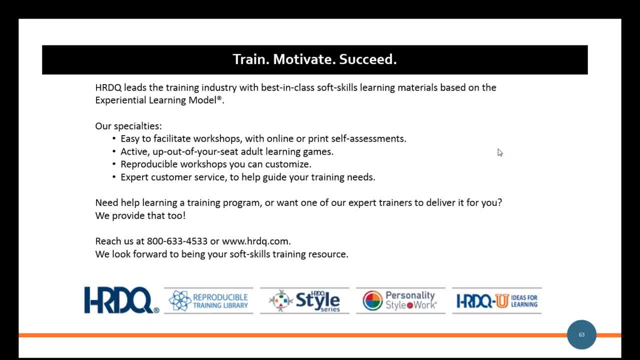 emotion. um, what role do emotions play in critical thinking and decision making? are they always a problem? yeah, no, i don't think. i don't think emotions are always a problem because, again, emotions can be based on sort of your gut reaction, and your, your gut reaction is not necessarily. 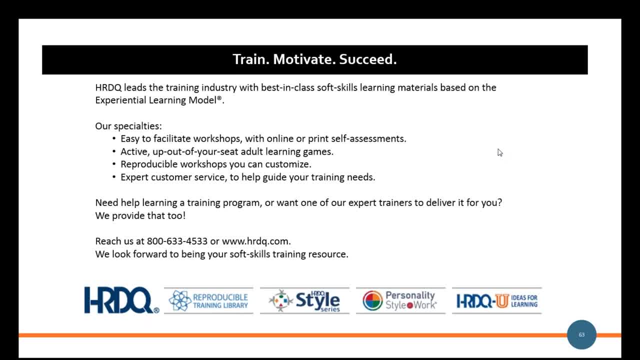 based on nothing. right, it's based on your experience, your previous experience, your knowledge um, which really adds a lot of value. you may not be able to articulate it clearly, but the emotional side isn't always bad. now the emotional side, like anger or stress, can definitely be a problem. so the 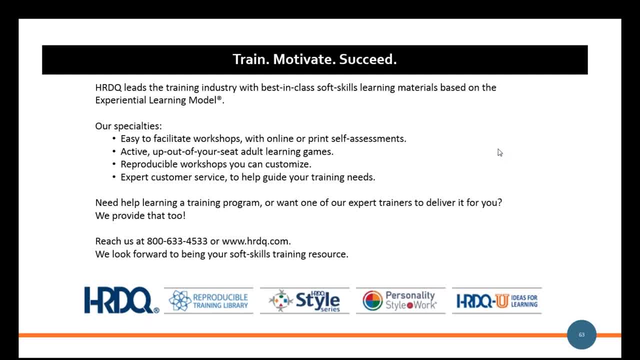 idea there is to sort of, you know, take time. it's sort of like count to ten and give time for your rational brain to kick in. but you really do want to have a balance of both the rational analytic side and sort of the intuitive gut sense on things, because both of them add value. 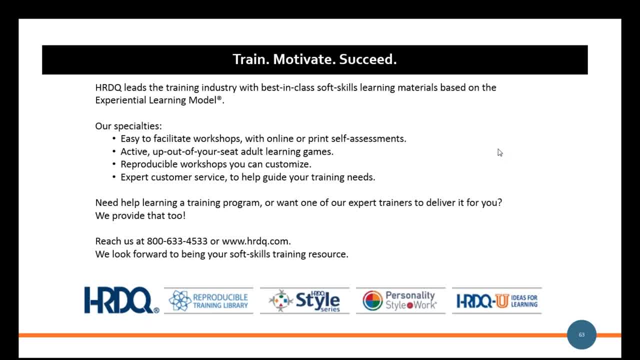 and again, the challenge is to keep them in balance and not let one dominate the other. overall, great thank you. our next question, um, is about the culture of the organization. um, how can you change a poor decision-making culture? yeah, and that could become a little bit more difficult. so 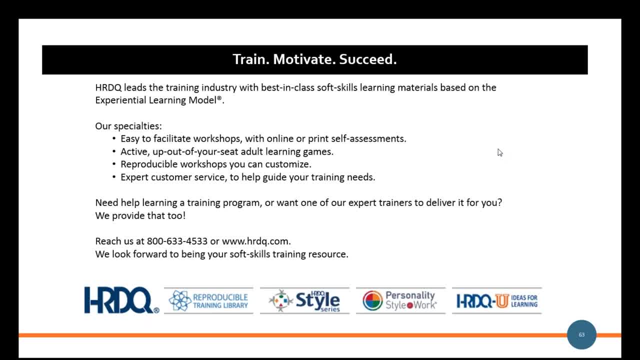 part of it is define culture, and a lot of it depends on where you are in the organization. but, um, culture is really the kind of the aggregate of individual behavior, right, and that's uh, and behavior kind of reflects values and norms overall. so it starts with controlling what you can control, you know, as to the best durability. so for those of you that, 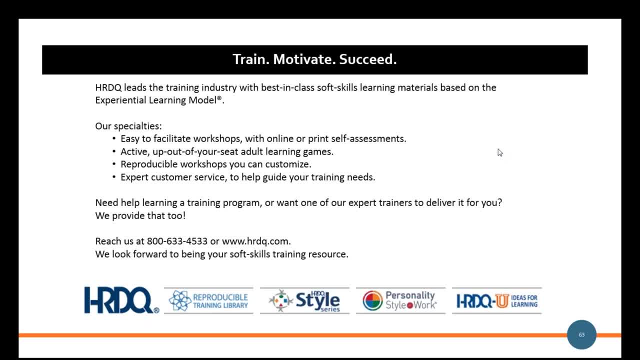 actually lead teams. you actually need to be able to control what you can control- and that's part of it- actually can start to apply some of these critical thinking concepts to your team overall. now again, you may not be able to impact the entire organization, but you can impact the culture. 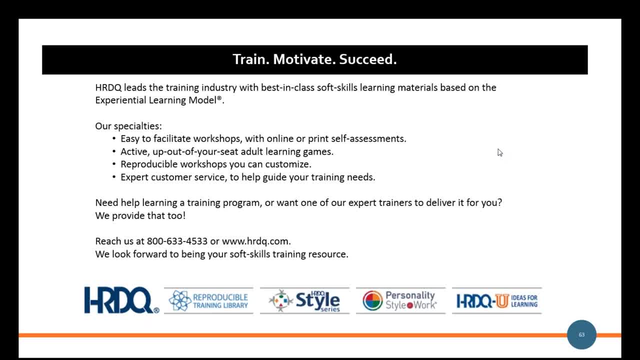 of your team, the culture of your department overall, if you're just an individual contributor where you don't necessarily have authority or control over how the department or function or organization is working. the idea is just to start to model it right to ask some of these key questions, to pose alternatives for people, to do it in a way that's constructive. 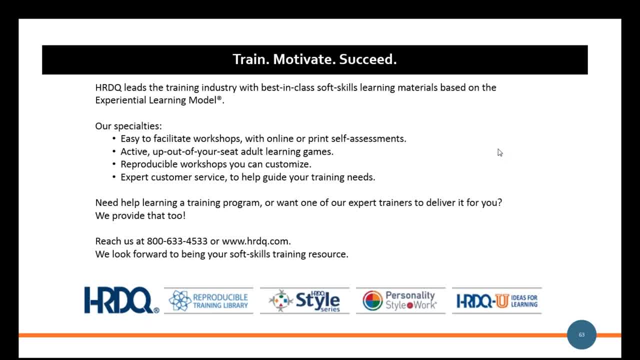 that doesn't necessarily eat up a lot of time, but to help people see the value overall. so there are a number of ways to make it happen, but the more senior you are in the organization, the more you can, the broader, uh kind of span you can impact by the application of some of these. 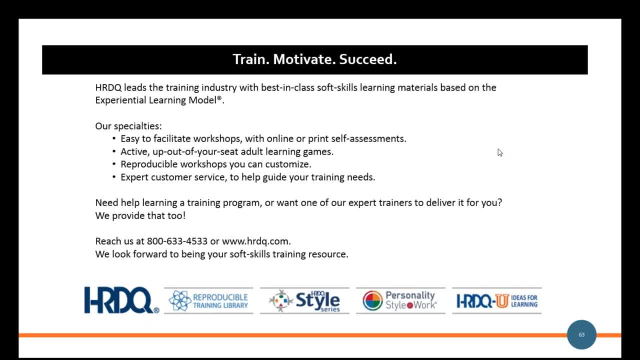 concepts and tools and it's really just setting up expectations to make sure that people are available, that people understand what they are and that you're reinforcing their youth. good and rick, i, i sort of have. i have a question here. um, for you myself, how do i know? 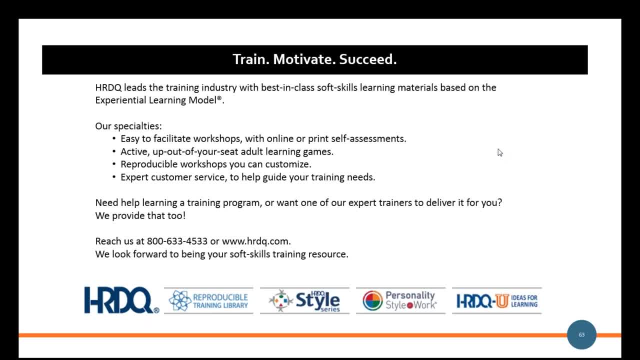 that i that i am a good- you know that i am good at critical thinking: how, how, how would i have a have a sense for that right? well, there's a couple of things one i mean on the. it starts with being self-reflective and really starts with being self-reflective and really starts with being self-reflective. 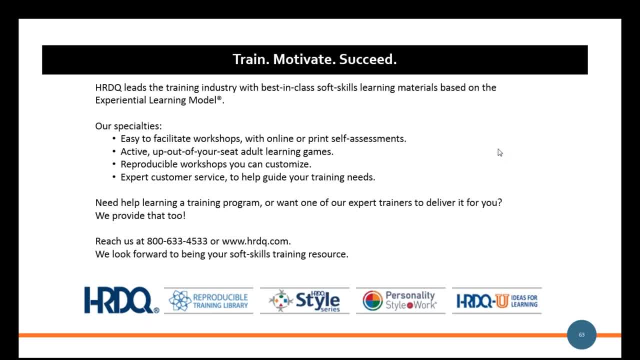 thinking about? are you questioning assumptions? are you using a systematic process? are you evaluating information? you could just sort of do a self checklist. you can also get feedback from others in terms of, you know, debrief the decision making process. you know, take a look at decisions that have been made and say how do we go about that overall and debrief it in the context of 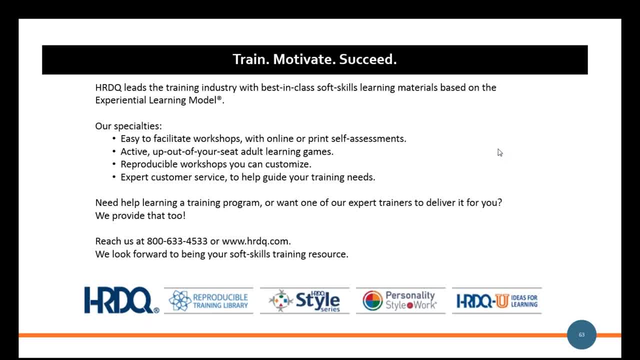 some of the tools we talked about today. but in addition to that, you could also evaluate your uh thinking using different um self-assessments. there's two of them that are out there. one of it is the watson glazer critical thinking test and the other is the hogan business reasoning inventory. 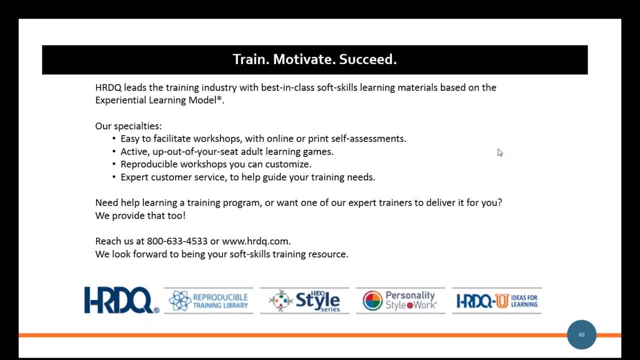 both of them will give you some insight into your ability to think critically. they give you a whole range of scenarios and they ask you to draw conclusions based on the scenarios that you're looking at. so those are two self-assessments that are available, uh, in the public domain, that you'd 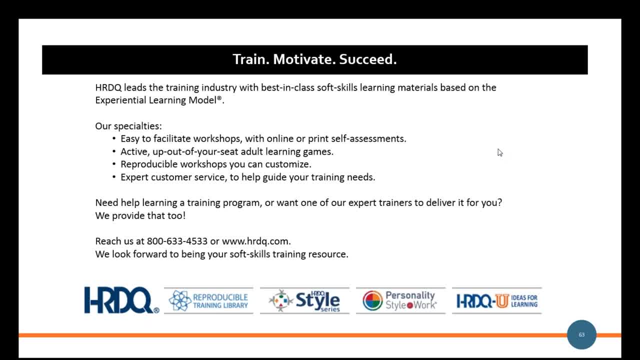 be able to use based on the scenarios that you're looking at. so those are two self-assessments that are available, uh, in the public domain that you'd be able to. So get some read on your critical thinking skills. Good, Great. And our last question- here I think that we're going to have time for- is around hiring. 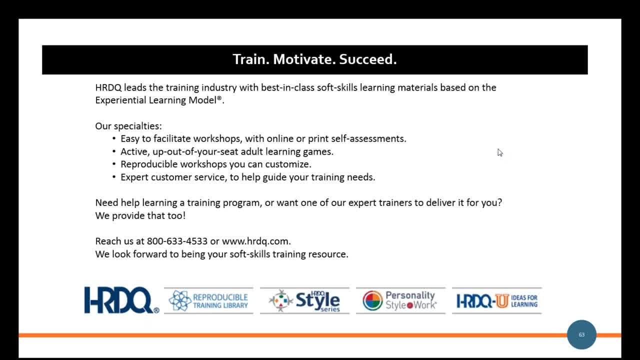 Can you talk a little bit about critical thinking in relation to bias and emotions in when you're making hiring decisions? Yeah right, That's actually a good question, because that's one of the places where where it plays out a great deal. So what one has to do with the time we put in to really look at the candidate overall and the kinds of questions we're asking in the in the hiring process. 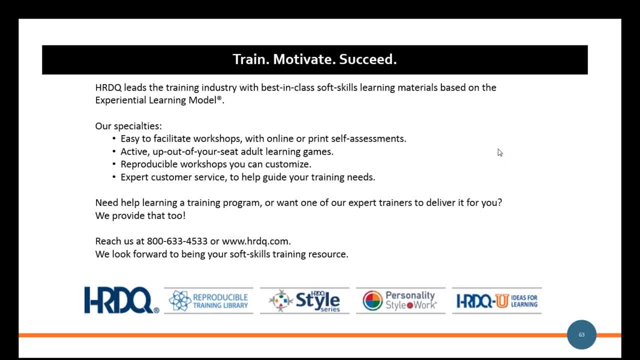 Frequently. frequently we ask sort of softball questions, easy questions, We don't really challenge people and we may not even have a competency. The competency model would be your decision criteria and to say: how well does this person line up against these competencies that I'm using to make the hiring decision. 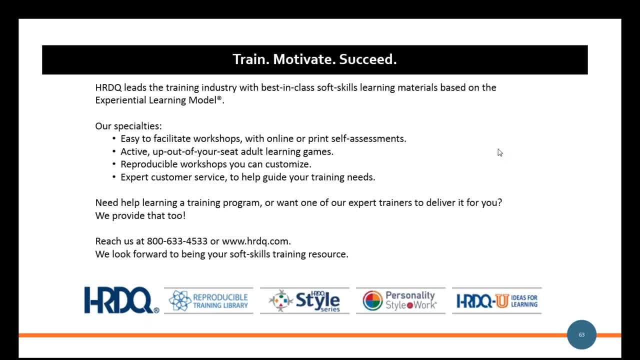 So that's one starting point. Do you have the competencies that you're looking for And are you asking questions to better get at whether they have the competency or not? The other is around biases. You know, if somebody walks in and we just like them right, they go to the same school. 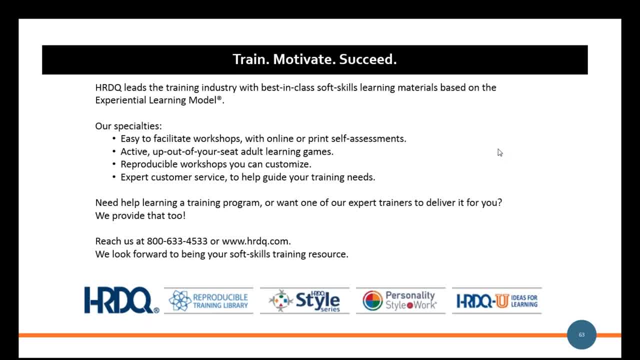 We went To. we just look for data that supports why we should hire them Right. So you're trying to avoid that kind of a bias, you know that confirmation kind of a bias, or the rationalization bias overall, or we're just not really we don't care. 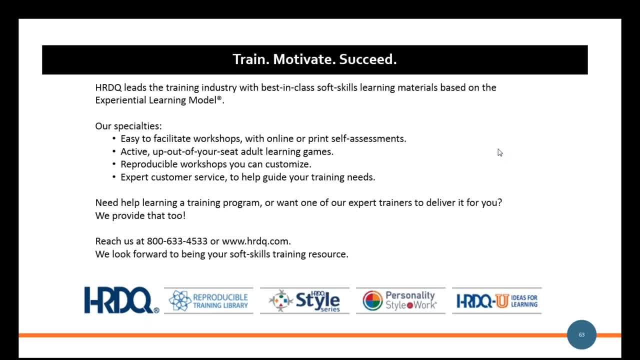 We've got to fill the spot. We'll take the first warm body that looks like they can answer my questions and seem reasonably personable. We'll just like get them into the seat right away, Right, And the problem With that is that you end up getting into a cycle of having to continually rehire because you make a bad hiring choice. 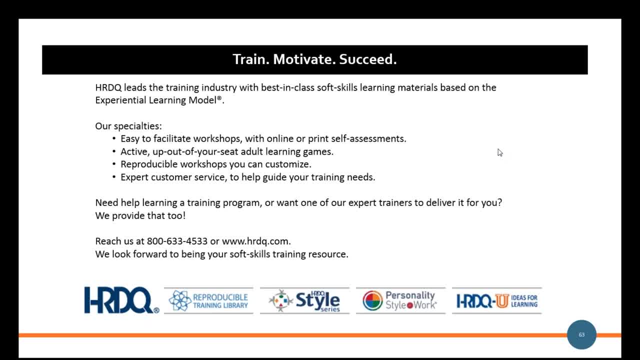 The person doesn't work out And rather than the speed there works against you, because rather than finding somebody who will stay with the organization and perform at a high level, we find someone who really is not a good fit, They turn over and then we're back into the hiring cycle again. 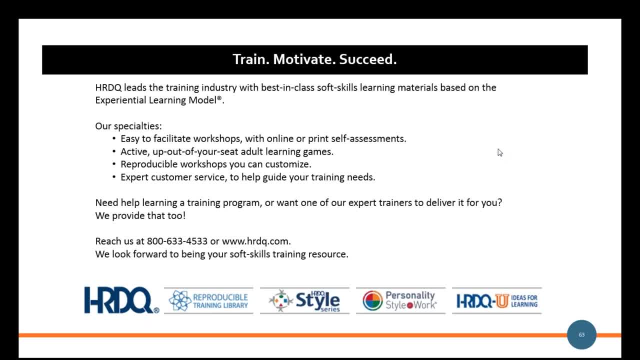 So here, taking the time, using Competency model as your decision criteria, you might even think about using objective testing, because in an interview, people know how to answer your questions and give good interview. But if you use leadership style questionnaires and assessments, they tend to be more objective and you get a better read on people's preferences, their inclination and their style and the extent to which they're a good fit. 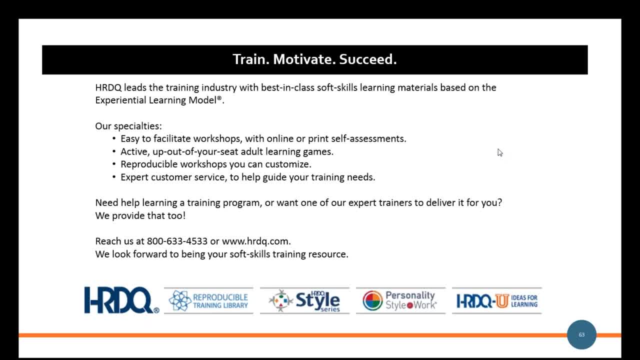 Not just the way they've been coached to answer a question in the interview overall. Thank you so much, Rick. It's it's always wonderful to hear your expertise. Okay, thanks very much. I'm glad we were able to do this and, again, everyone. 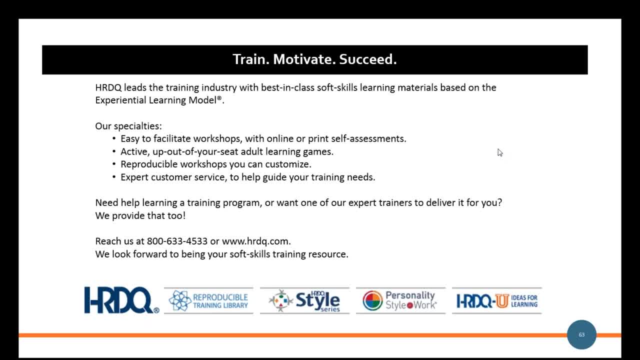 Thank you very much for joining us again. This idea of critical thinking, you know, it's not that there's more fake news in the world, It's just that there's less critical thinking. So The idea is we really do need to be more skeptical, more critical, more objective, to probe a little bit, be more open-minded when you're hearing different points of view. 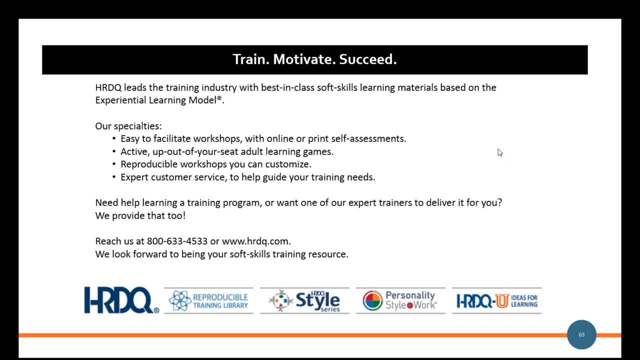 And I think all of that's really about enhancing judgment and the quality of your decision. So thanks very much for joining us today. Good, And if we did not get a chance to answer your question, we will email you shortly with that answer. 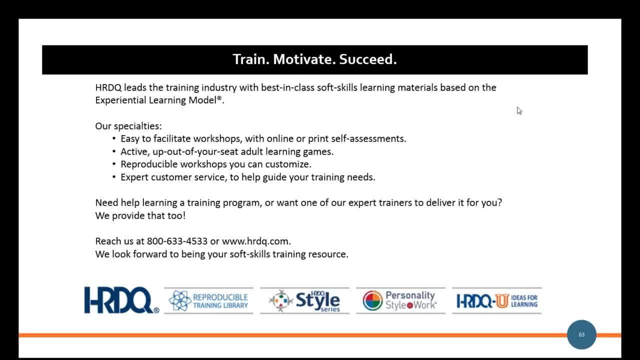 So go ahead. if you have any additional questions, go ahead and type those in. We'll stay on the line here for a second so I can capture those, And we look forward to having you participate in our next webinar.